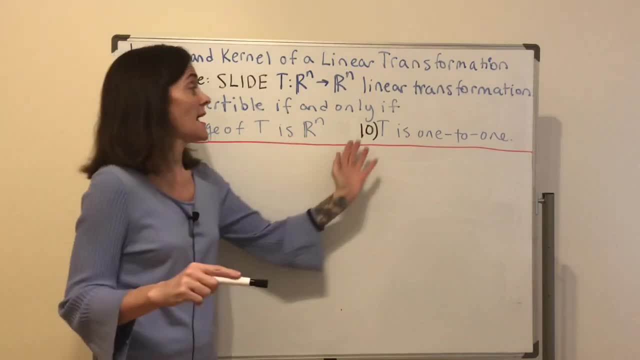 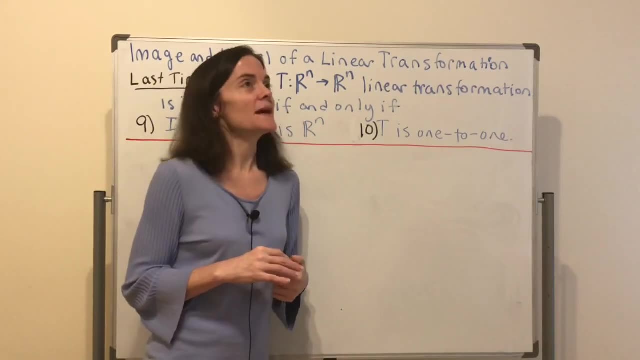 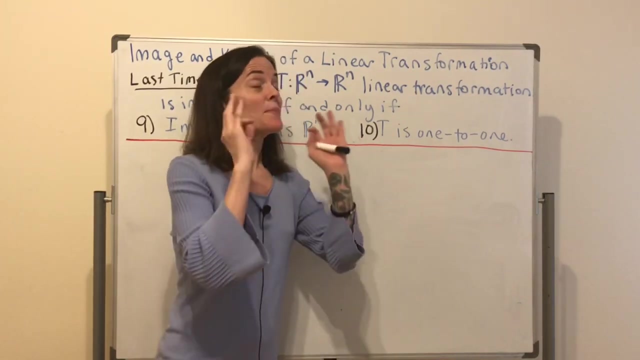 that the image of T is Rn and number 10, that T is one to one, And those are concepts that I touched on during the lesson a little bit, but I didn't really go into detail during the discussion. But now we are going to pursue these ideas, or I should say explore. 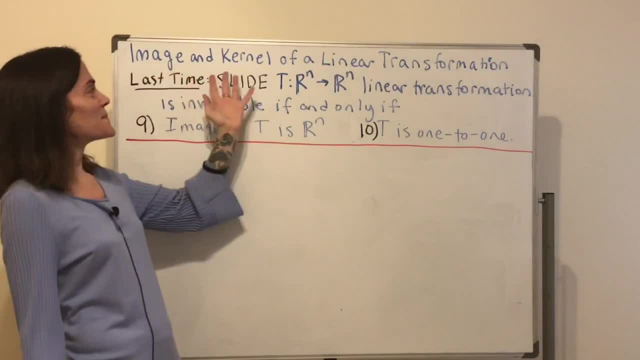 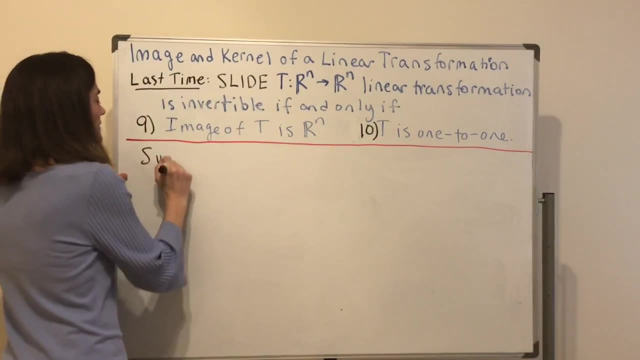 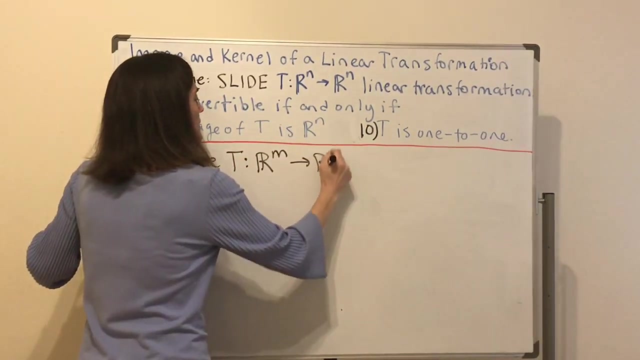 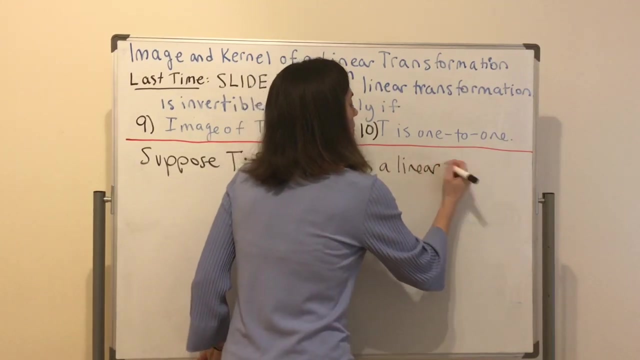 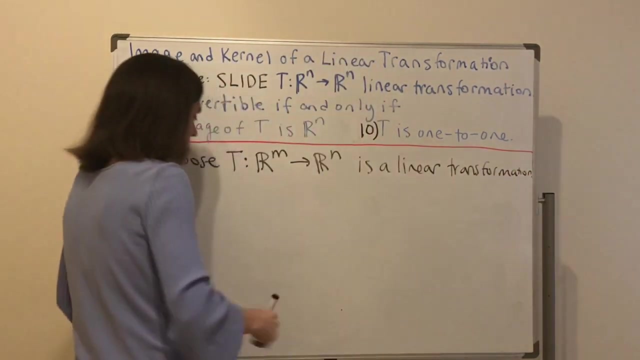 these ideas further as we discuss image and kernel of a linear transformation. So let's begin with Rn And suppose that T from Rm to Rn is a linear transformation. Okay, And what I'd like to define is the image. Well, technically I define the image when we 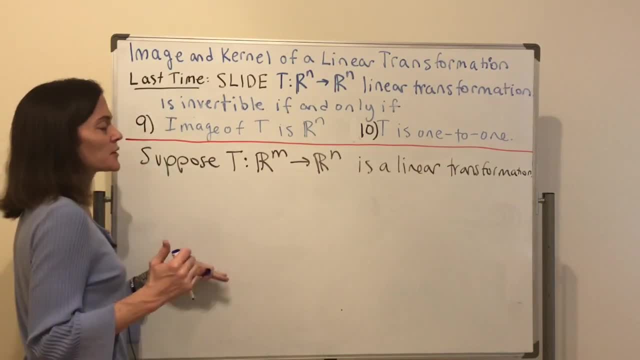 first say Rn, So let's say that T from Rm to Rn is a linear transformation. Okay, And what? I'd started talking about functions, but I will define the image and the kernel right now, and then we're exploring both of them, how to calculate them, things like this, This: 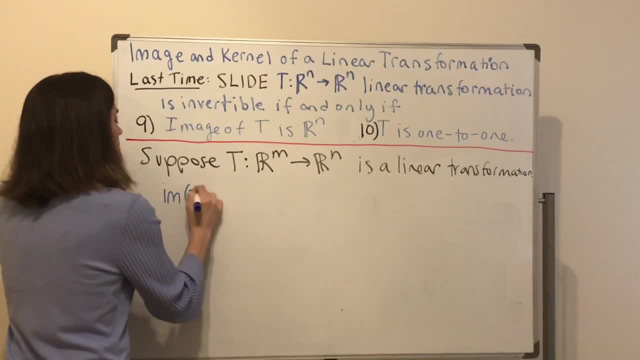 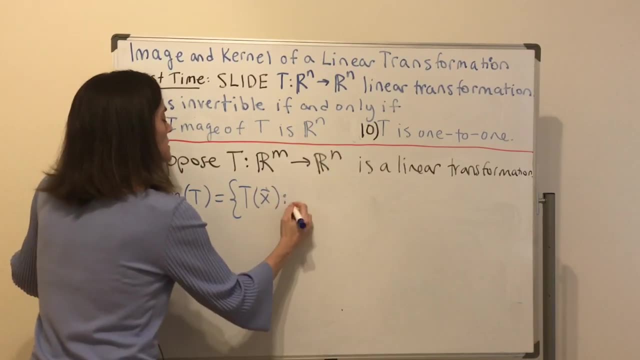 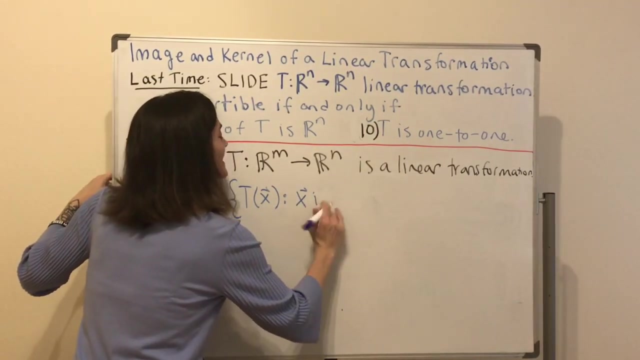 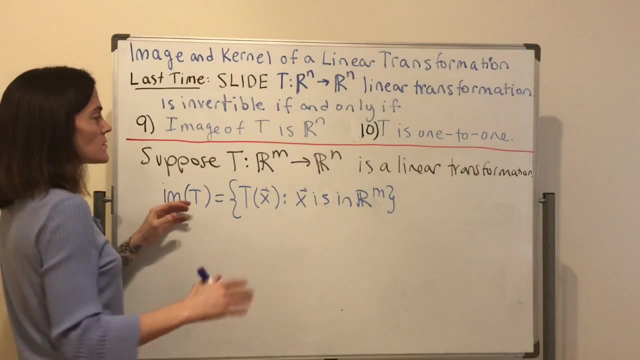 is the topic of today: The image of t. this is a set, It's all t- of x, such that x is n, is n, r, m, And you notice just by. so this is elements in the codomain right. These 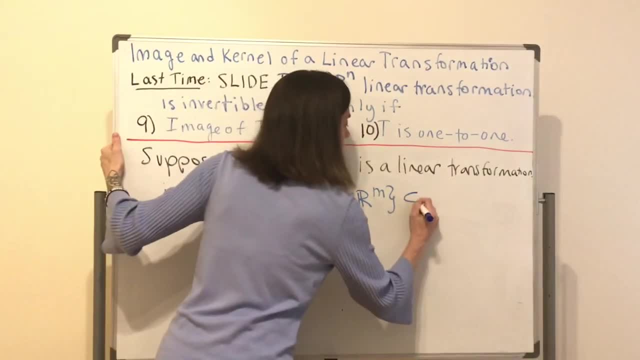 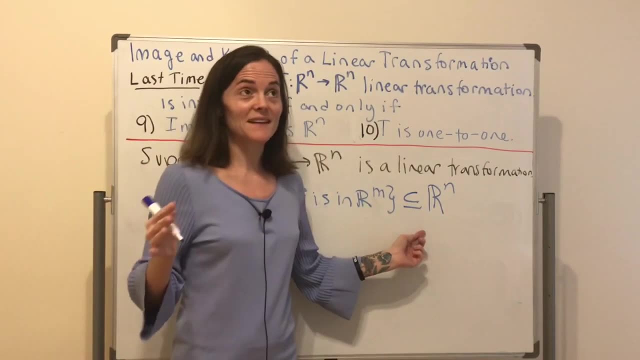 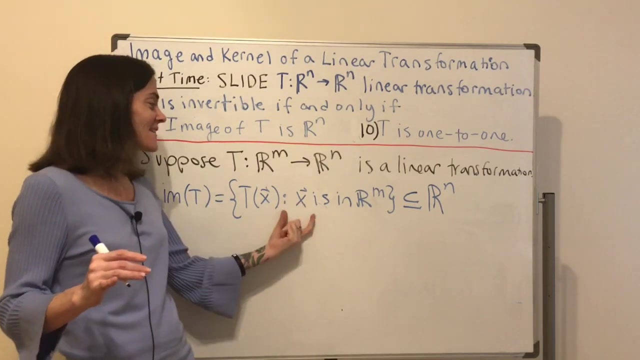 are t of x's. So this is a subset of r, m And this symbol I think most of you have seen. if you haven't, I'll tell you now what it means is said that this is every element here, so every t of x is inside of this set. Okay, so this 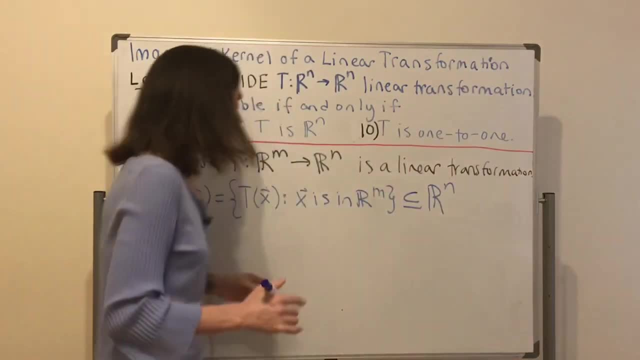 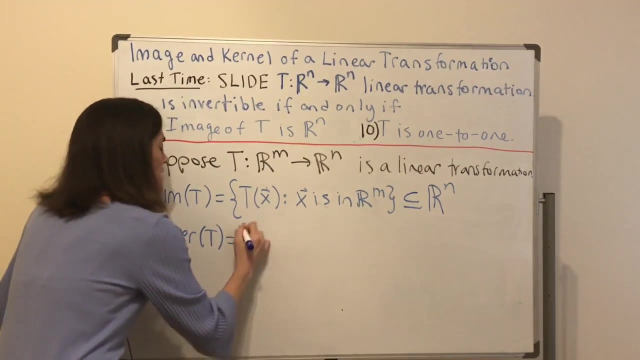 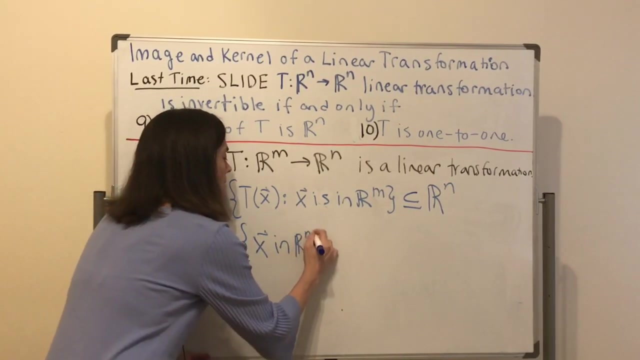 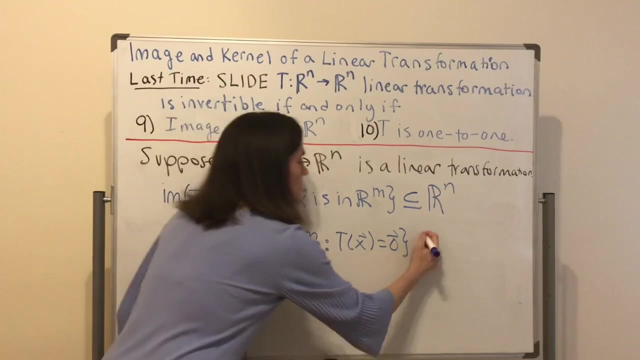 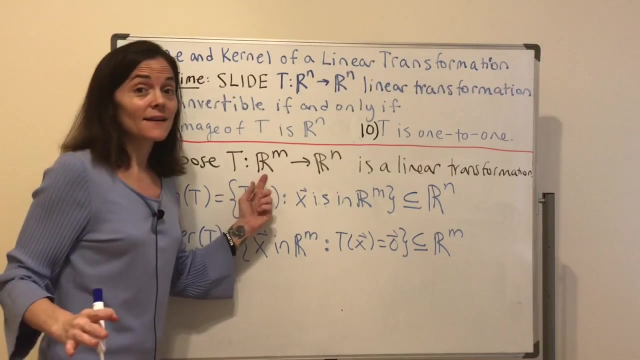 set the image is a subset of our n. Okay, now what's the other topic of today? Kernel, the kernel of a linear transformation. This is the set of all x in our m, such that t of x equals zero, and this is a subset of our m. Okay, so this is everything here in the 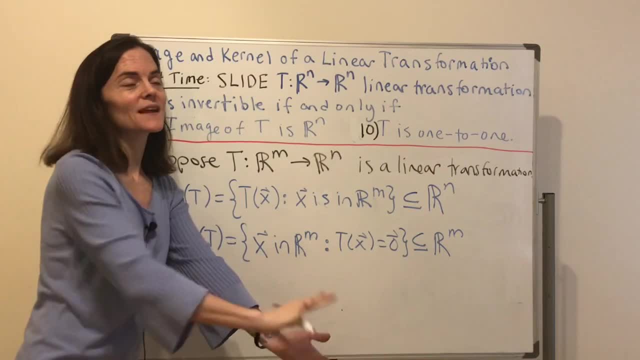 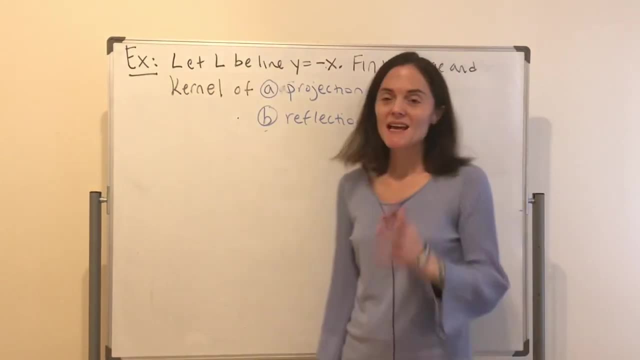 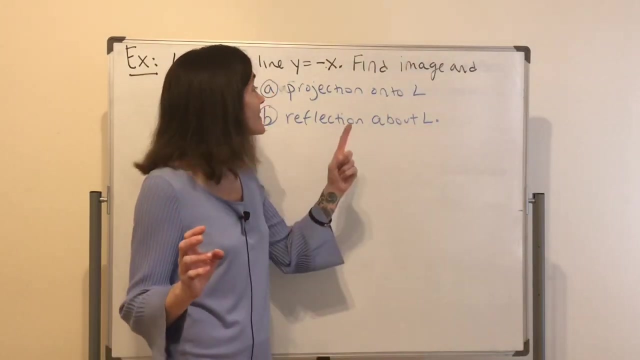 domain that maps to zero, and it is linear transformation. This is the kernel. Let's do an example from geometry first, okay, and I'm going to think about the kernel and the image from the geometry viewpoint, but then I'll also write down the matrices. 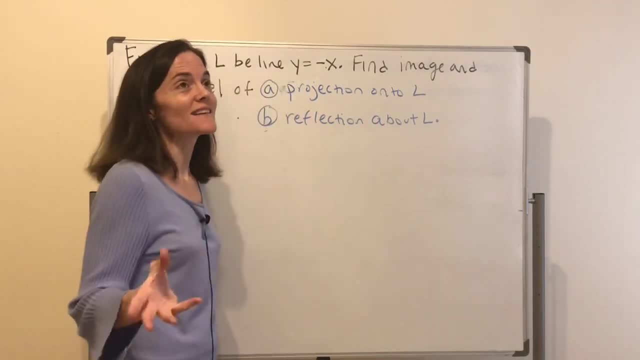 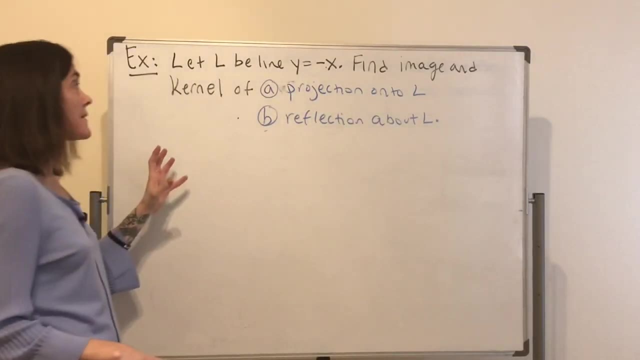 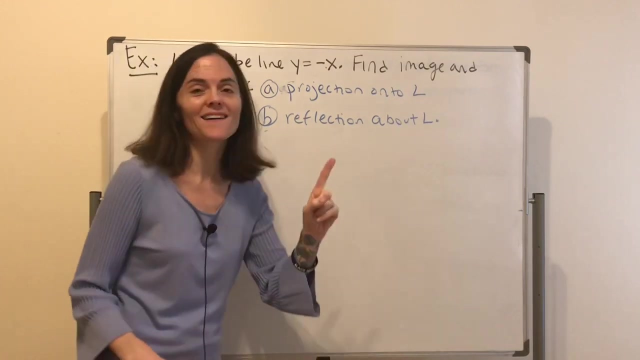 as a nice review, but also to start to connect kernel and image to the matrices, which is a big goal of today. So here l is the line, y is minus x. Let's find the image and kernel of two things: the projection onto l and then the reflection about l. Let's start by drawing a. 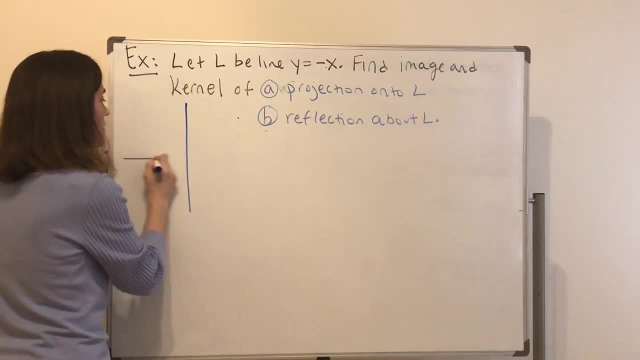 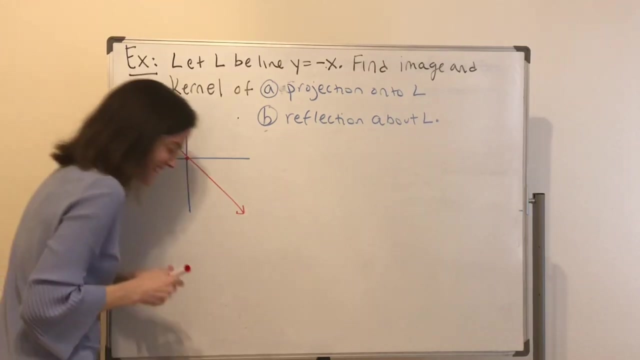 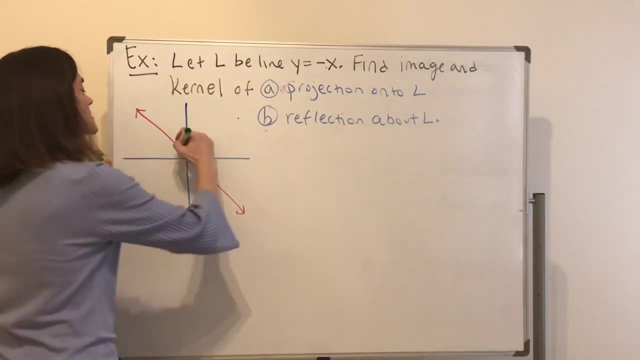 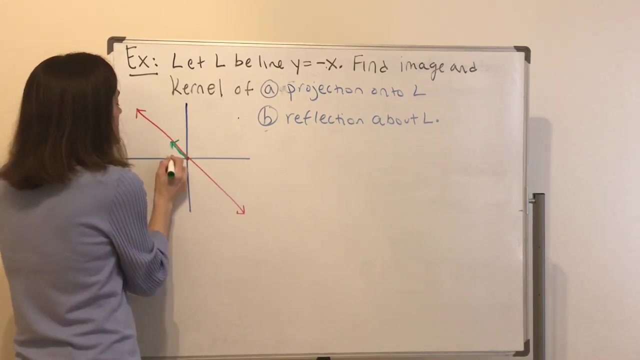 picture here. What does l look like? Well, it's just y is minus x, something like this. okay, and then what do I need in order to think about projection reflection? Well, once I get to the matrices- really, which I will- I need a non-zero vector along the line I can take. 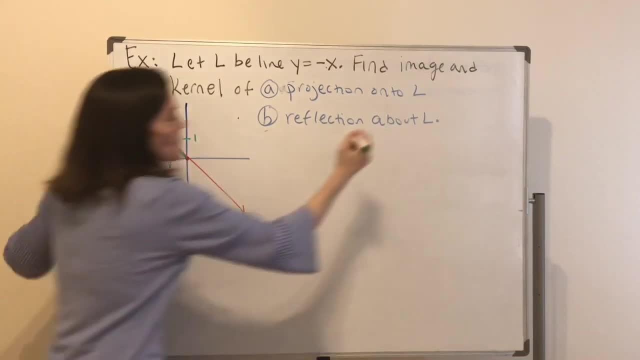 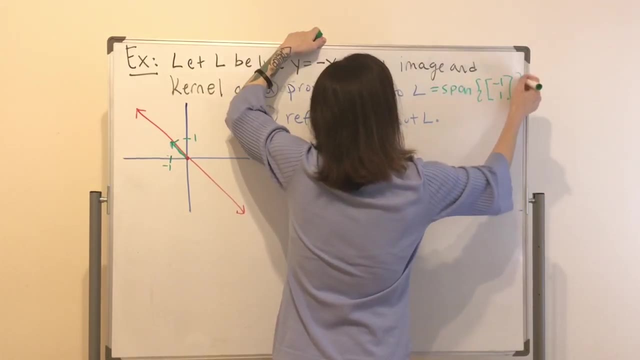 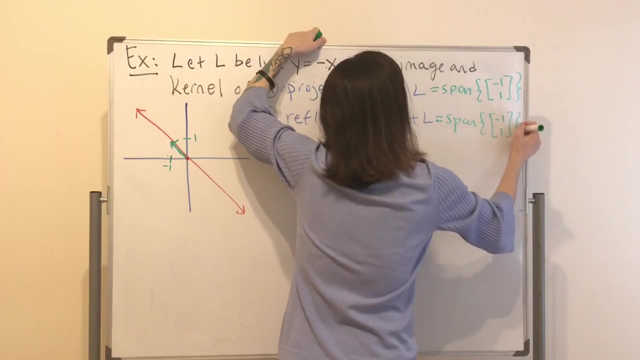 for instance minus 1, 1, so I will take l as the span minus 1, 1, and similarly here This vector is not unit, for example, but that's fine, You just need some non-zero vector along the. 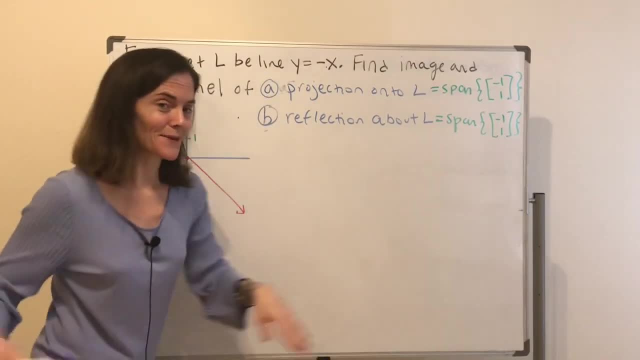 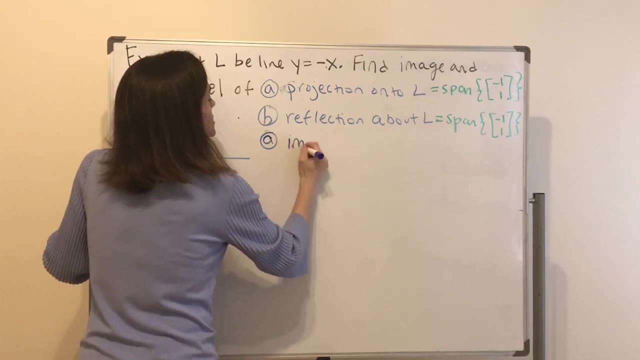 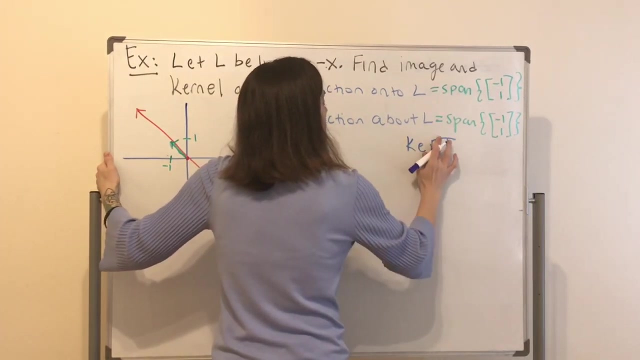 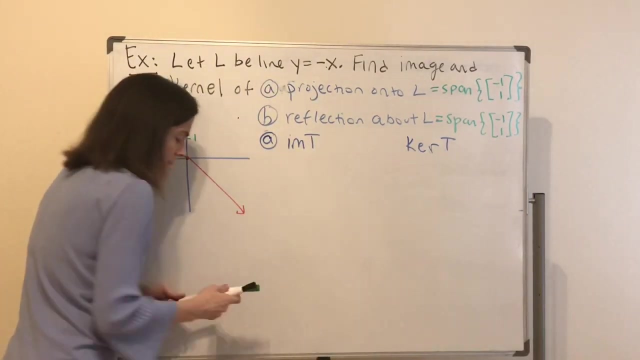 line. Okay, before I write down any matrices, we're going to think about this problem. So, part a: We want the image of t and we want the kernel of t. Okay, well, what happens when you project on a line? We know this is something we spent some time on a few sections ago. no matter what, 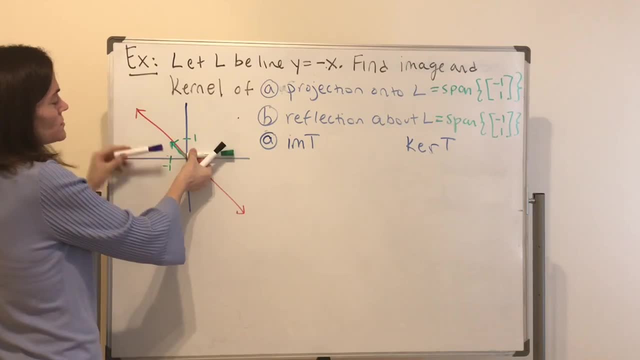 the vector is. okay, there's two vectors, right, They're projected to the line. So it's very clear that the image of t is the kernel of t and we want the kernel of t, okay. Well, what happens when you? 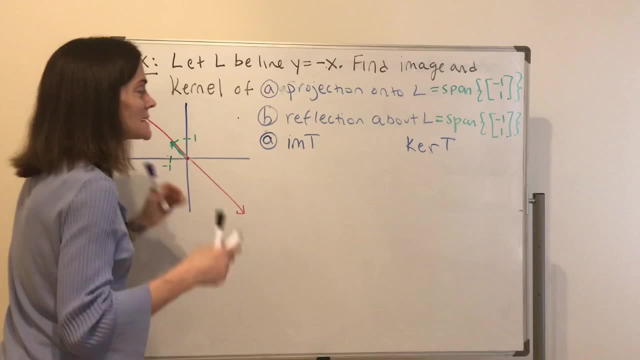 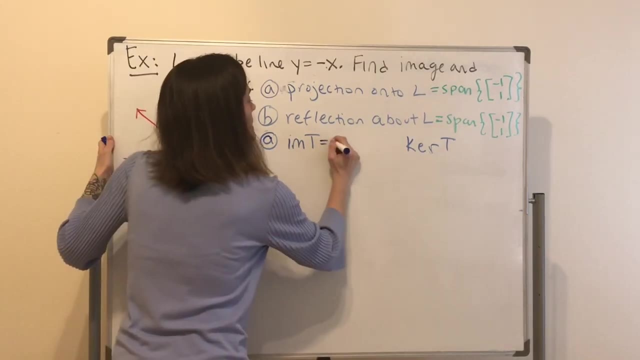 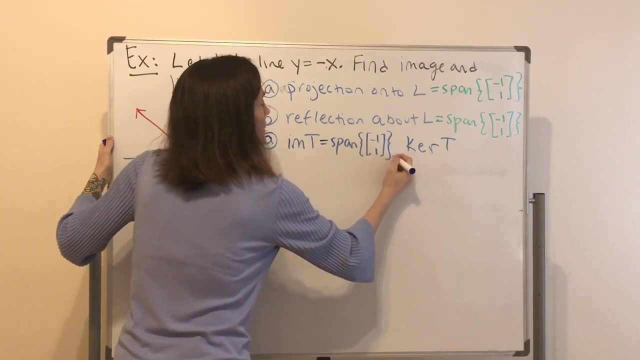 take the image, And we saw this in Maple. The image is the line: Okay, so the image of t. in this case, I'll write it as a span. This is the span of: well, this vector. Okay, what about the kernel? 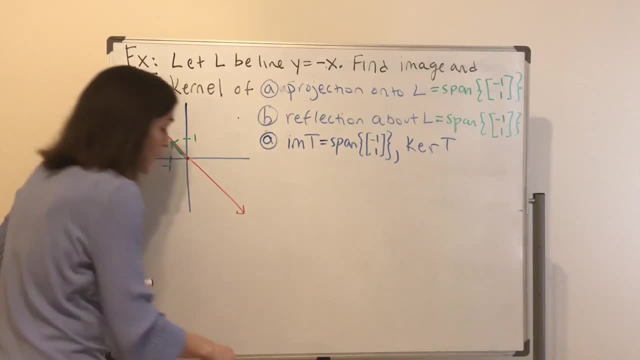 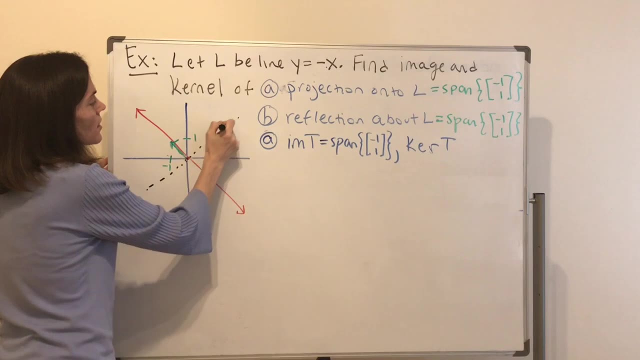 of this transformation, What maps to zero? Well, if I take anything along the line, I'm going to take anything along this line, this line, so I can take a little vector here that meets w perpendicular. Then, if I project anything along this line or any multiple of this which I've 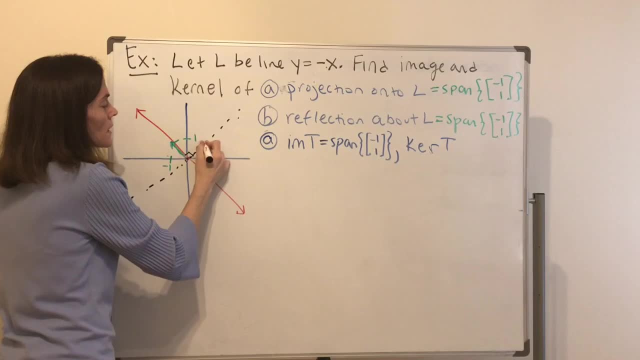 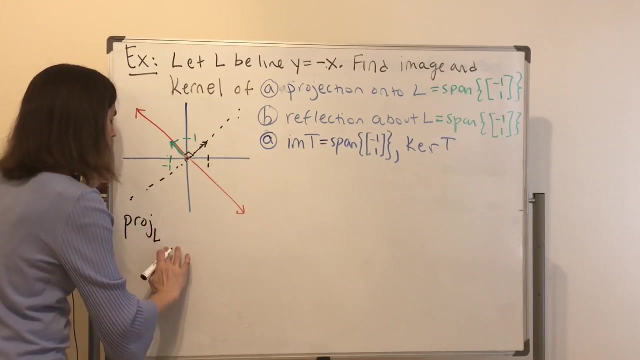 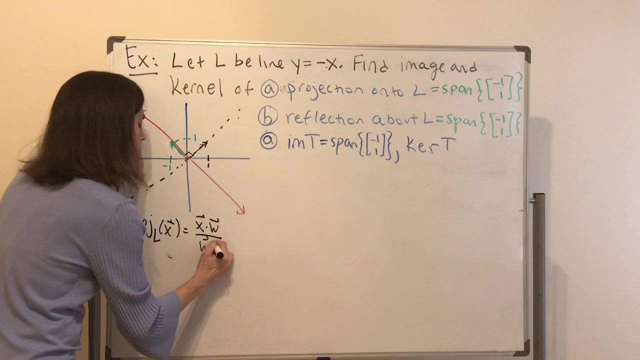 drawn it to be, or try to draw it to be, one one it's going to project or map to zero. Another way to see that maybe I'll write it over here: The formula: if you project on this line of oops of an x, we get xw over ww times w And the only 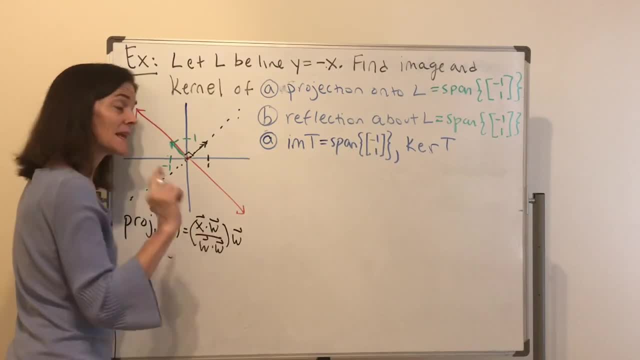 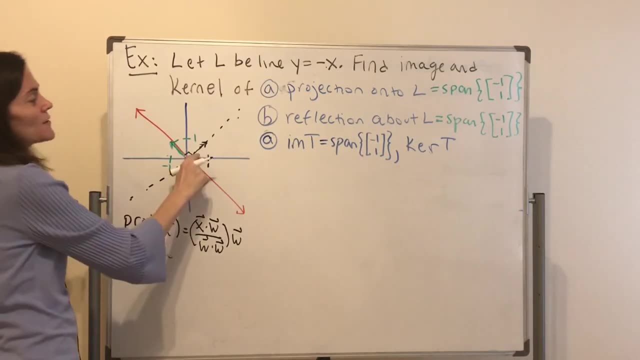 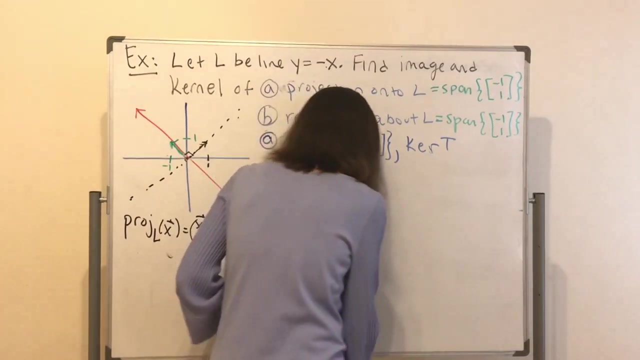 time you see this will be zero is when xw is zero, namely that x is perpendicular to w And here is one vector perpendicular to w and only one vector perpendicular to w, And here is one vector perpendicular to w And all multiples of it are 2.. So we can write the kernel as the span of: 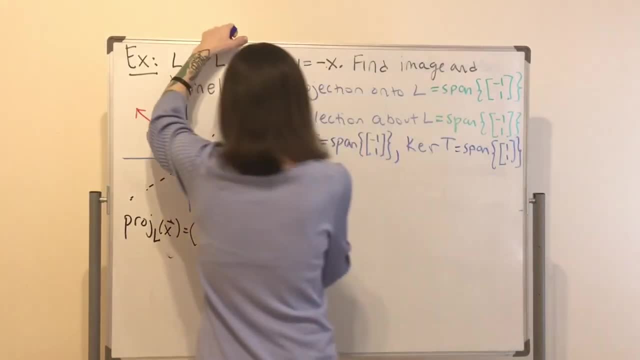 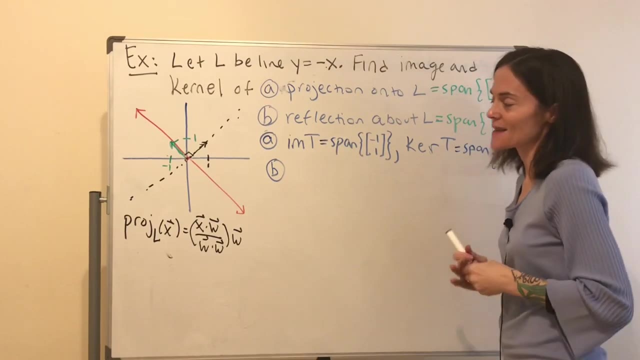 one one, Okay. So part A is done, although I will, as a nice review and also to connect these to matrices, in our very first example, I'll write the matrices after we finish B. Okay, what about reflection? Well, now, this black line is not as, so This is my reflection qualities. to B. Okay, what about the reflection? Well, now, this black line is not as, so This is my reflection. This is my reflection. Okay, so now this black line is not as, so This is my reflection. Well, now, this black. 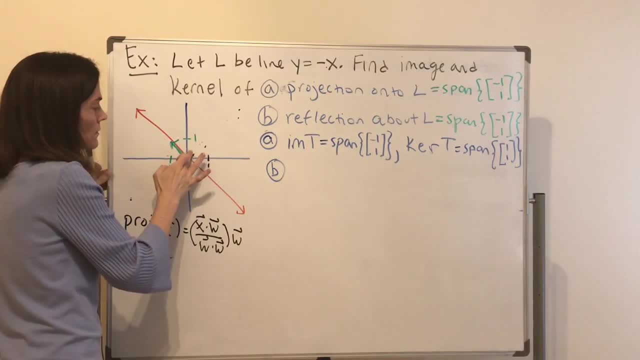 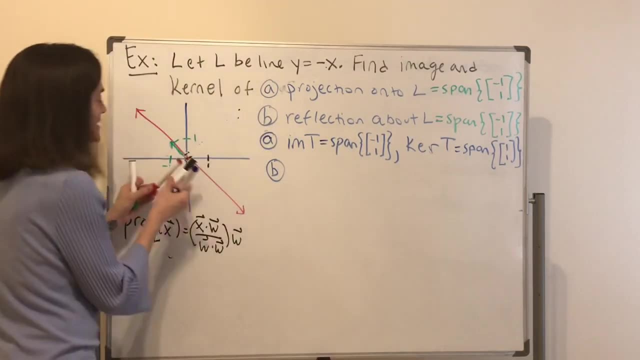 line is not as. so This is my reflection. Okay, and then I'll apply this one. Okay, what about? as meaningful to me Reflection, Here are four vectors in R2.. I don't know where to put them. I can't handle four. 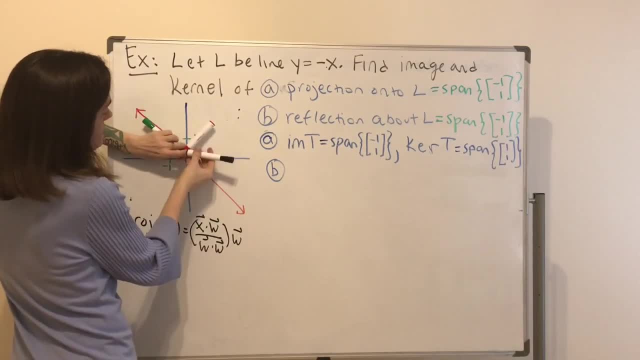 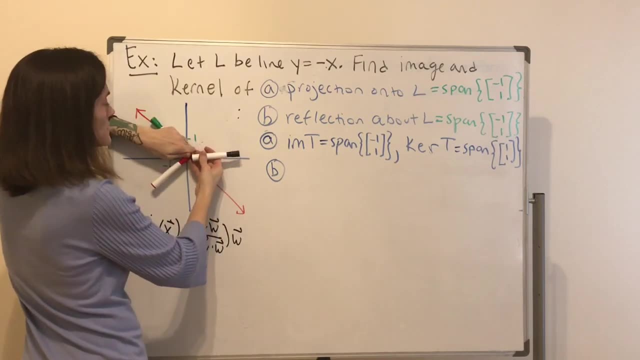 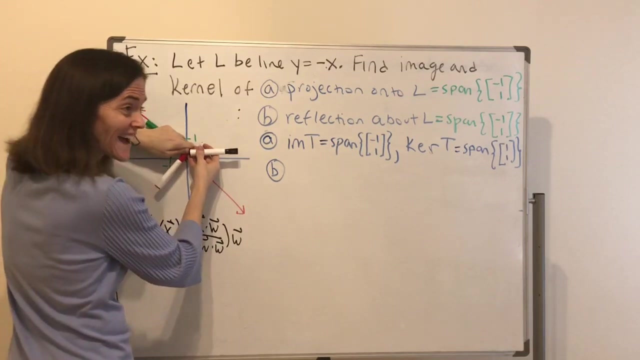 Let's do three vectors in R2.. Okay, here's three vectors in R2.. What happens when you reflect: Uh-oh, this one comes here like this Right Now. did any of those three map to zero? No, they did not. 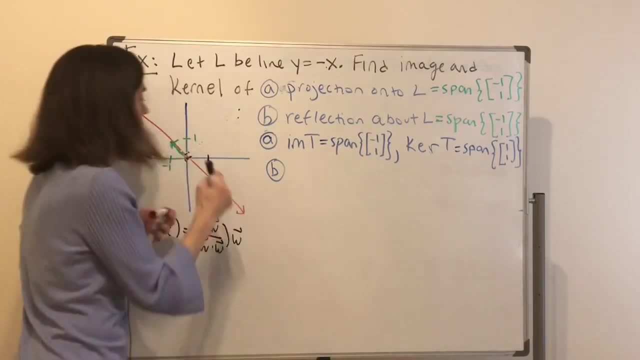 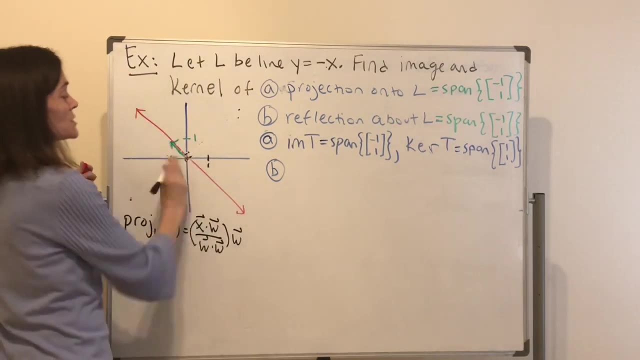 Could you have any vector map to zero? Well, sure, zero maps to zero. That happens with every linear transformation. But anything else, okay. imagine some non-zero vector: It's gonna reflect, okay, Even if you're here on the line. 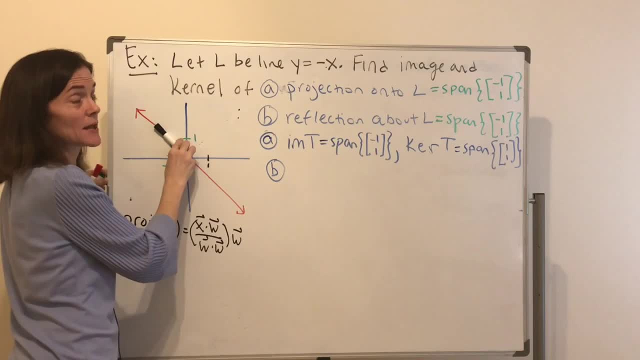 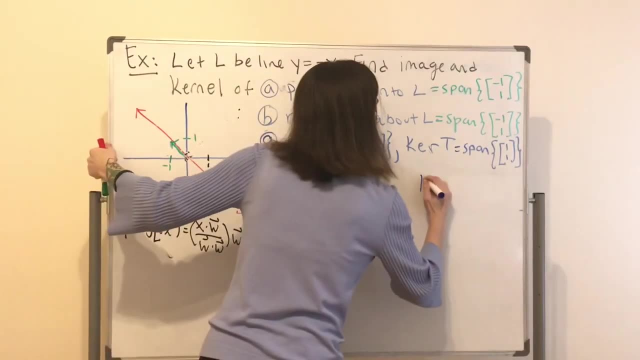 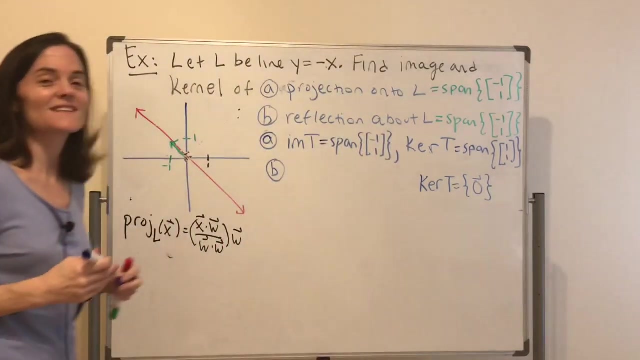 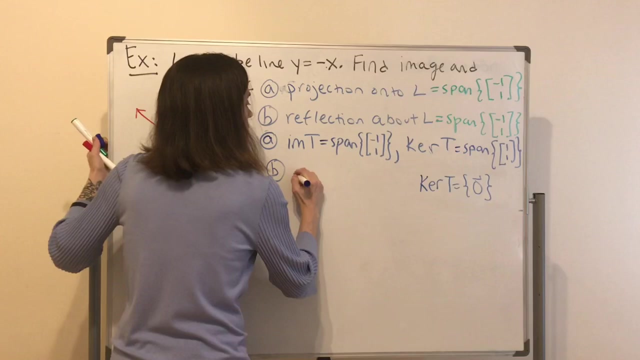 what happens when you reflect? You stay right here, but you do not map to zero. So here, the kernel of this reflection is zero, Just the zero vector And it's image. Well, here's what I'll claim, and then maybe I will try to justify it. 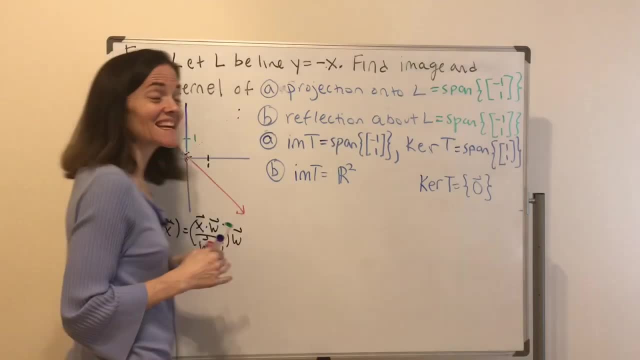 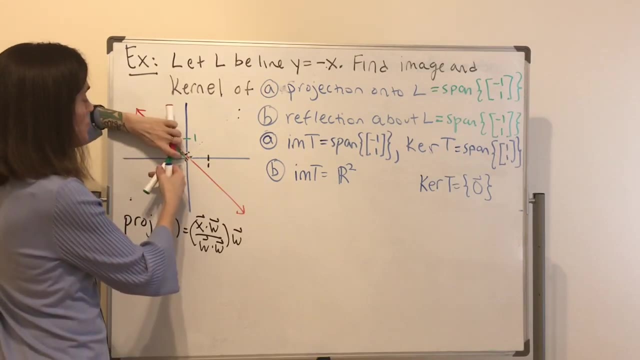 This is all of R2.. How can we see this? Well, one really neat thing about reflection. what happens when you do reflect? You do reflection twice. Now I'm just gonna work with one, Yeah one, You do it twice. 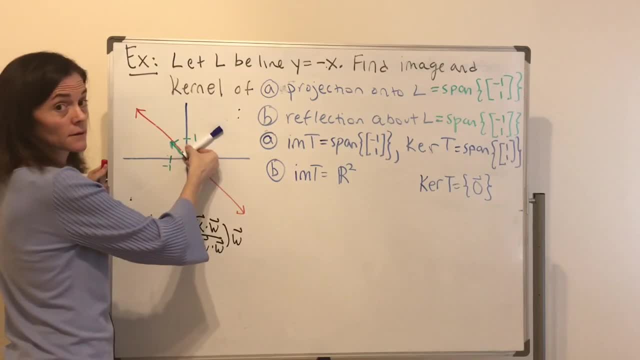 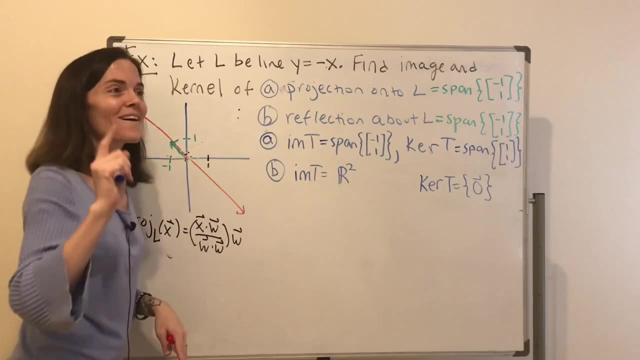 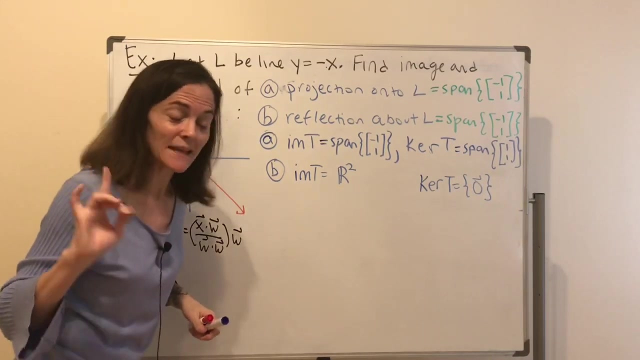 So, one time reflect, Do it again. reflect. Reflection is something that satisfies. if you do it two times, you get the identity map. Or, as we thought about last time, this map is its own inverse. Okay, I hope you followed that. 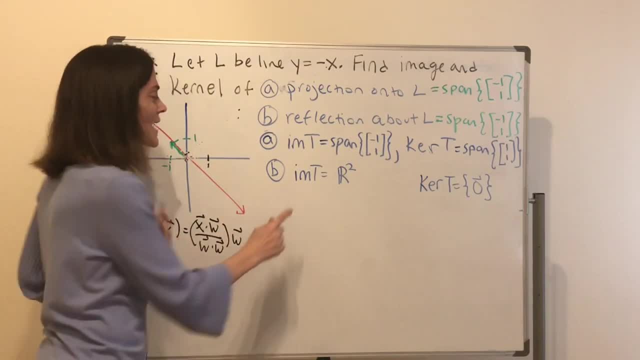 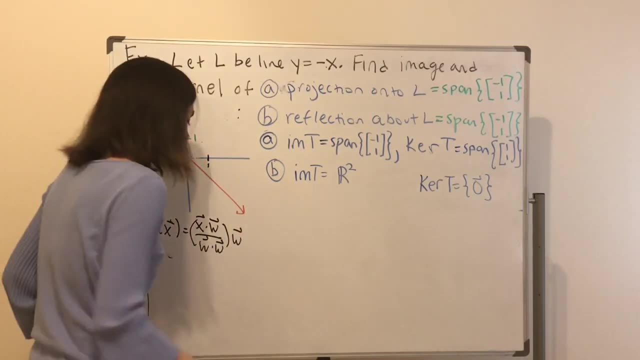 If not, it's okay, because pretty soon we're gonna talk about how to find this, how to find this, We're gonna talk about this from the matrices, But this is one that you can very much just think about with both of these reflection and projection. 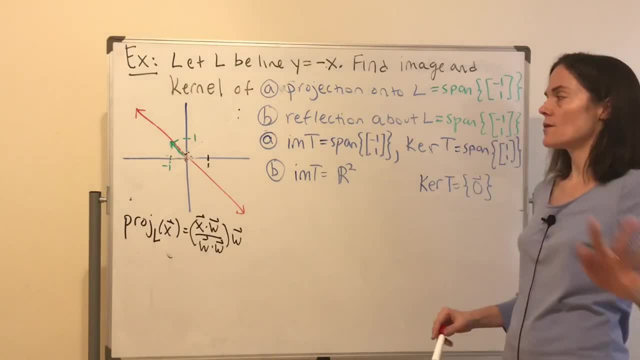 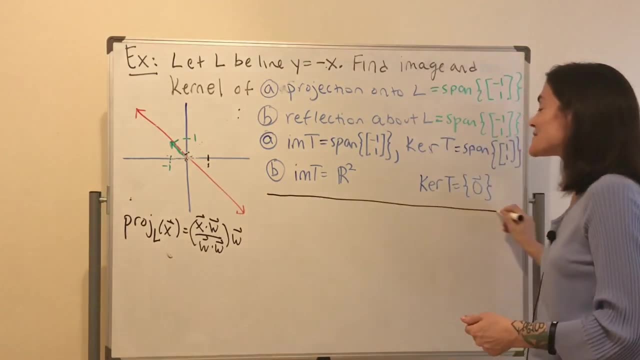 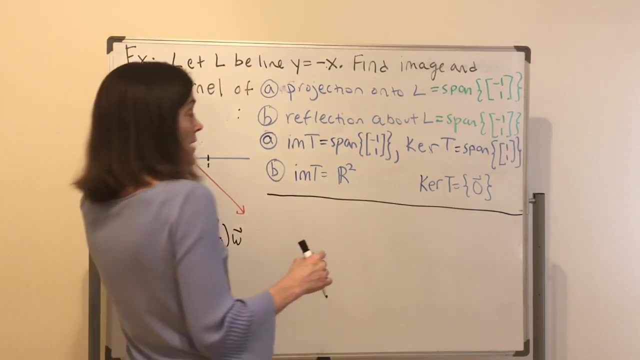 You can think about the geometry to analyze what's the kernel, what's the image. Now let's write down the matrices for these two linear transformations, because I want to make a comment about that, While the projection here is my vector. 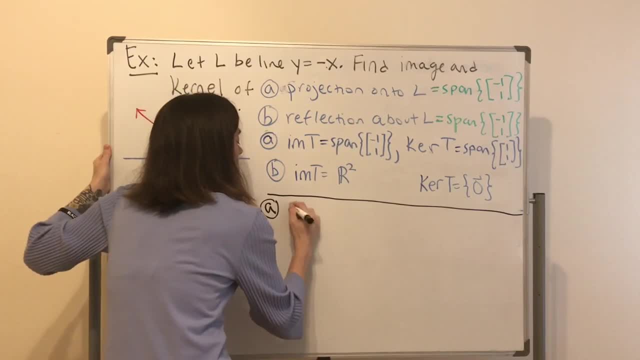 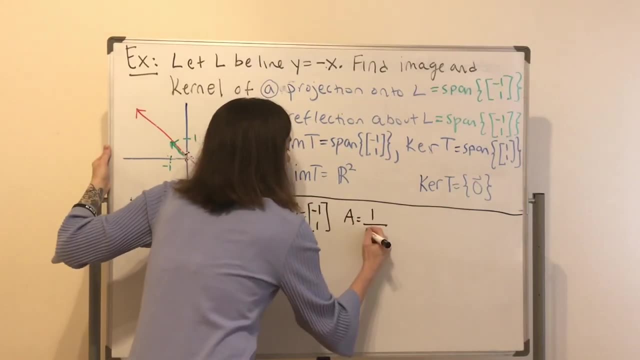 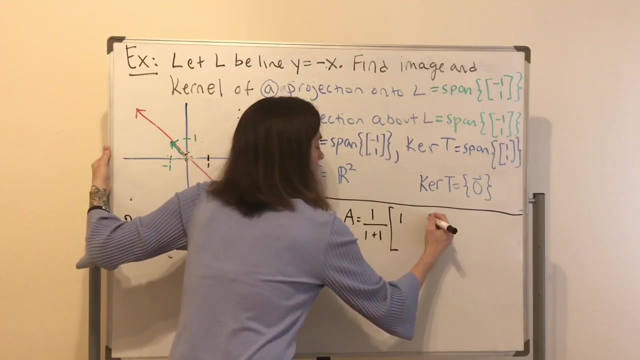 so for A let's find the matrix. W is this: It's not unit, but that's okay. So the matrix will be one over w one squared plus w two squared, And then we have w one squared, And then here is w one times w two. 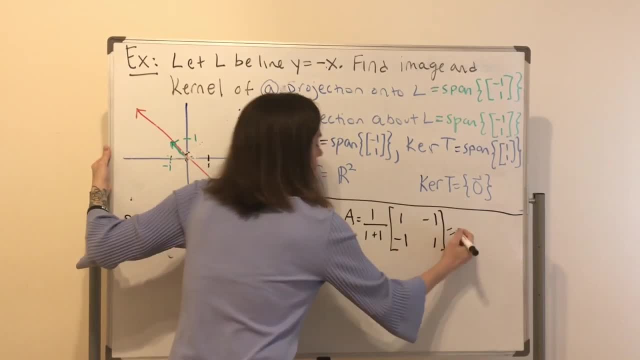 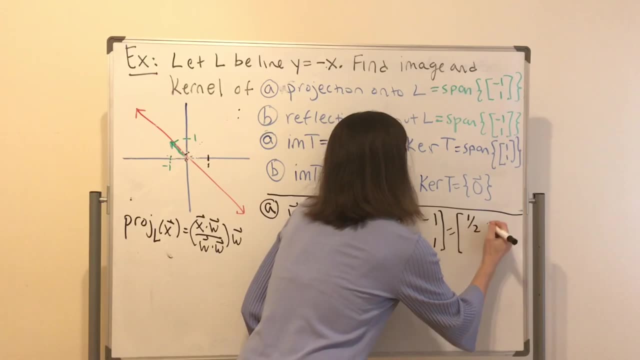 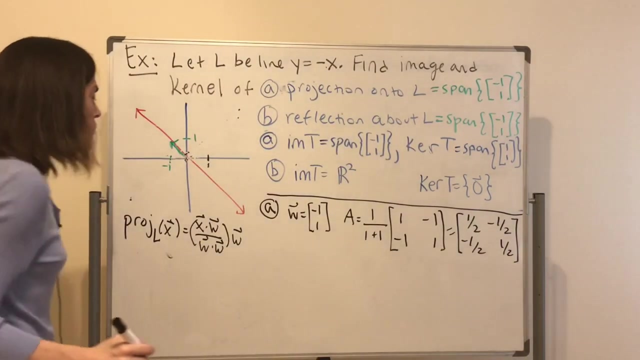 w one times w two, w two squared. So this is the matrix for projection, And if we write it as one matrix, we get a half Negative, a half negative, a half a half. Okay, Well, what about reflection? 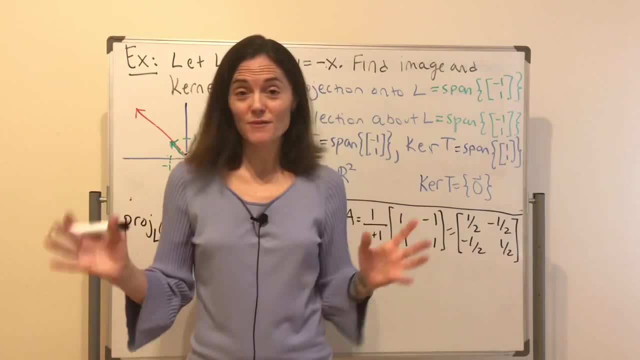 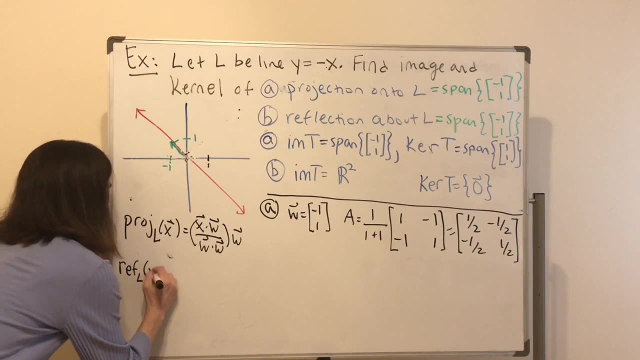 Now the way that I did it in the video, and if all I had to do was reflect, I would just take: well, let's write the formula: Reflection is it's two times the projection minus. like this, This is what reflection is. 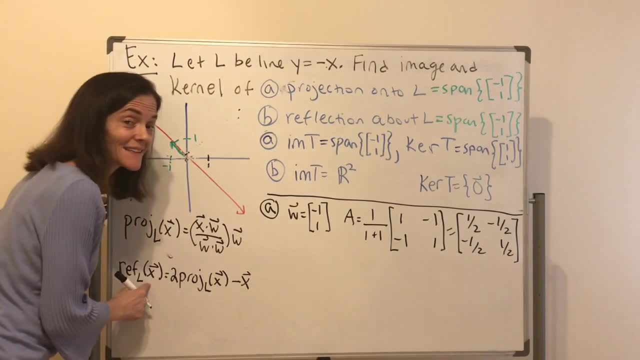 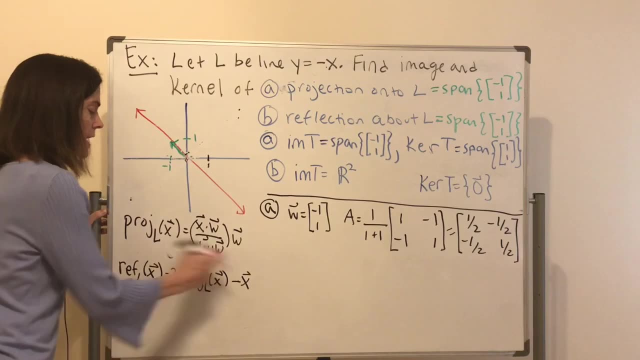 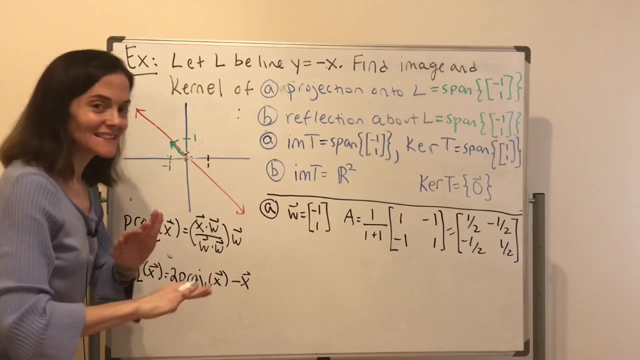 And this is projection And the way that I found it in the video and maybe did my homework, is you just find what happens to E, one okay, Under this map, And then that forms like a look at AB And then you put B minus A. 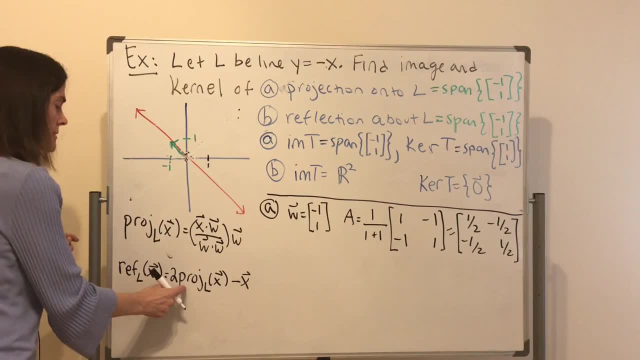 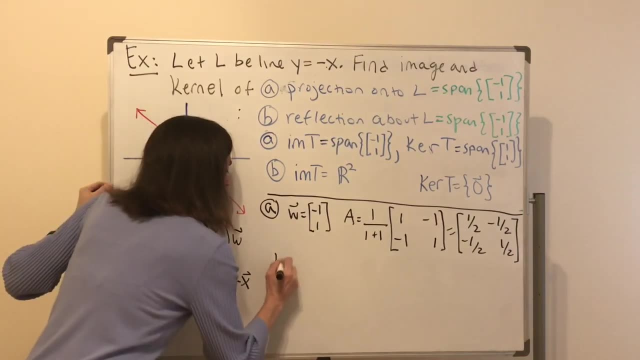 This is the matrix. But also just looking at this and understanding what we know about transformations and matrices, I can, right here, I can write the matrix, Write the matrix down, because I already have this one, So the matrix will be two times this matrix. 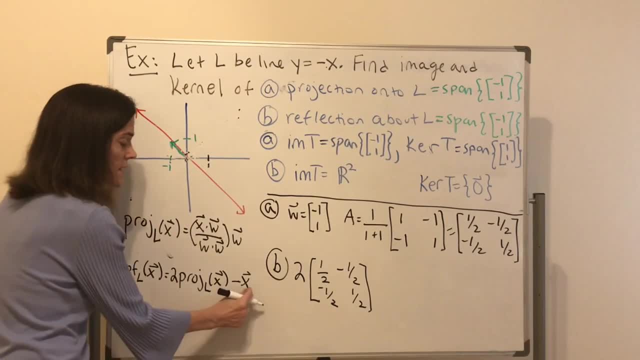 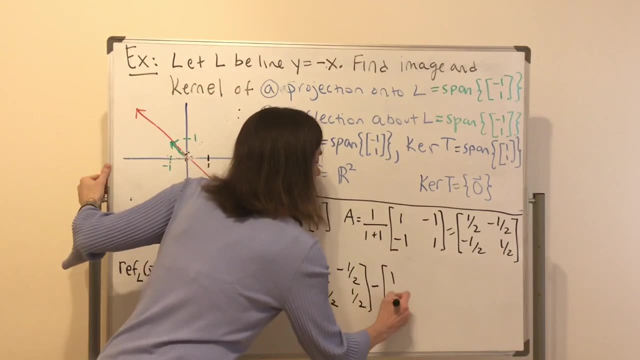 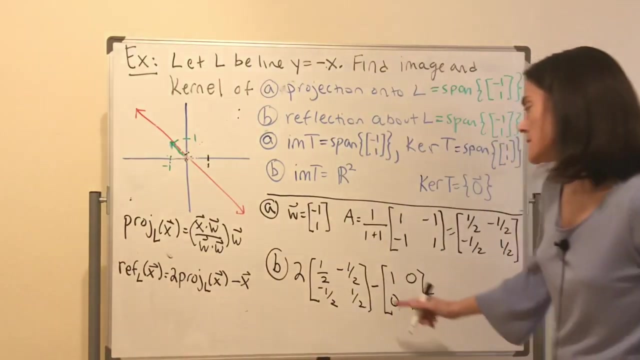 This is the matrix for projection, And then this is the identity. Well, minus one times the identity, So minus the identity. This is another way to find this matrix. What do we get here? This is one minus one zero. This is minus one. 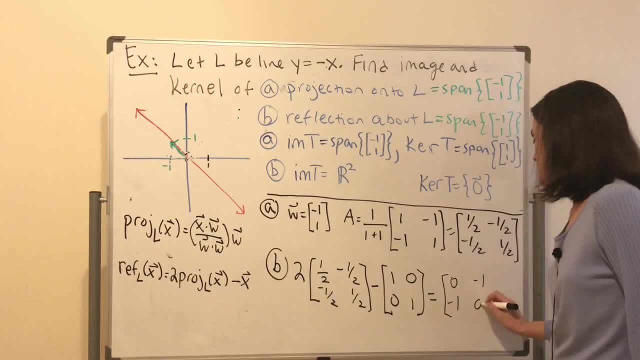 This one's minus one, And then one minus one zero. So this is the matrix for reflection, And this is B, And this is the matrix for projection. Now let me make some observations, then we're gonna move on. Now let me make some observations, then we're gonna move on. 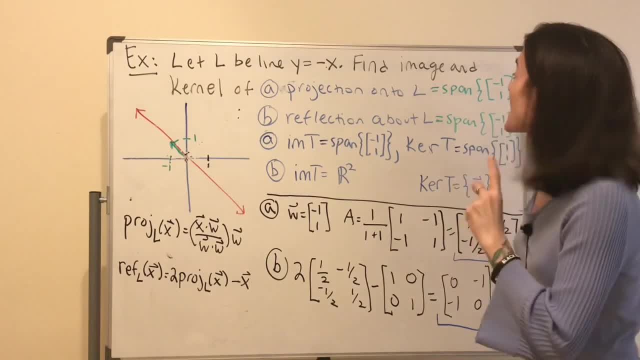 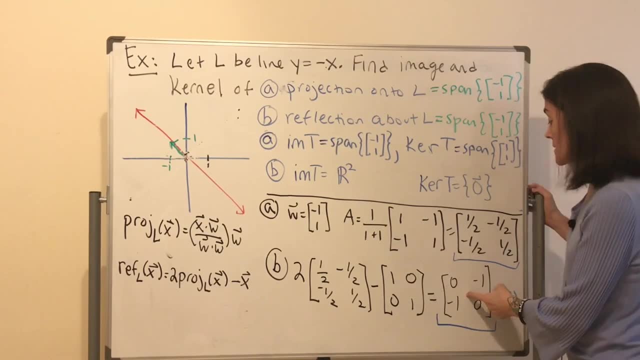 We're gonna move back to speaking generally about kernel and image. What do we see? Well, this matrix has rank two. How do you see it? Interchange the two rows, Multiply three by minus one, to each row, say, And then those are elementary row operations. 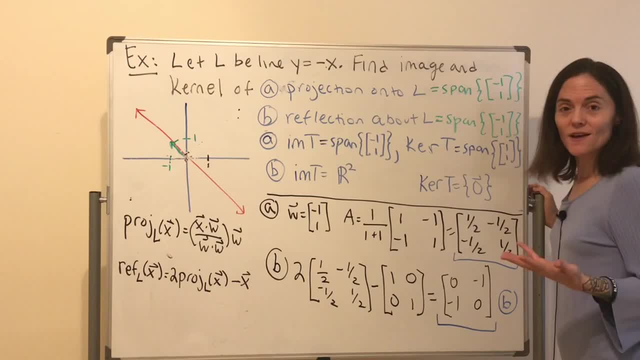 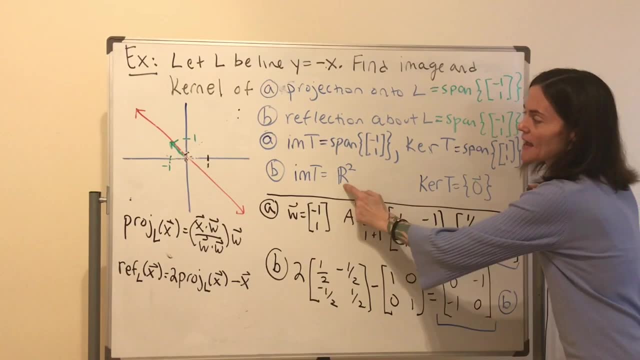 You will have one zero as your reduced row echelon form. This has rank two And you see we have a rank two matrix And you see we have a rank two matrix For the transformation that we have that the image is R2,. 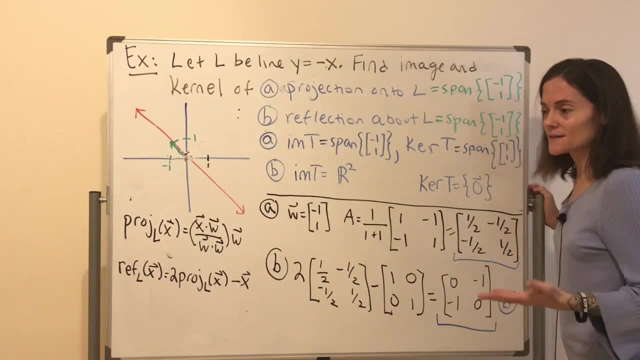 and that the kernel is zero is two by two. This is not. this is not by chance. Okay, but then what's happening here? Well, the observation I wanna make at the moment. look look at this column: One half minus a half. 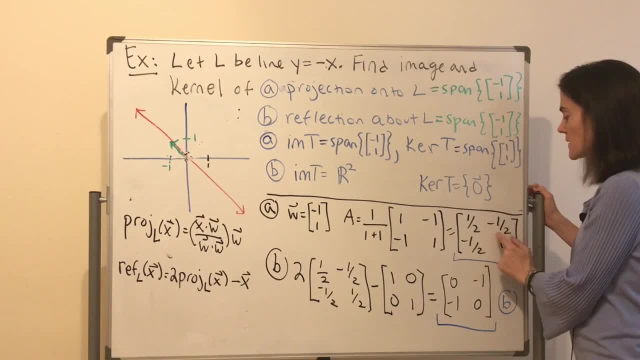 Look at this column Minus a half one half, Both of these columns. here they're in this span. This column is negative a half times this vector. This column is one half times this vector, And well, similarly, both these columns are in here. 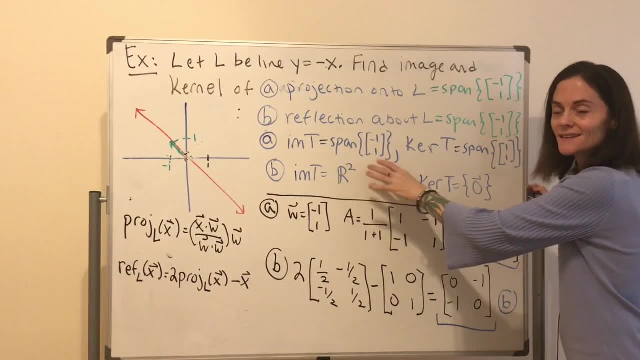 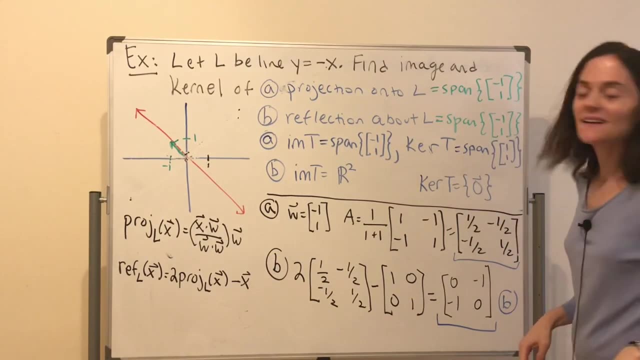 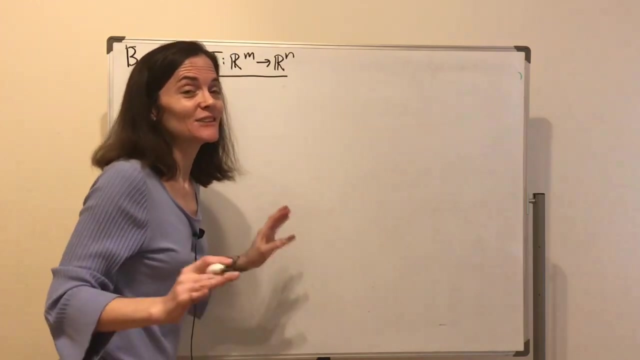 So we see the columns are appearing in the image, And that's the other comment that I wanted to make. Okay, let me erase. Now I wanna go back to transformations from RM to RN. Okay, not just two by two. So when you have a linear transformation, 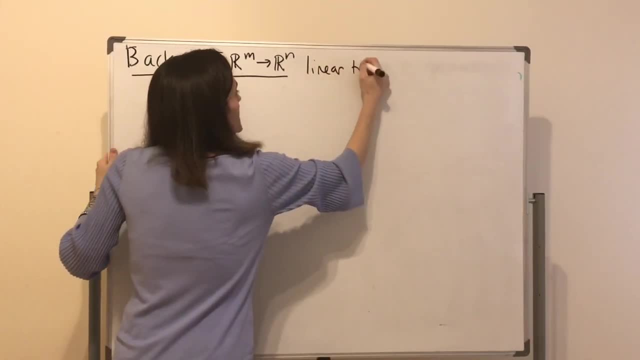 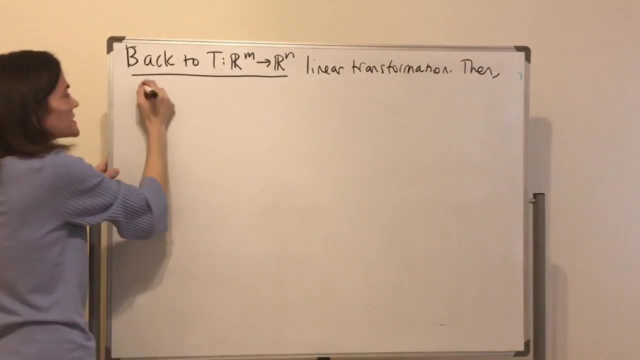 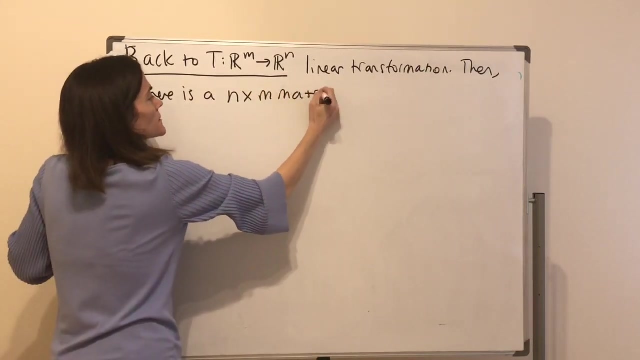 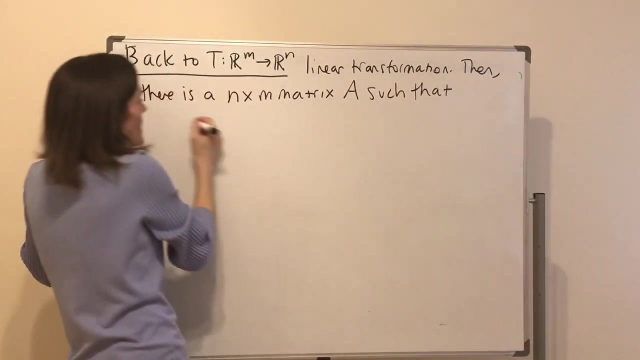 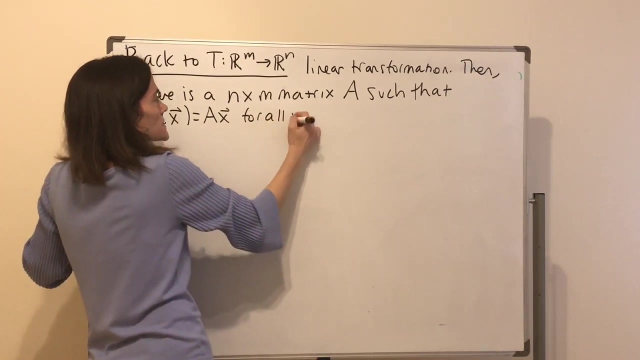 well, of course, linear transformation. Then, what do we know? Well, the definition is: there is A, it's gonna be an N by M matrix A, such that, well, T of X is A times X for all X in RM. 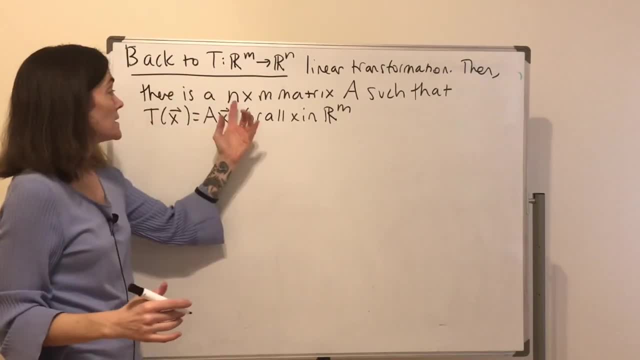 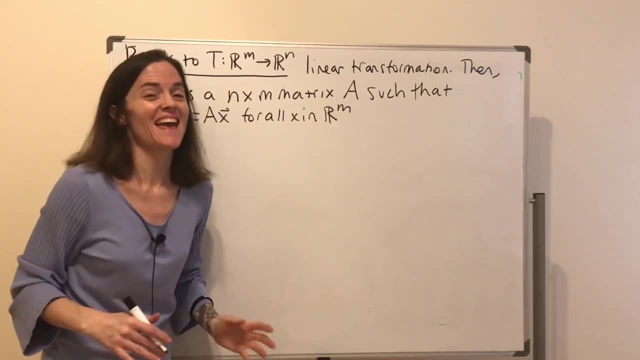 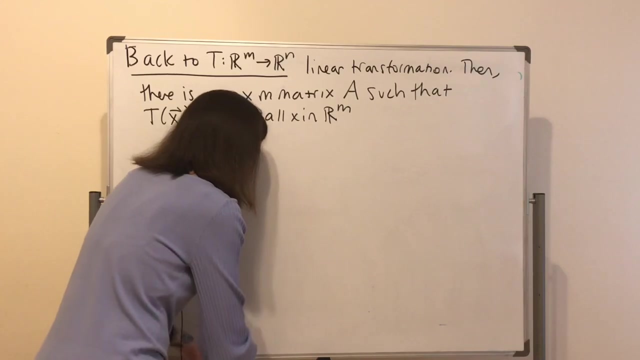 Right, this is the domain And, without a doubt, if you are N by M, you could certainly multiply by a. this would be a M by one. Okay, everything's working out in terms of dimensions, So let us talk about the image and the kernel. 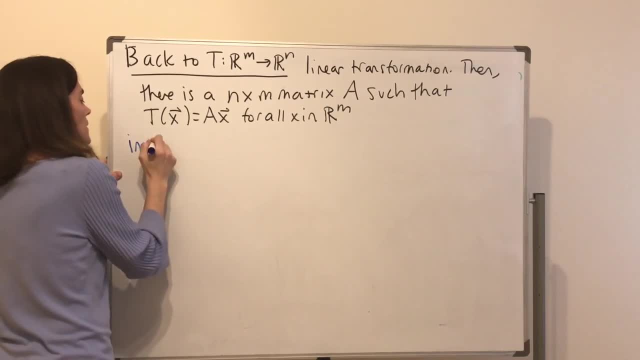 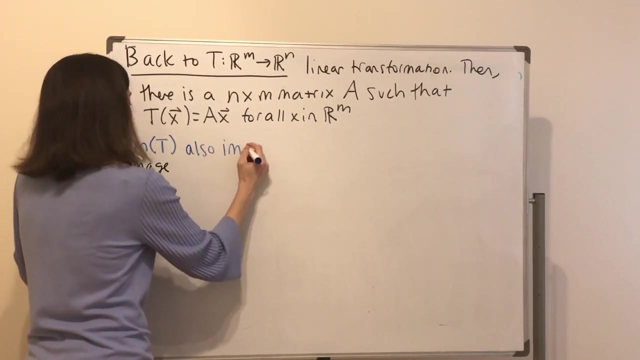 So first of all, there's the image of T. This is also. this is the image. don't write that underneath. this is the image. This is also written like this: The image of A. So these are the same thing exactly. 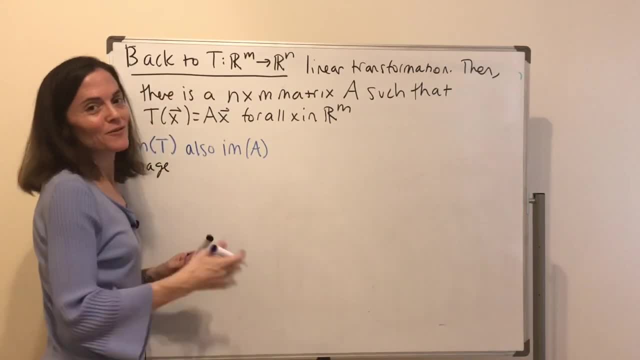 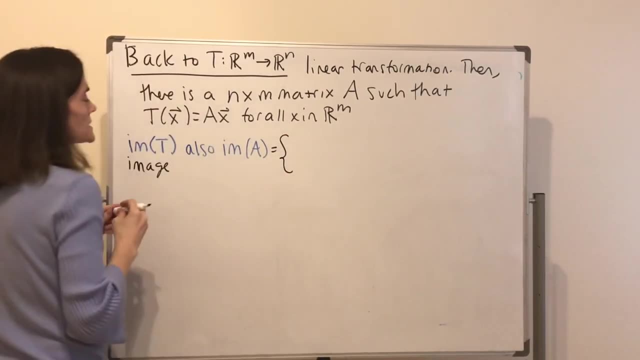 Just sometimes you might refer to it as image of a matrix, Sometimes you might refer to it as image of a transformation. Okay well, let's write with this. Okay well, let's write with this. This is all if I think about it in terms of the matrix. 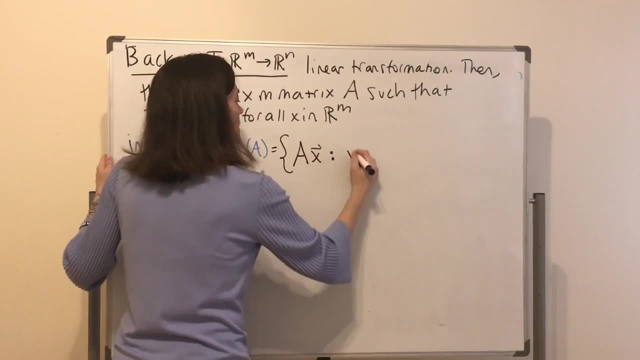 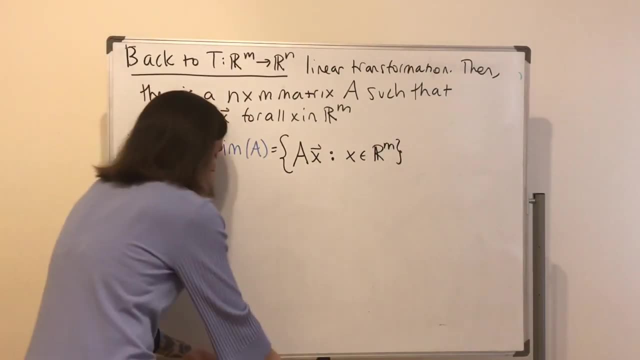 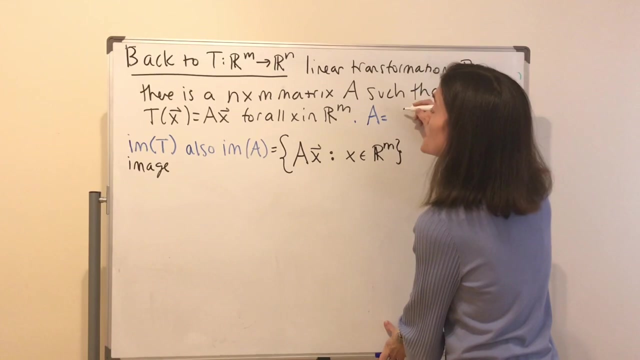 it's all AX, such that X is in RM. Now let me add more to this picture, because we're about to go further with this. Let's suppose A we have M columns say our columns are V1, V2 to VM. 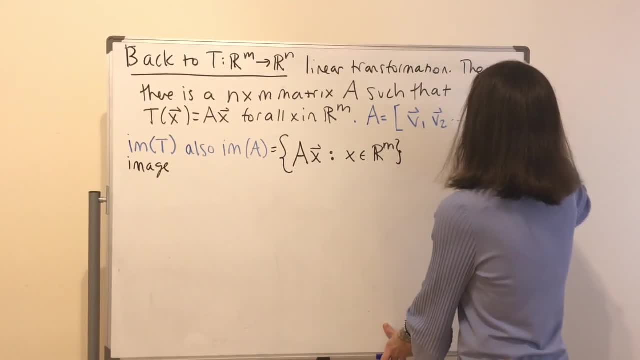 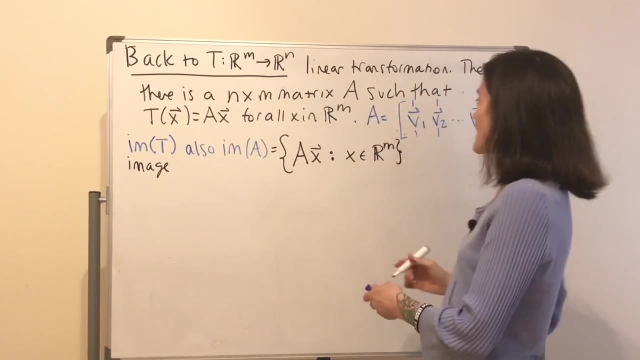 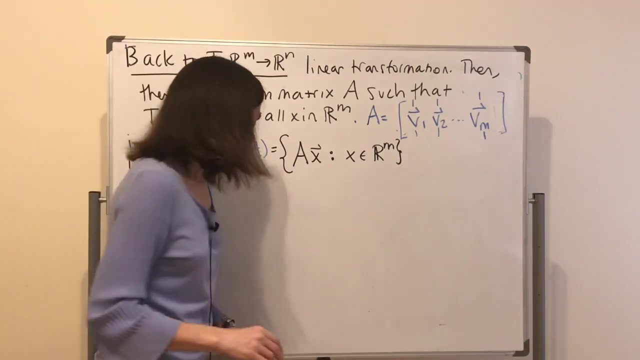 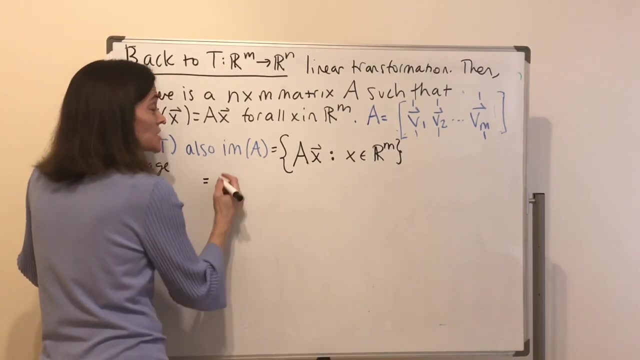 These are columns And I'll make this a little bit taller. Okay, here's my columns. Well, we had a column picture for understanding AX and this is important today. This okay, This okay. We may write as a linear combination of the columns. 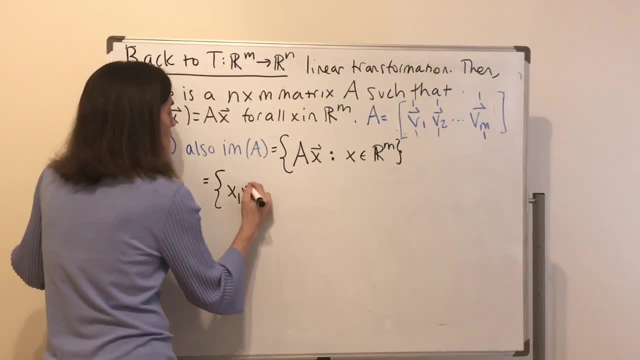 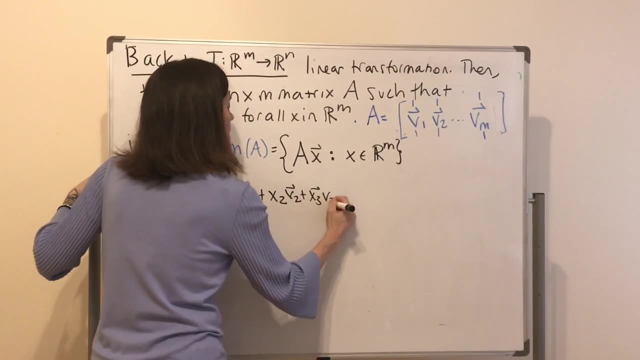 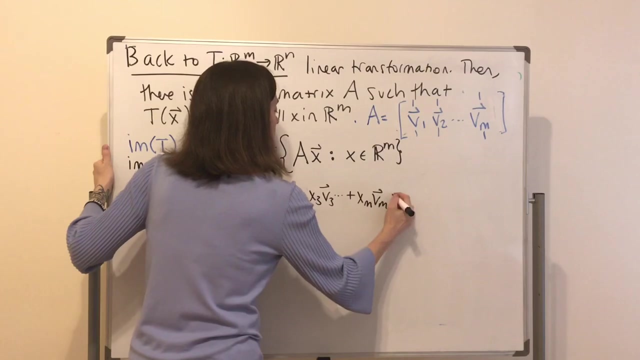 So here this would be say X1V1, plus X2V2, plus X3V3.. Uh-oh, wrong place to put my hat. And all the way out to XMVM, such that XI are real numbers. 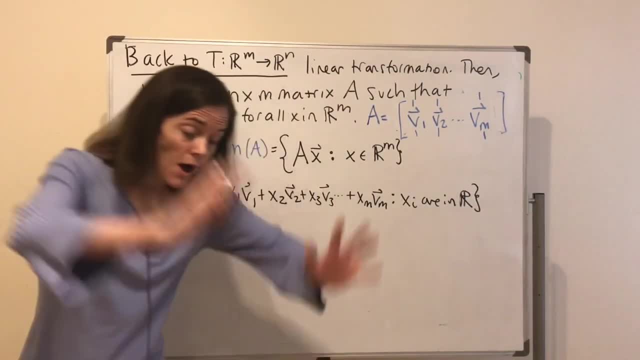 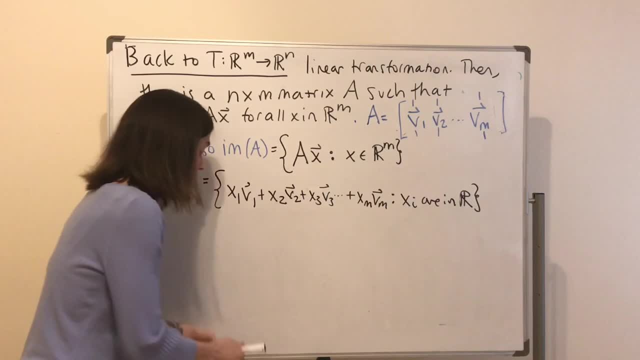 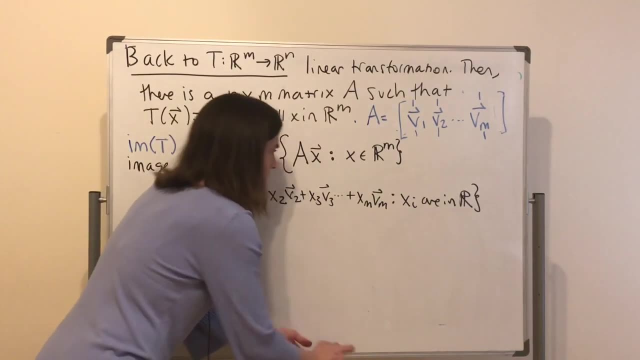 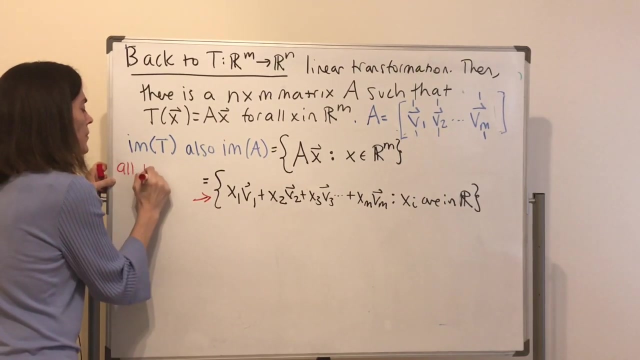 And so this would be all possible. Well, what is this? This is all possible linear combinations of the columns. So the image here- I'm trying to figure out what color to write This is, I'm going to erase, find the space. all possible linear combinations of the columns of A. 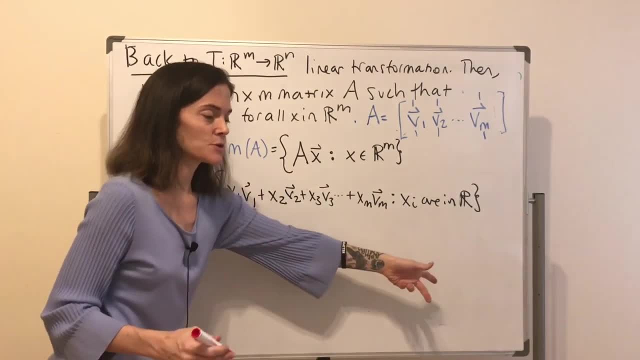 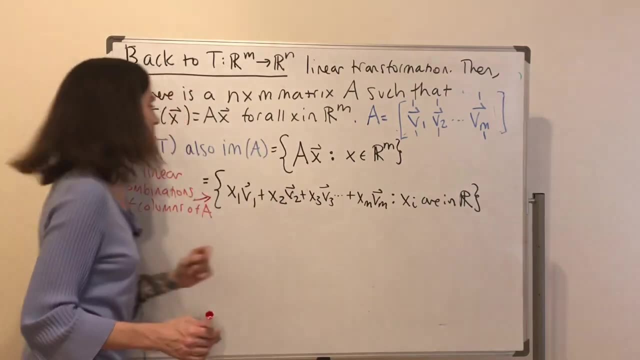 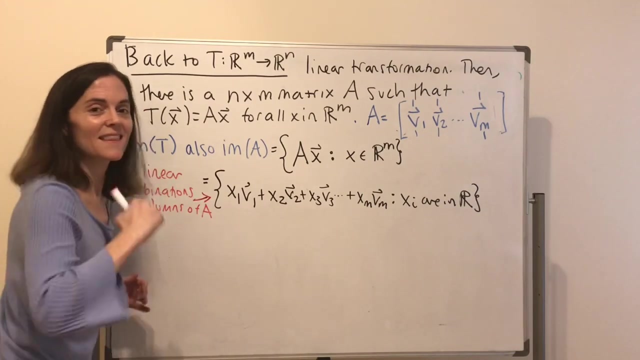 And this is what we saw in this geometric thing. When I wrote down the matrix, we realized that the columns were in the image, For example. but you take all possible linear combinations of the columns of A. This is the image of A, the image of T. 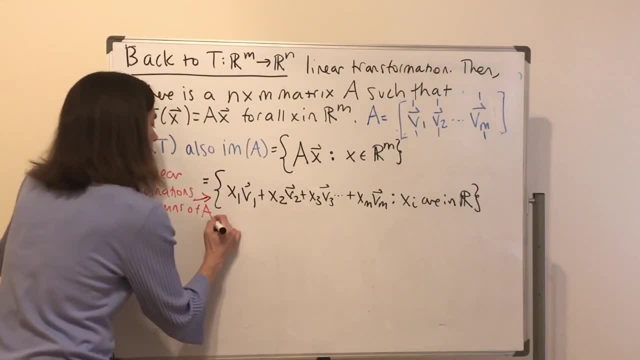 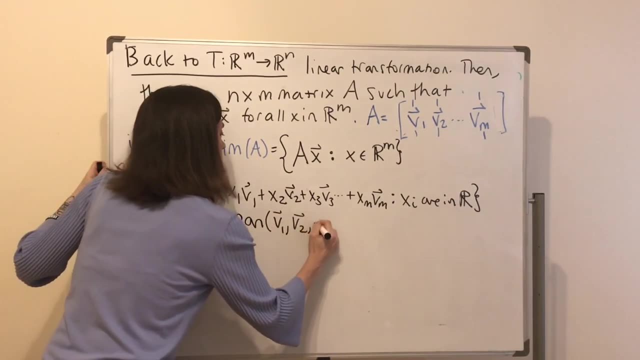 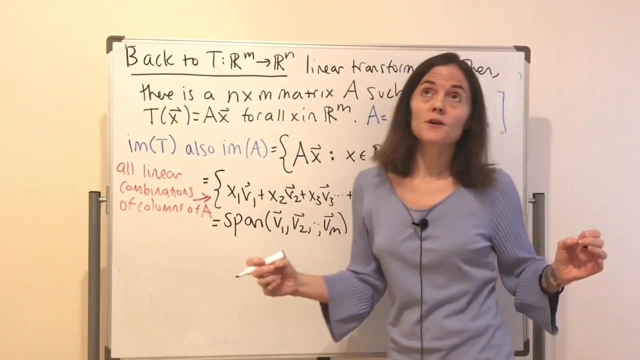 Okay, well, how else could I write this? I could also write this as follows: Span of V1, V2, up to Vm. I referred to span of one vector. It said it was all multiples of the vector. I started talking about that when we did orthogonal projections. 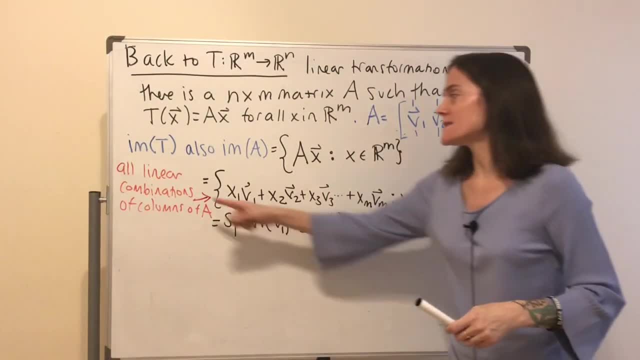 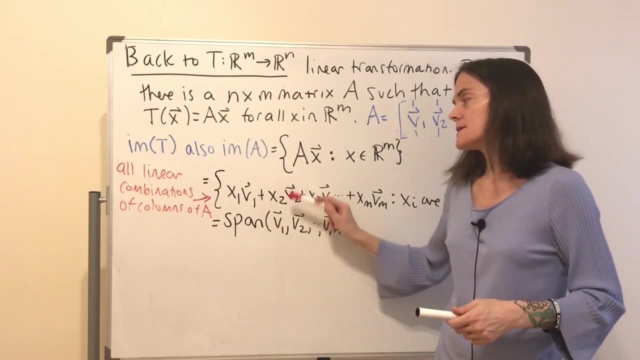 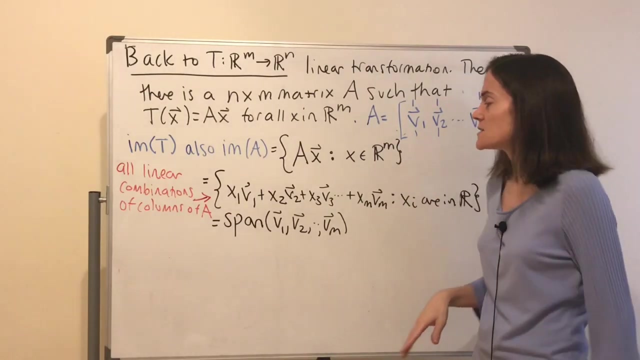 Span of a collection of vectors. Well, it's this, All possible linear combinations of that collection. So this and this are the same. Span is just another way to say it. Instead of writing all of the coefficients, x, i's, you just say, oh, it's a span of these vectors. 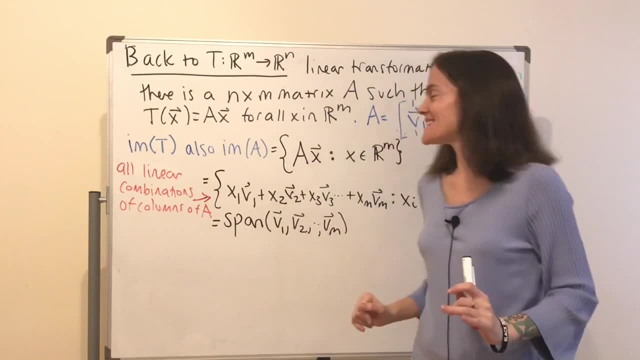 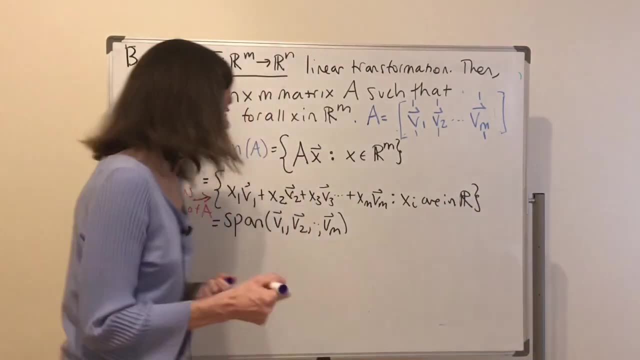 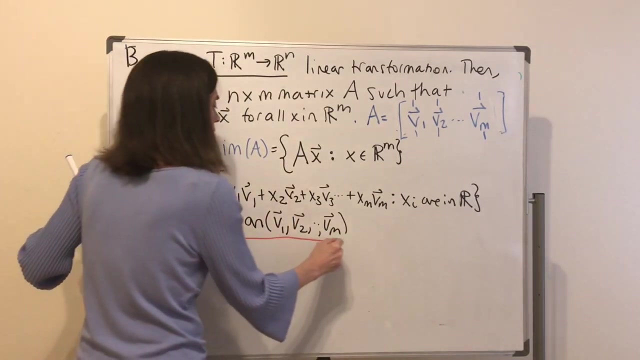 And that means you take all possible linear combinations, just like this. Okay, so this is the image. Now I'm going to talk a little bit about the kernel. Then I'm going to start: instead of looking at them together, I'm going to look at them one at a time for a little while, because they're both worth thinking about. 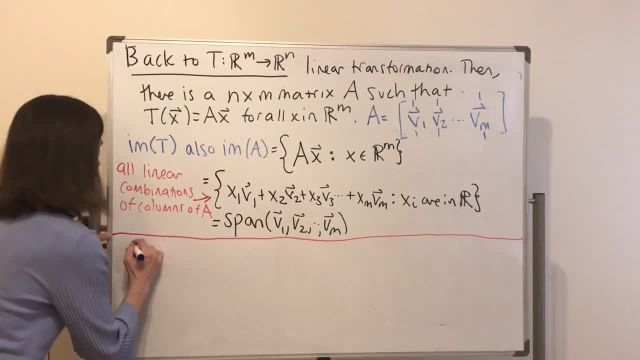 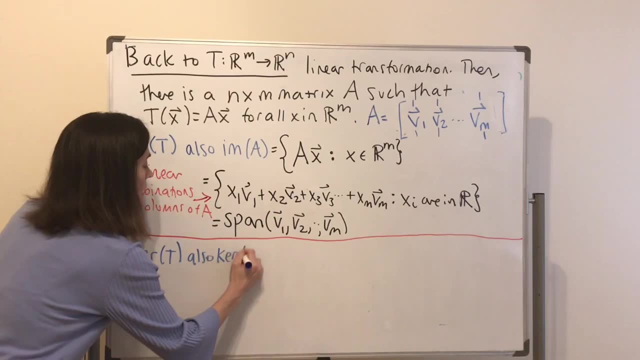 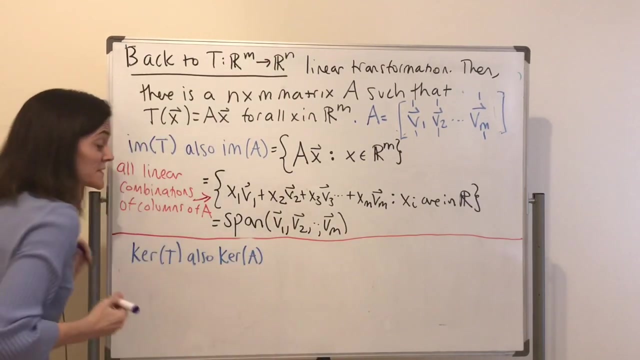 Okay, what about the kernel? Also, it's called the kernel of A. Okay, maybe I should put parentheses. Same thing, just like with image. you might refer to it as a kernel of a matrix or a kernel of the transformation. 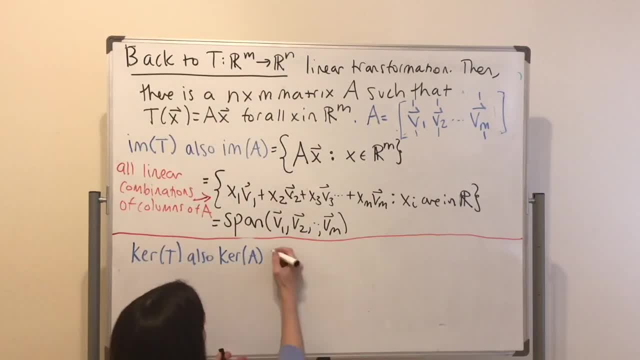 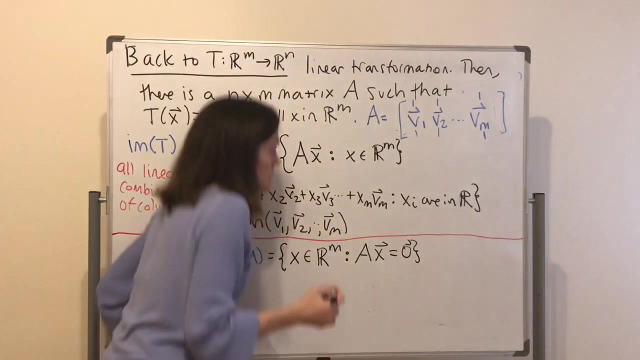 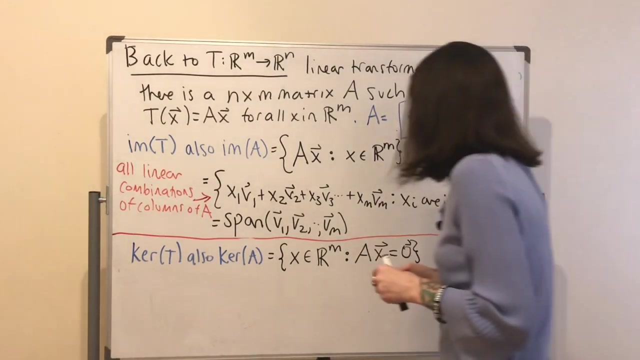 So let's write this in terms of the matrix: This is all x in Rm, such that Ax equals 0.. Okay, Okay, See, did I want to say anything else? Not really, It's just all solutions. Maybe I'll recopy. 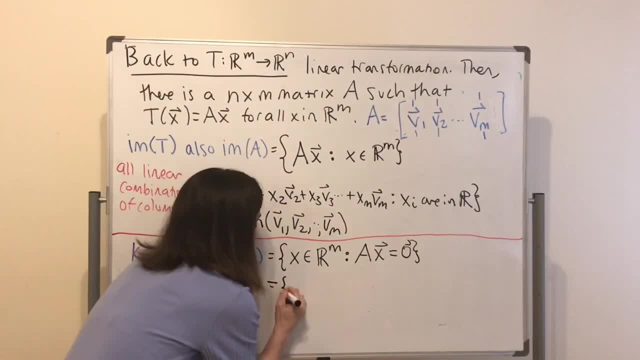 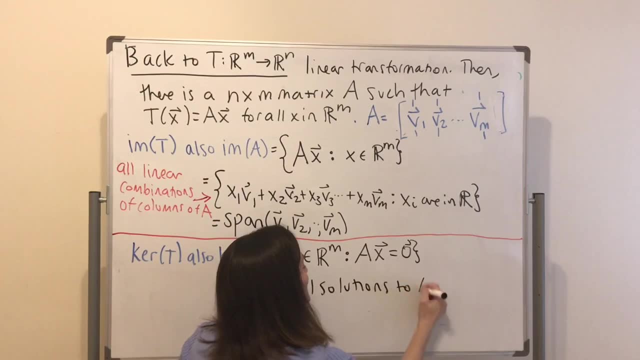 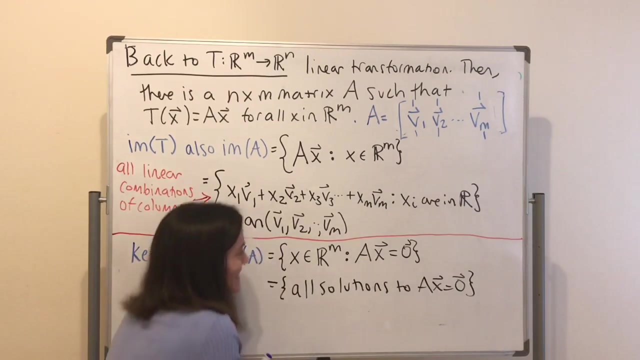 I didn't have so many fancy ways to rewrite it. That's why I'm going to look at my notes. It's just all solutions to Ax equals 0.. And then I will make one more comment before we get into some examples. This look, I'm starting this. 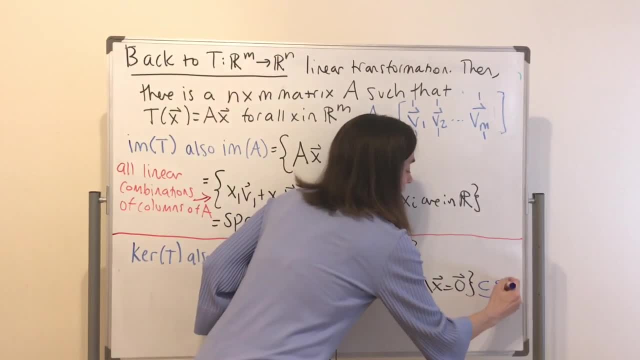 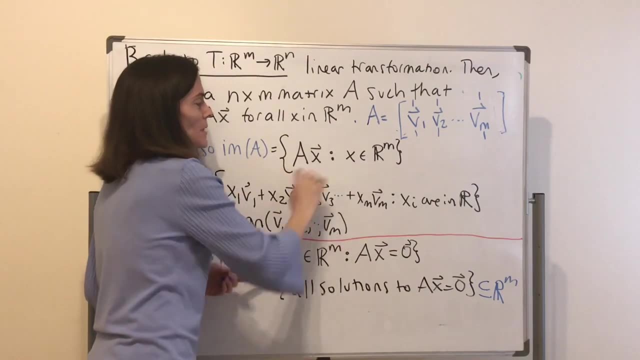 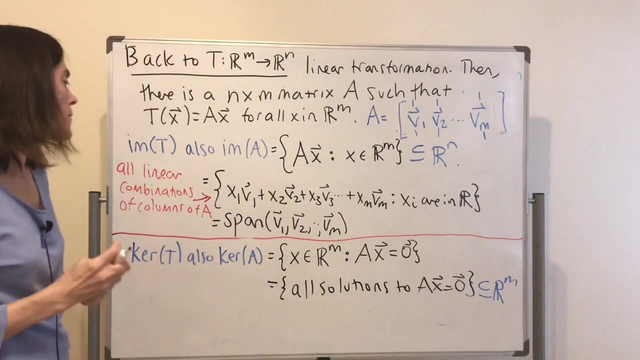 something in Rm. This is in Rm, as I mentioned at the very beginning. And then here these are. well, if you take x, you multiply by a, these are in Rm And I also mentioned that at the beginning. but it's good to observe. So we're going to now, I guess, the nice thing. 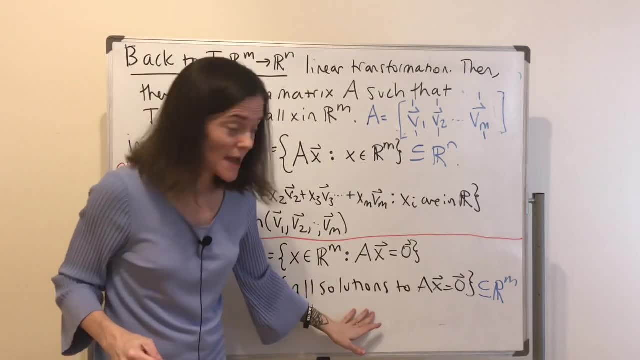 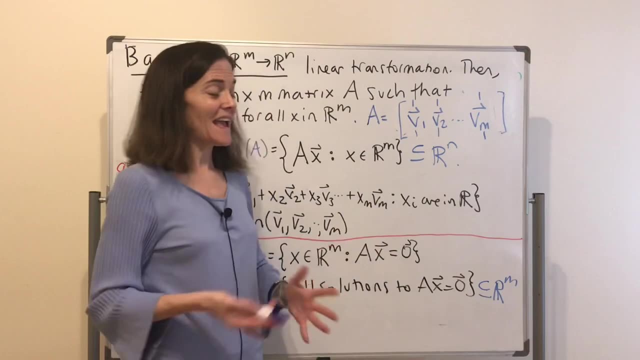 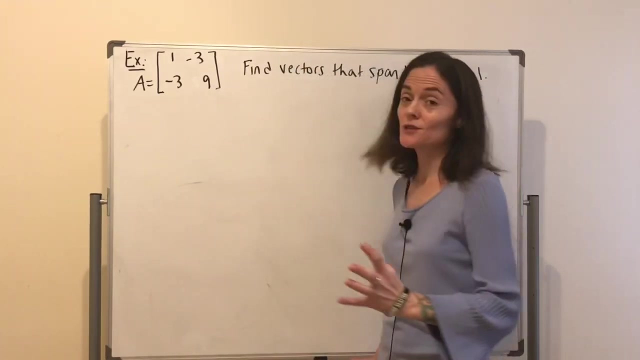 about realizing it this way. all solutions is: we know how to solve things like this, right, We know how to solve a x equals 0. And so we know how to find kernels. Great. Well, here's our first example. It's just 2 by 2.. It shouldn't take too long, We want. 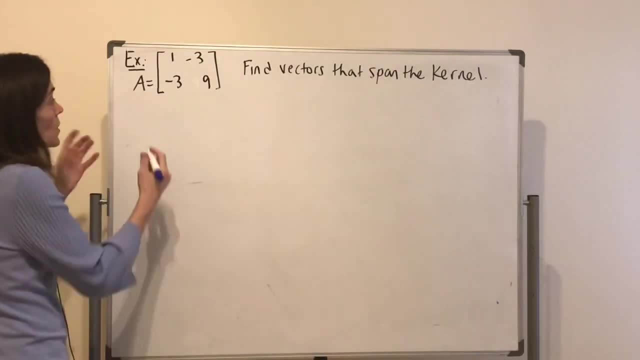 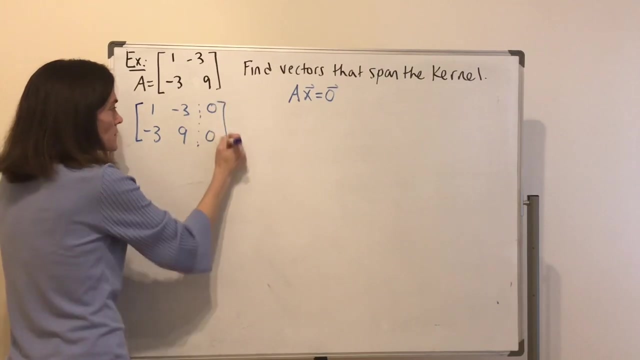 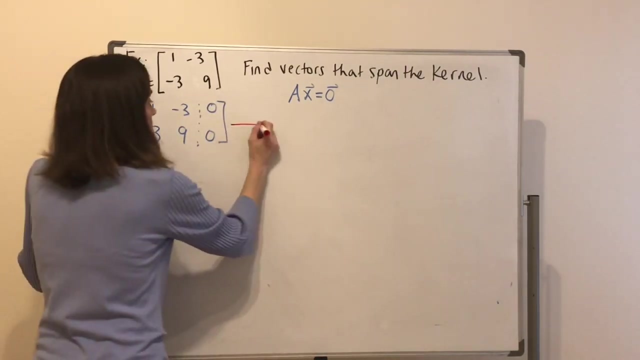 to find the vectors that span the kernel. So this one: how would I solve? right, I want to solve this system And I could take, augment the matrix, The zeros, Okay, And then I perform elementary row operations, And when I do this it doesn't. 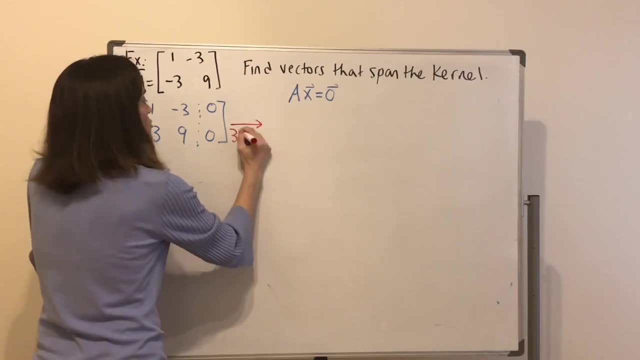 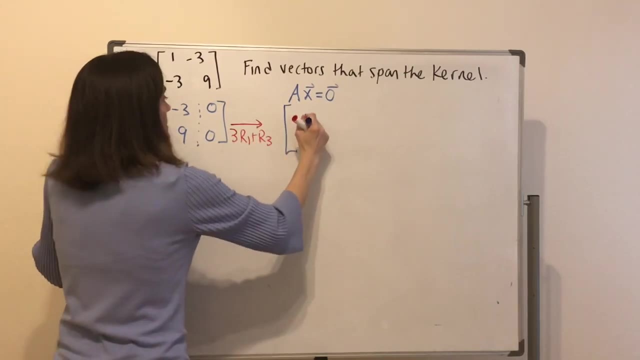 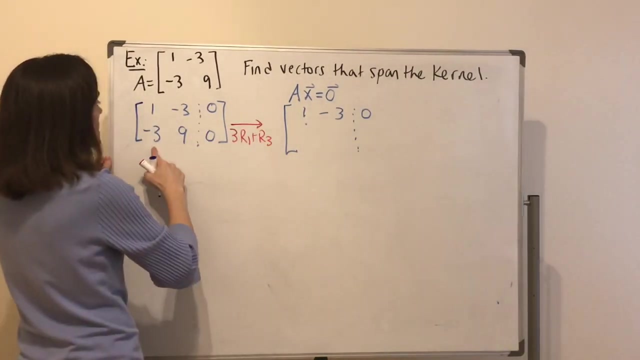 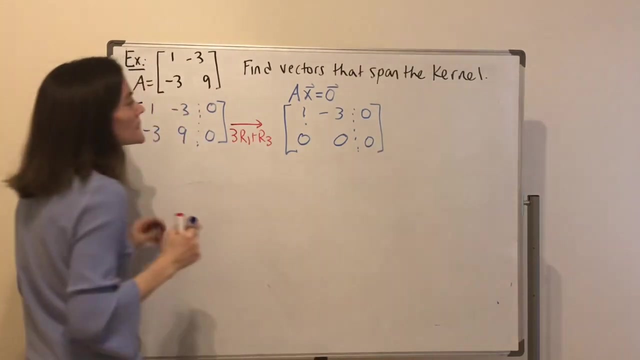 take me very long with this matrix. I take 3, row 1, add a 2, row 3.. And what do I have? I have: row 1 remains the same. Row 3 is now 0.. 0, 0.. Okay, We see, this matrix has rank 1.. We have a leading 1 in this column. It means 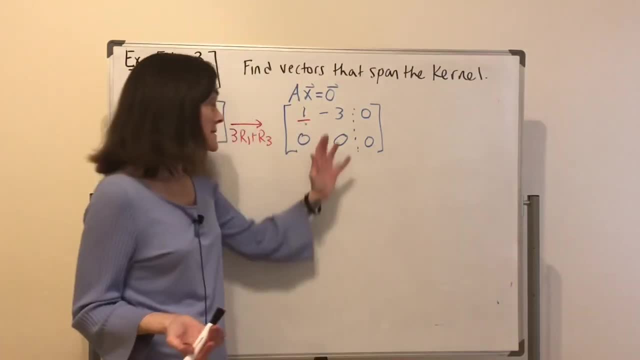 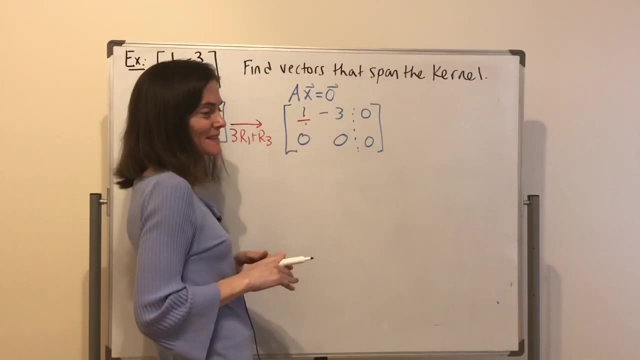 and this is a nice review of some things that we have already discussed- it means that this corresponds to a free variable. So what I did in well, last week's videos, for example, is: I would say x, say x2,, for example, is: 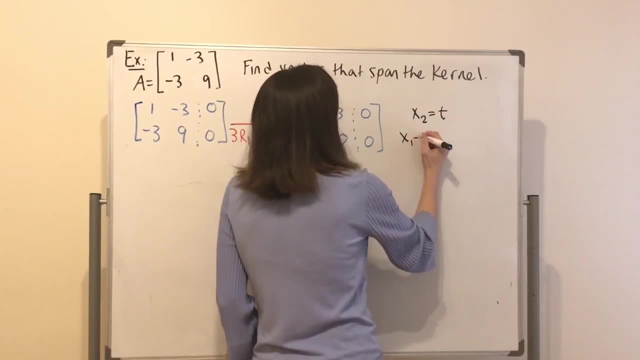 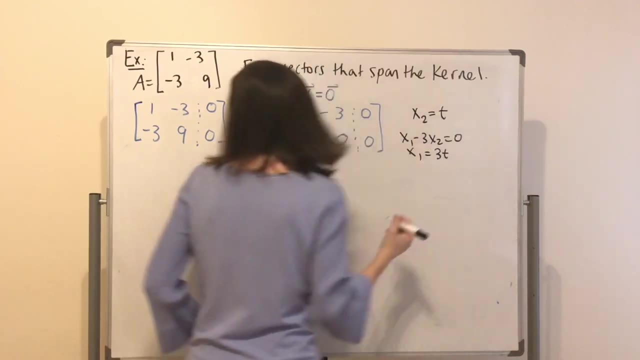 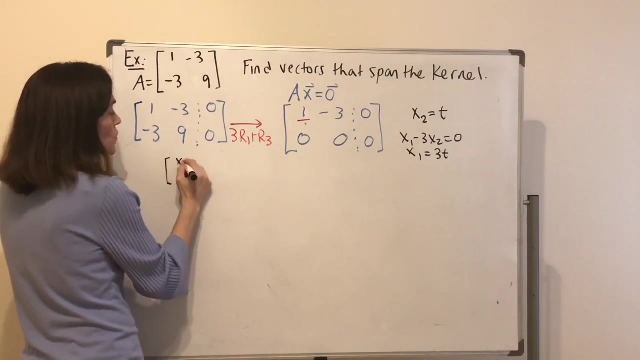 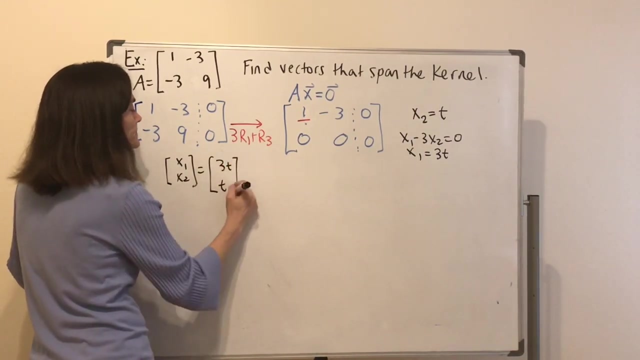 t, And then we see x1 minus 3x2 is 0, gives us that x1 is 3t, And so we get the following: as we get the following, x1, x2 is, if we just write it, t, 3t, And this is how I would have. 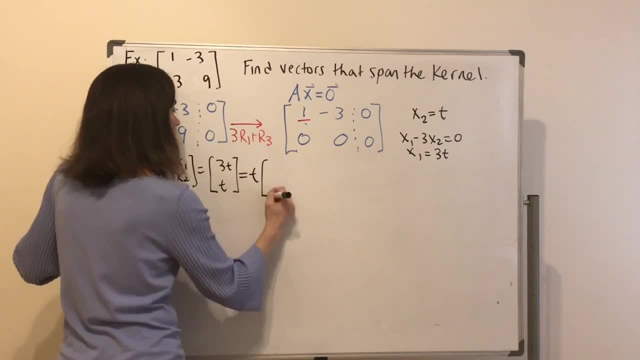 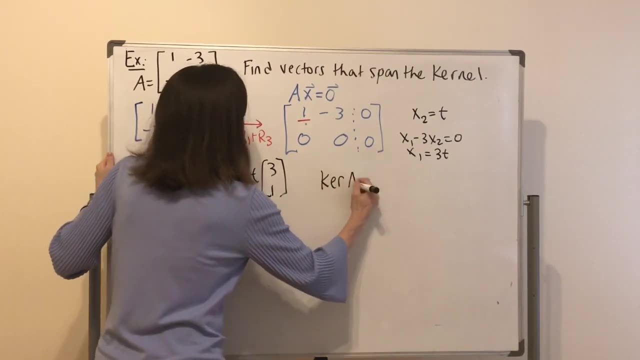 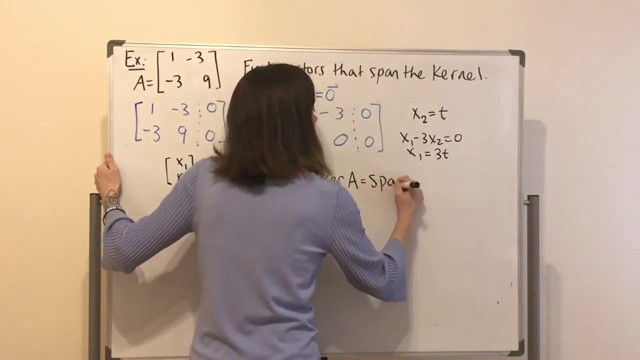 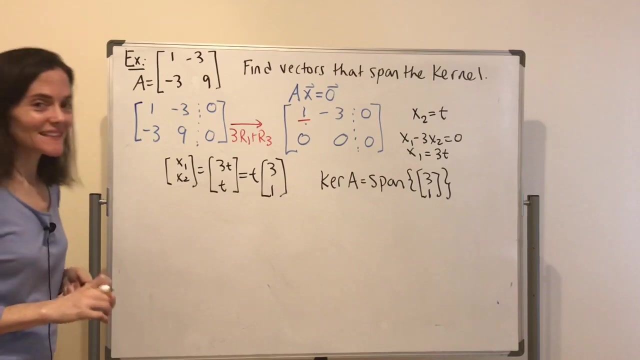 done it last week- Which then you can write like this: And now you see, this is the vector. So the kernel of a or the kernel of t, if you think about the corresponding linear transformation, is the span of 3, 1.. Okay, So far not too bad. This was a nice warmup. But one thing I will. 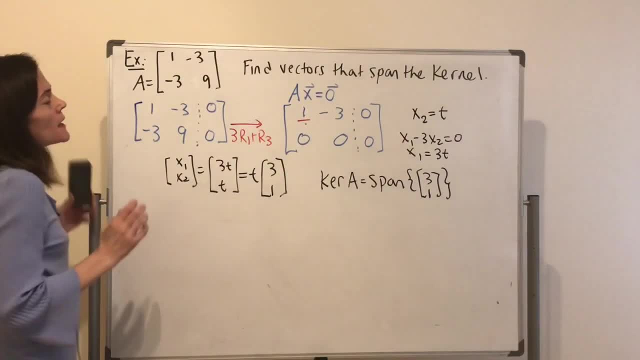 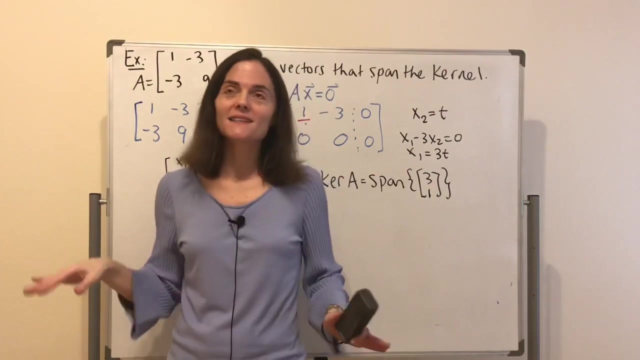 say before I move into a larger example: You don't really need to augment with these zeros, because if you have a column of all zeros, which this would be to solve, ax equals 0, no matter what operations you do: interchange two rows, multiply a row by a constant, add a multiple of one row to another- you're not. 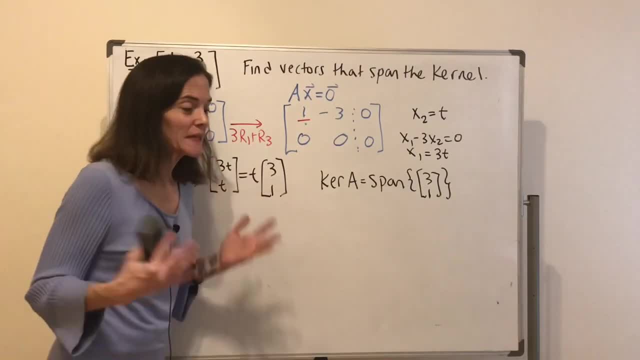 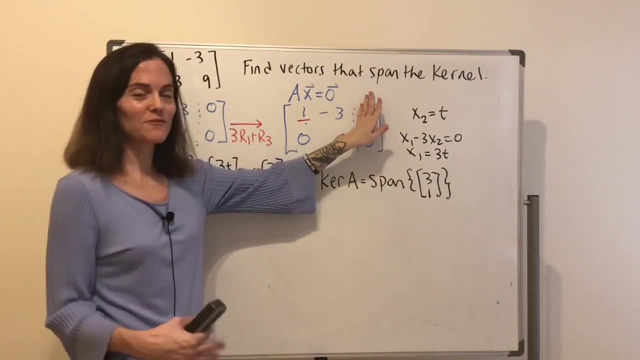 changing the fact that everything over here is zeros. So all you really need to do is find the reduced row echelon form of a, which would just be this in this example, and then you can read off the vectors that span the kernel, for example: 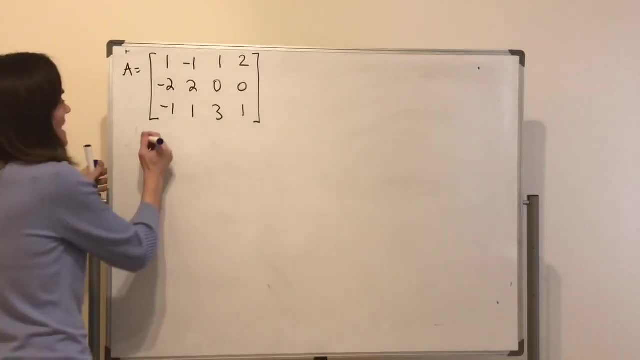 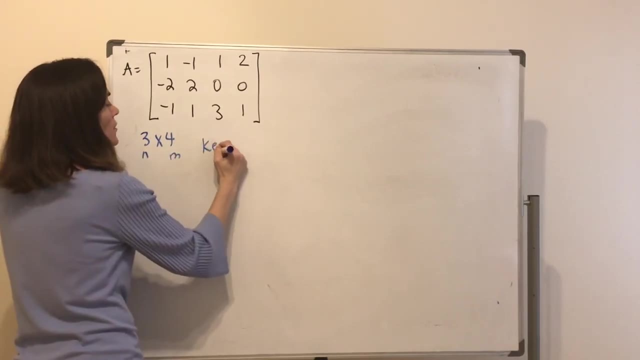 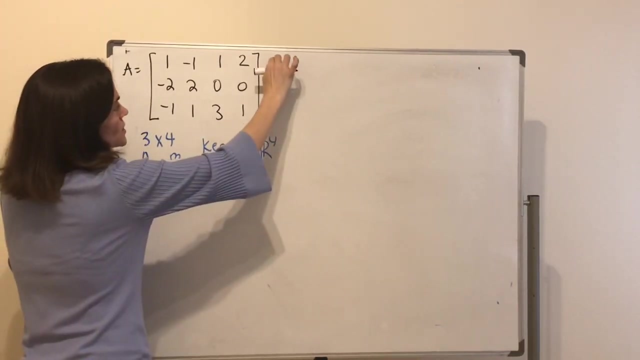 This is not square. This has three rows, four columns. If this is our n, this is our m, we will have that the kernel of this matrix will be a subset of r 4.. Well, of course, because what do you absolutely need to multiply? If you have 3 by 4, you need a 4 by 1.. And 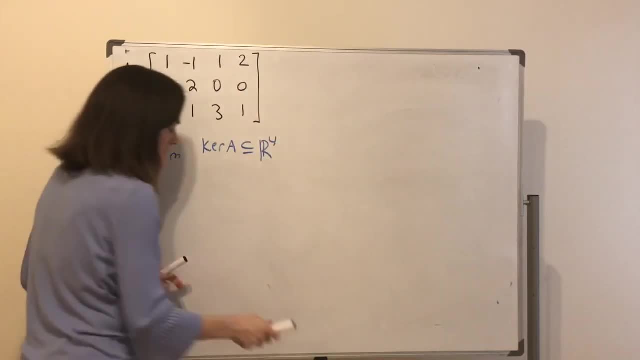 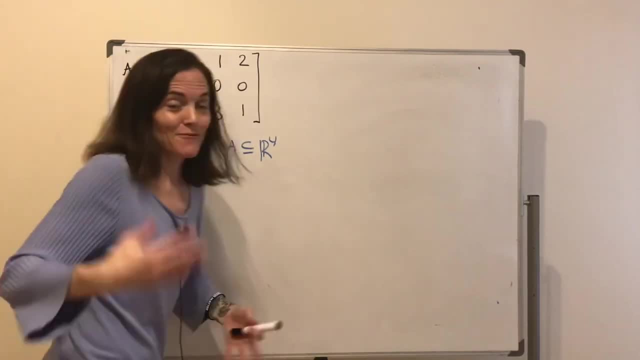 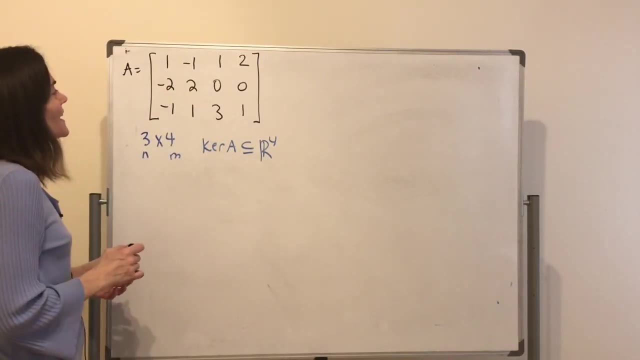 Okay, Okay, Okay, Okay, Okay, Okay, Okay. So what I can just do, if I what said the instructions not written down? same as the last problem: we want to find the vectors that span the kernel. I can. 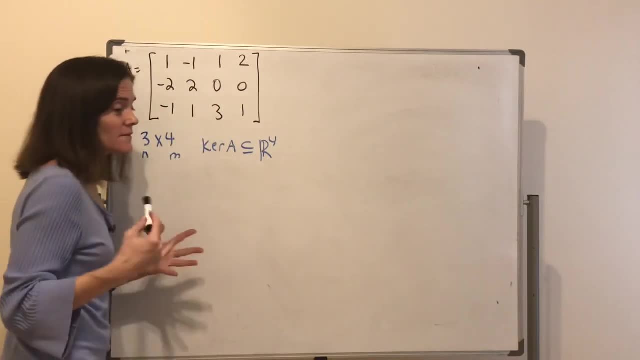 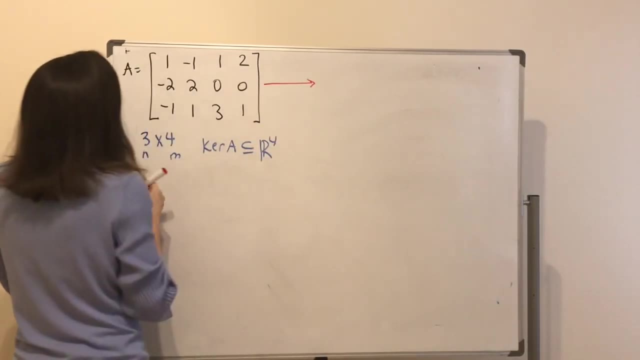 just start row reducing a. if I reduced row echelon form of a, as I mentioned in the comment, Okay, So I'm going to take 2 row 1, add it to row 2.. Take row 1, add it to row 6.. Take. 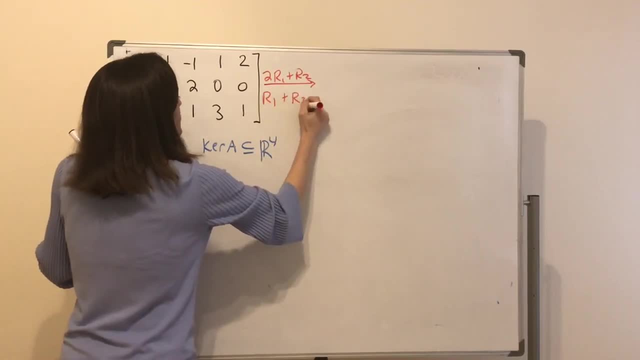 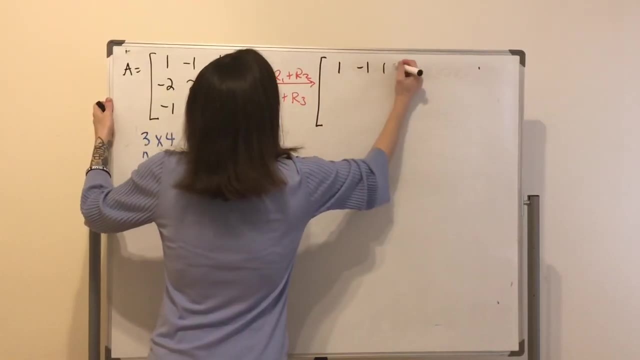 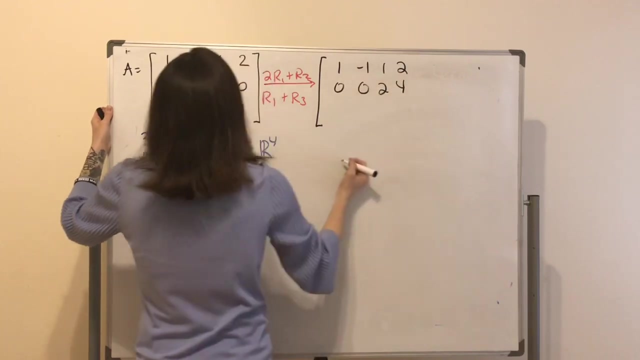 row 7, add it to row 8.. Okay, I'm going to take these two to the row 8, add it to row 1, add it to row 7.. Add it to row 3.. And what do I get? Row 1 stays the same. Row 2 is now 0, 0, 2, 4.. 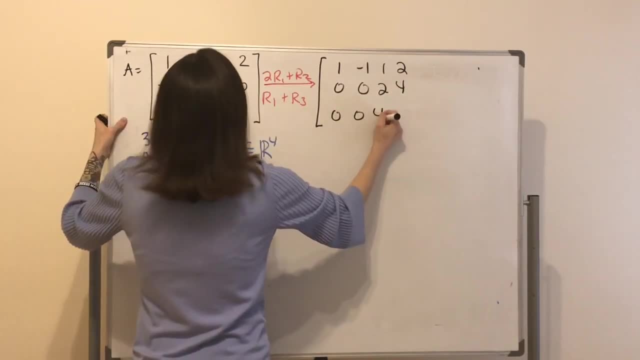 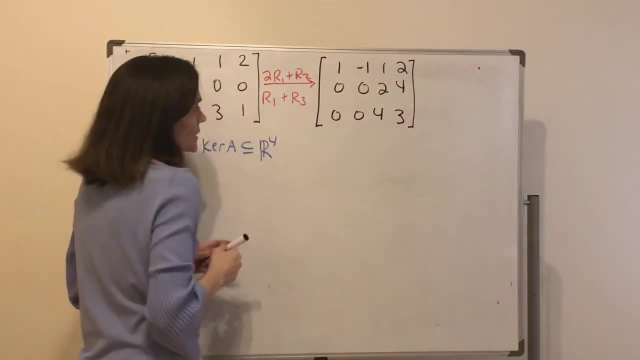 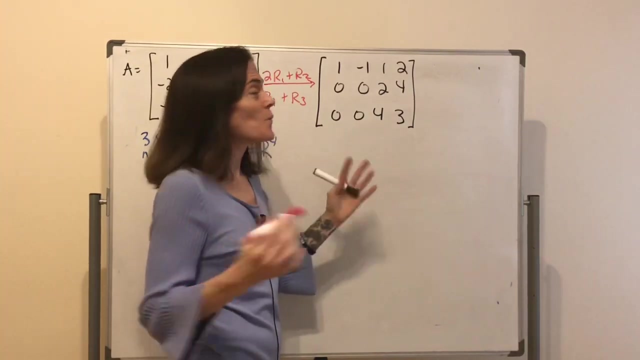 And then row 3 is now 0,, 0,, 4,, 3.. Is that right? Looks good to me. Okay, what's the next step? Well, you notice here in column 2, I will not have a leading 1.. 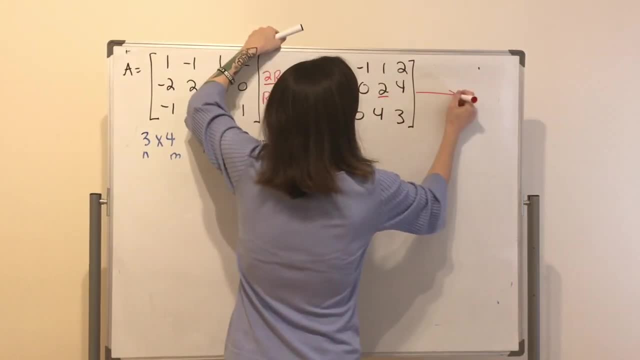 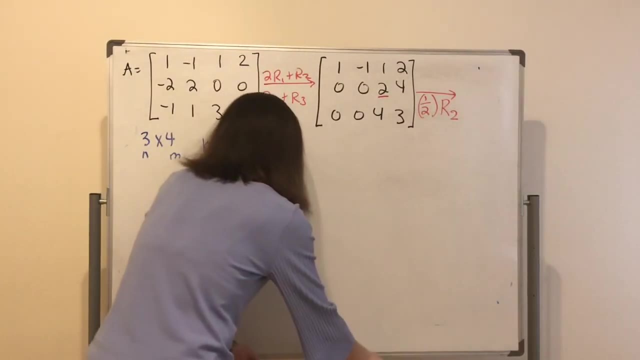 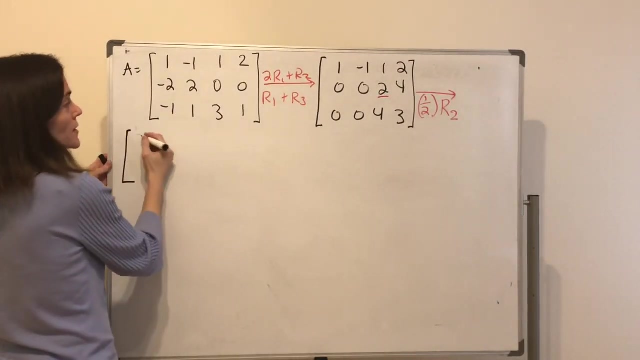 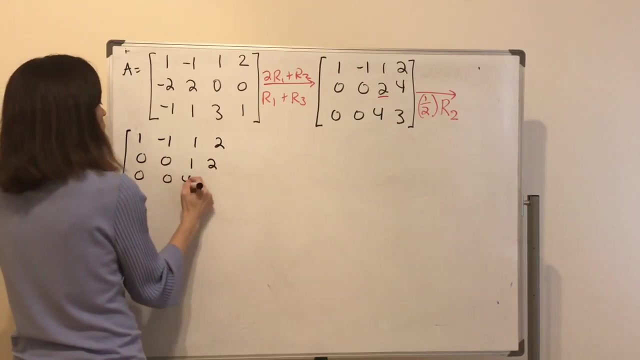 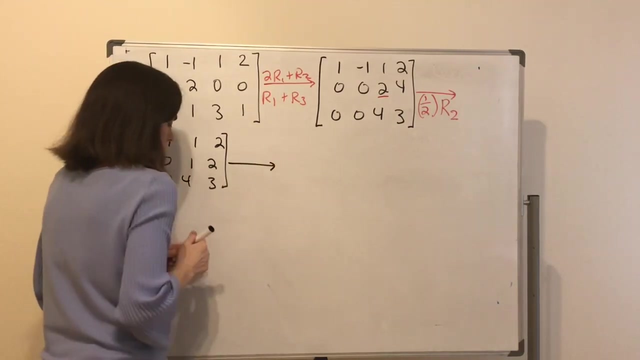 Okay, so I need to make this a 1.. I will take 1 half times row 2.. Let me erase this observation. Try to back up so I can fit more: 0, 0, 1, 2, then 0, 0, 4, 3.. Now I can eliminate this 4.. 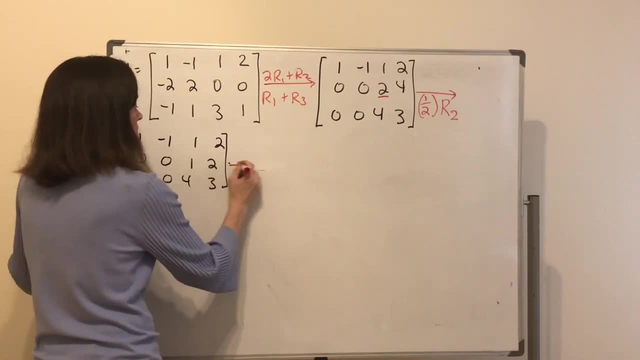 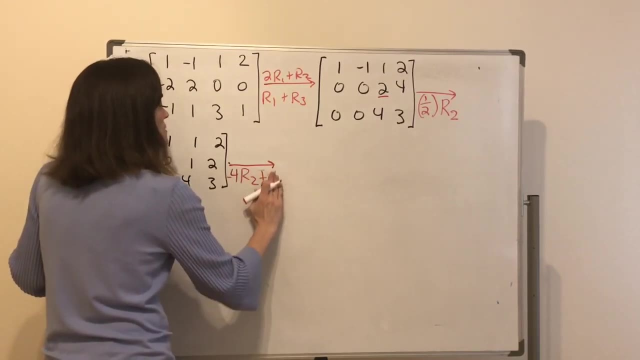 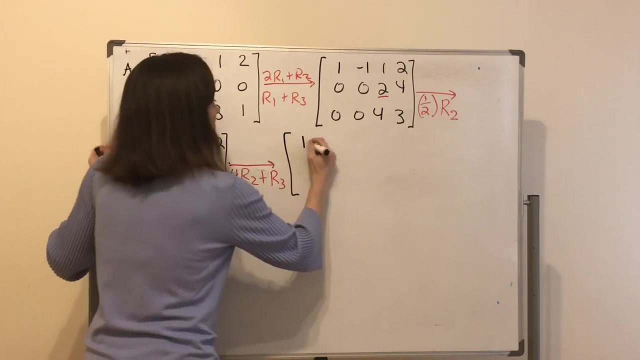 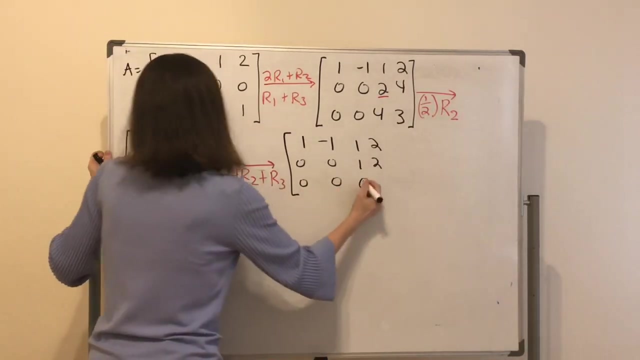 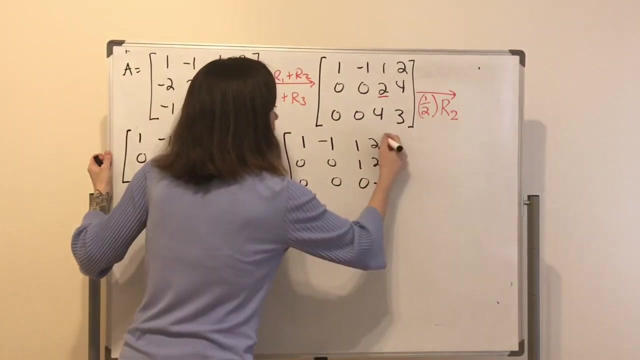 Okay, it should be red. I take 4 row 2, minus 4 row 2, add it to row 3.. Minus 4 would be minus 8.. We get out minus 5.. Very nice, Now I'd like to fit another one here. 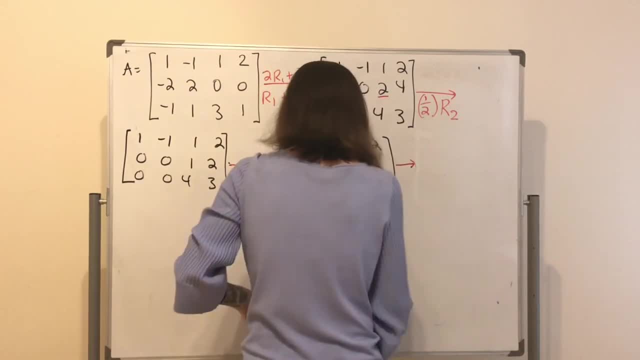 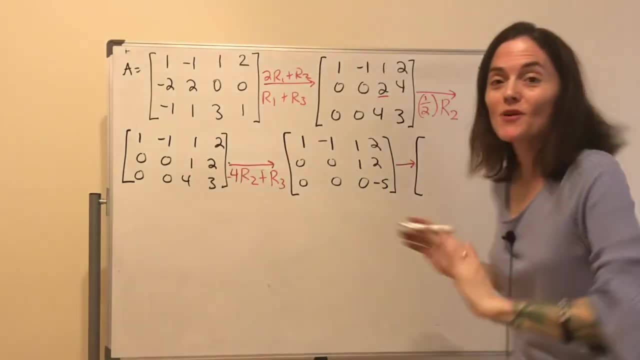 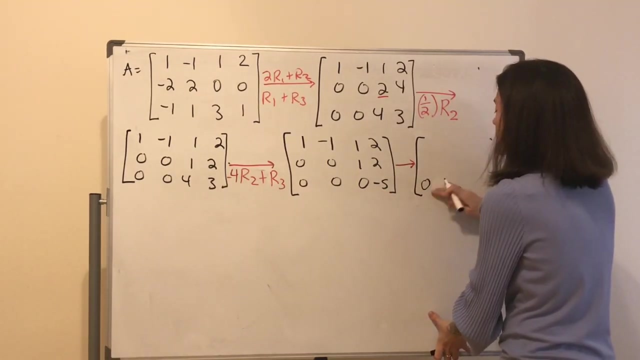 Well, what I'd like to do is I'll fit it. Okay, let me move so we can look at our matrix. I can make this a 1 just by multiplying through by. I'm going to do more than one step in 1.. 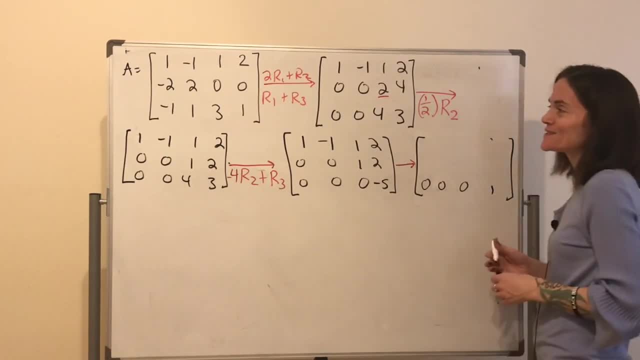 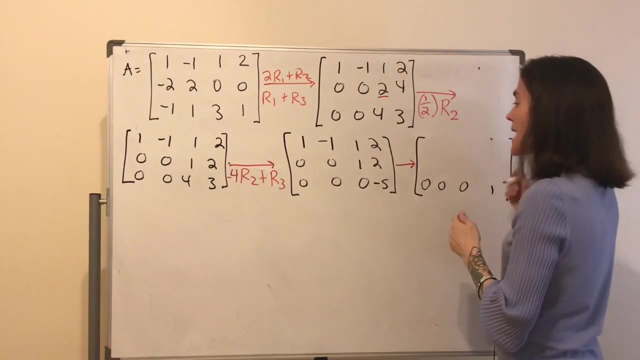 This is not the first matrix we have row reduced. I multiply through by minus 1. fifth, Very nice. Then I can take and take minus 2 times row 3.. Add it here, add it here, Right, And while at the same time. 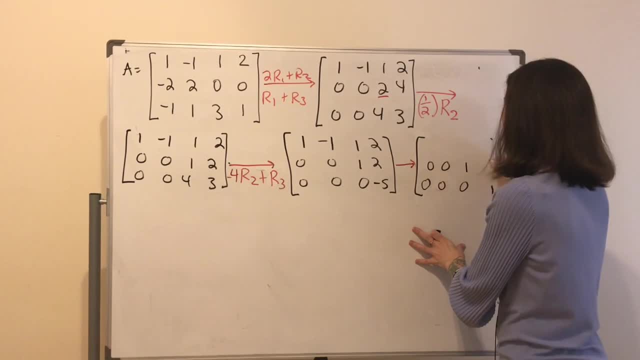 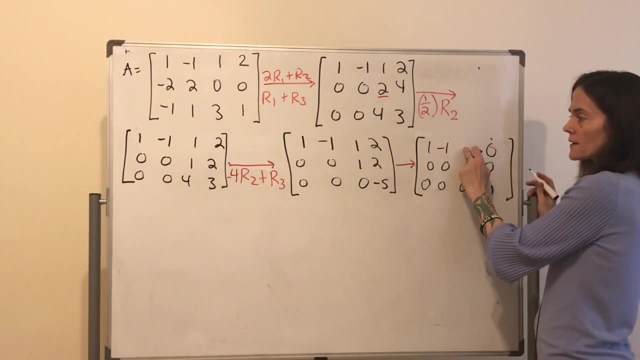 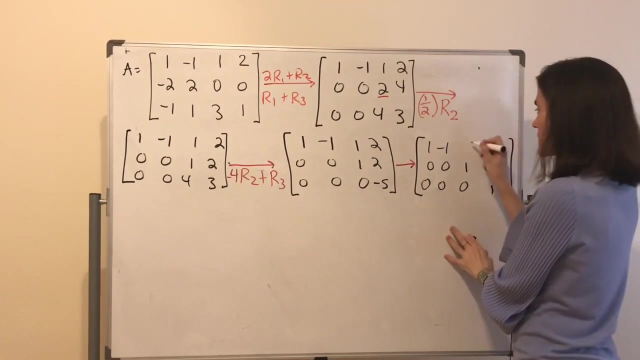 Once I do that, what would I have? I would have this right, And then I would have this with a 1 here. Oh yeah, that's right. And then if I just take minus 1 times this row, add it here, then I would get this. 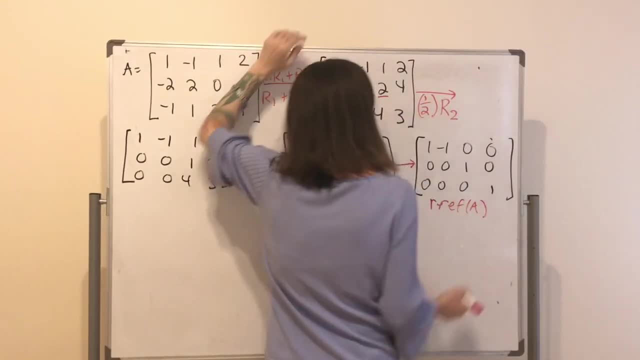 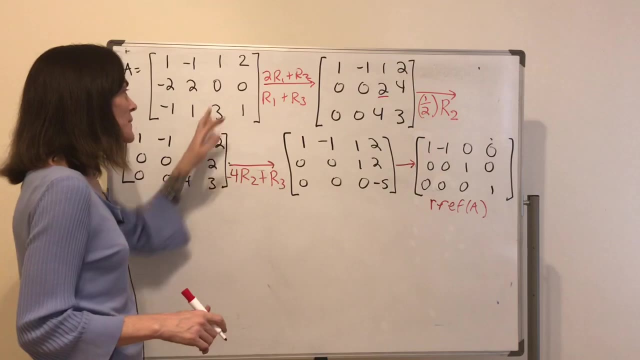 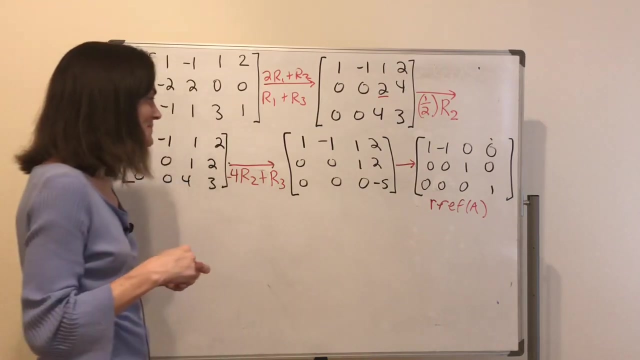 This is our reduced row echelon form. I verbally said what I was doing and then I did it. Okay, Certainly I wouldn't have done that early because I would make mistakes, But once I was down to just working with a few columns, it wasn't too bad. 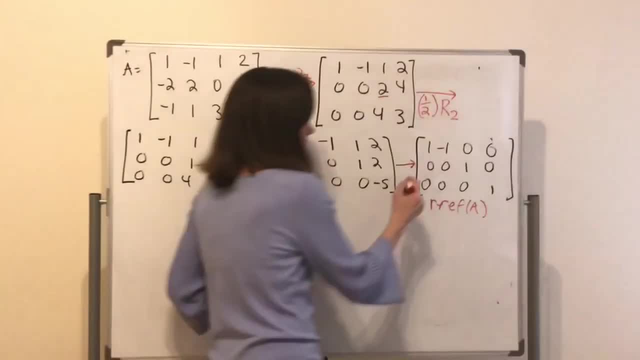 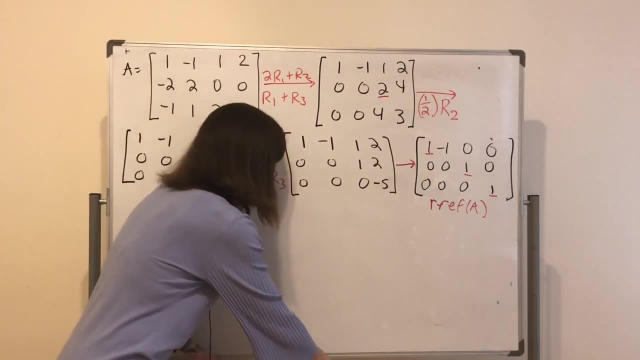 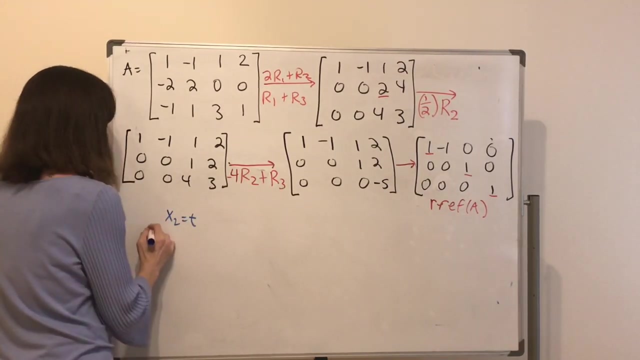 Well, what do we see here? We have leading 1, leading 1, leading 1.. So there's only one free variable, It's x2.. If I let x2 be t and then we get x1 minus x2 is 0. 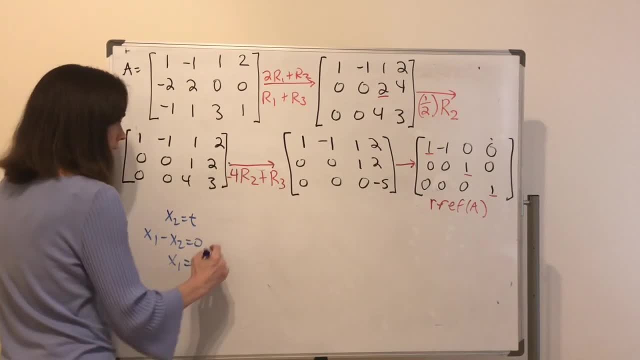 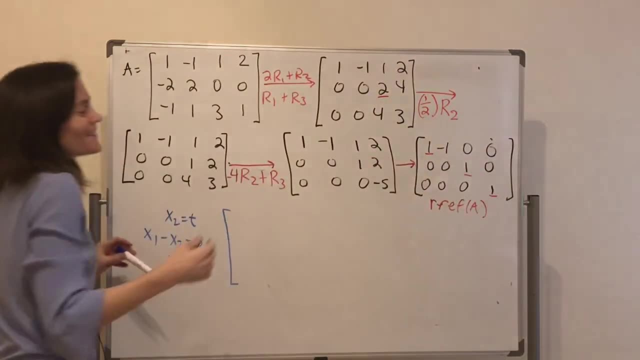 x1.. x1 will also be t, And so my solution to ax equals 0.. Remember, there's 0s over here. Right, I didn't write this down. It didn't augment the matrix, as I mentioned in my last example, but we remember that. 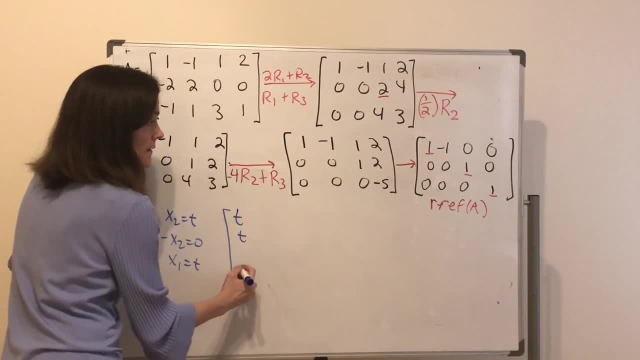 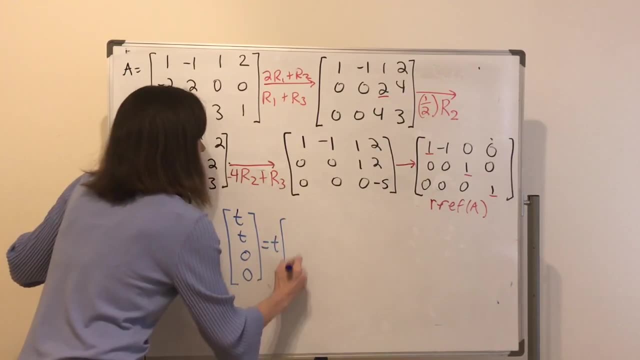 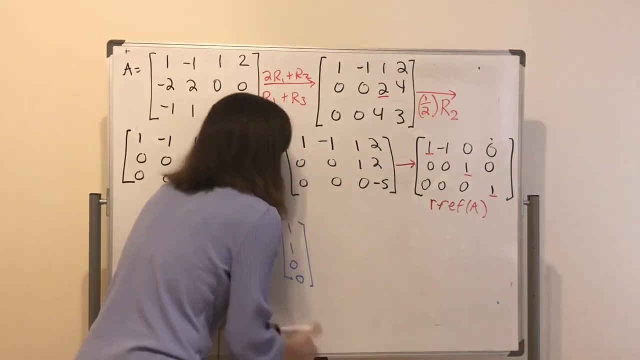 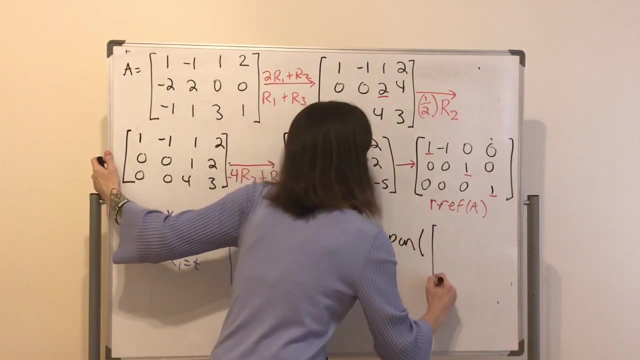 Okay, So I have It's just t, t and then 0, 0.. Which we can write as t 1, 1, 0, 0.. And finally, well, if we solve the problem, the kernel of this matrix is the span of 1, 1, 0, 0.. 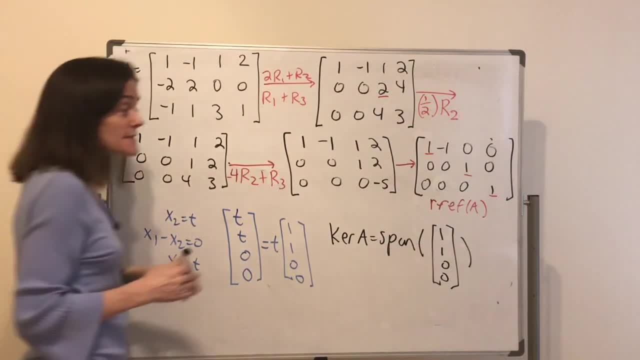 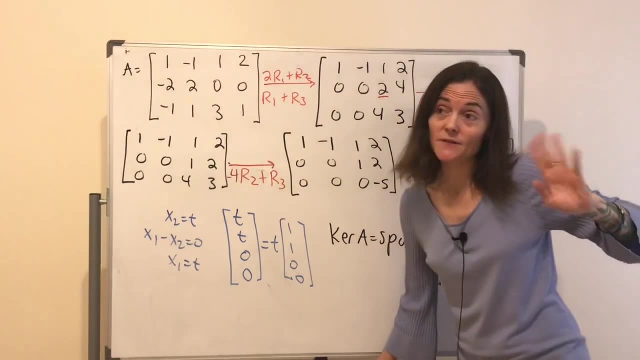 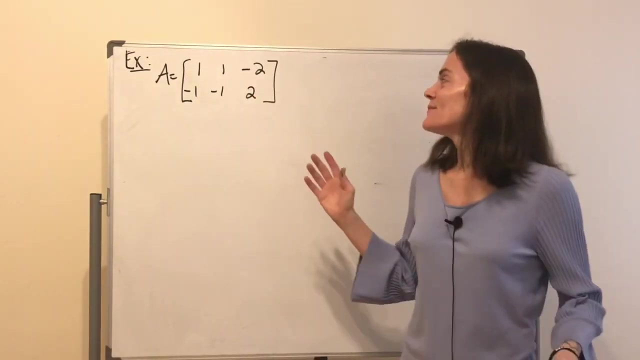 Okay And we get this well. like we saw in both the last two examples, We transform to reduce row echelon form. We did the first day first, second day of class, say: Well, this matrix is not huge and it's also very quick to write in reduced row echelon form. 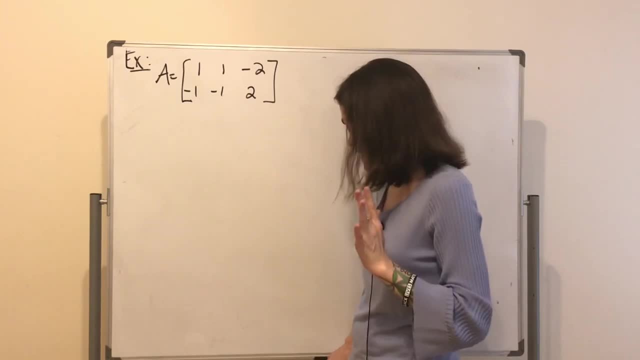 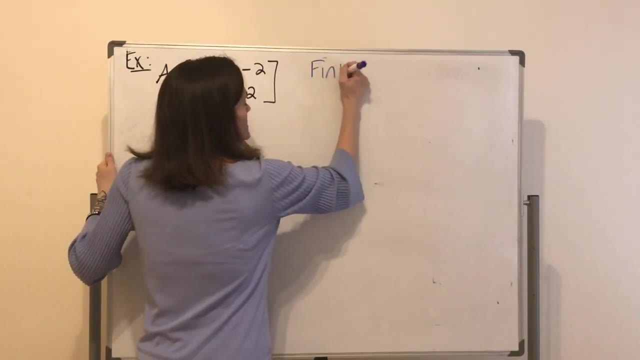 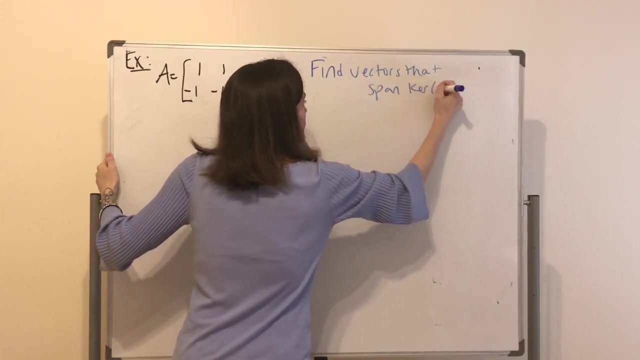 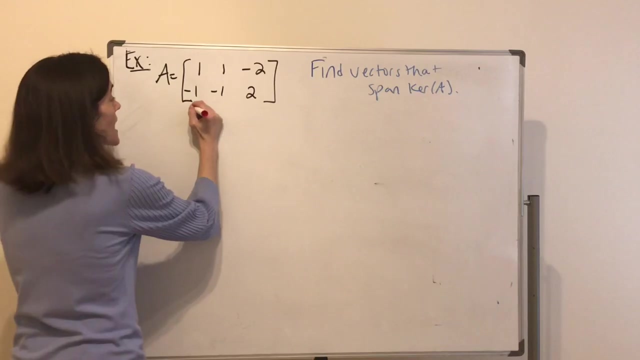 But it's very informative in terms of an example for finding the vectors that span the kernel. I'm still working with the kernel. Maybe I'll write it this time: Find the vectors that span the kernel, The kernel, Okay. Well, maybe I'm going to move down now, because I just wrote where I would naturally move to perform row operations on my matrix. 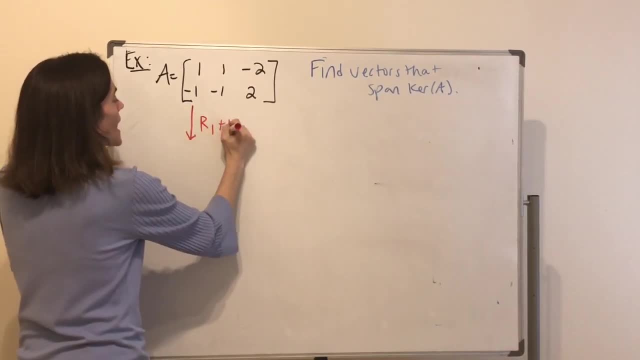 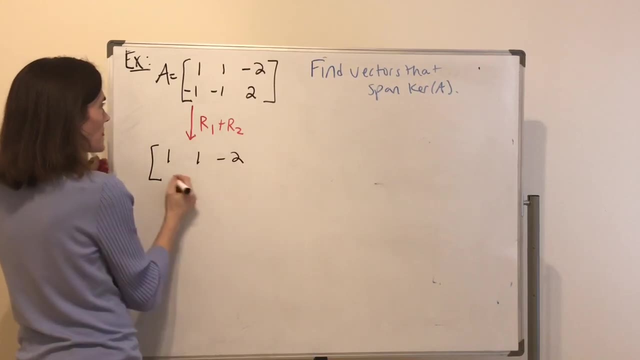 All I need to do is take row 1, add it to row 2, and look what I get. I get 1, 1, minus 2.. I get 0, 0, 0.. You see, This is already reduced row. echelon form. 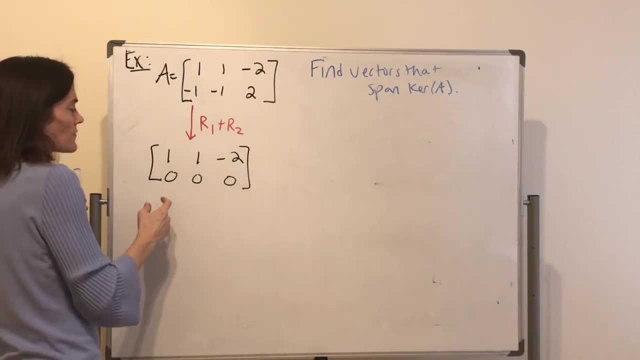 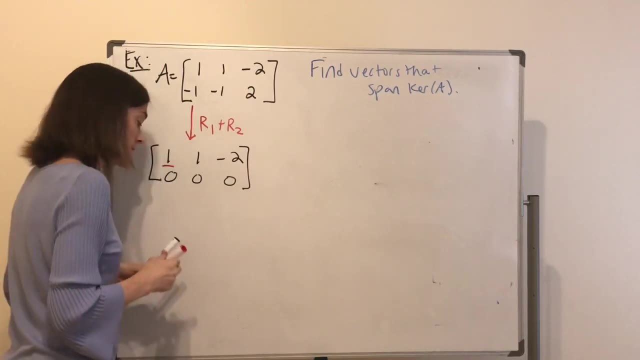 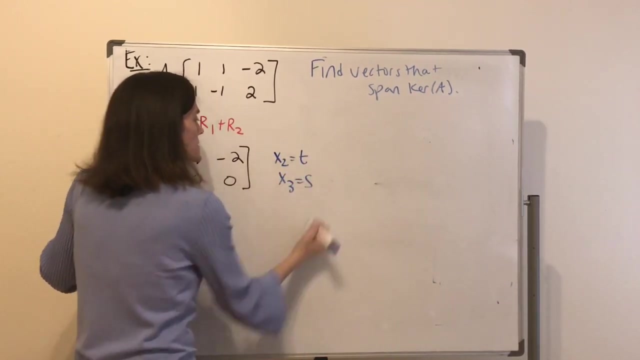 This is one step And we see we have only one leading one. We have one, two free variables, Okay. Well, how are we going to figure out vectors that span the kernel here? X2 and X3, so maybe X2 is T and X3 is S. 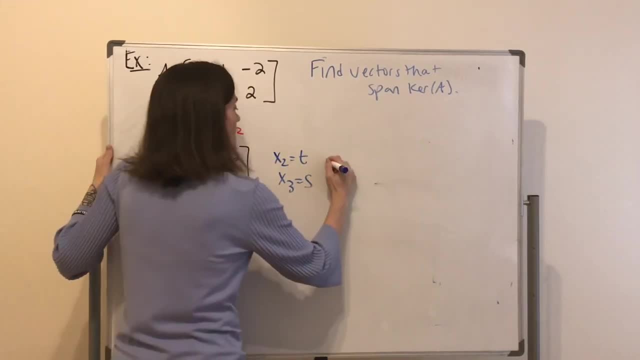 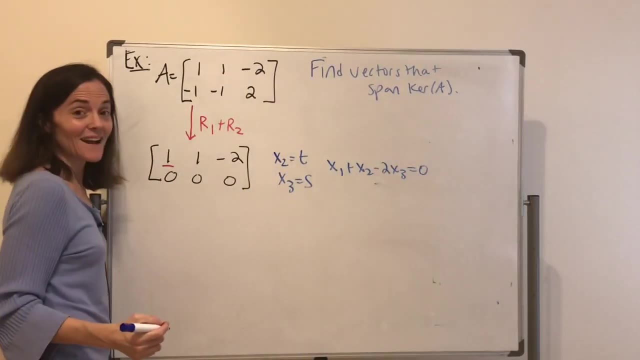 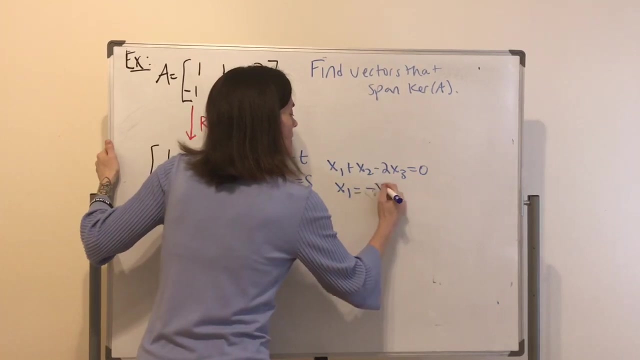 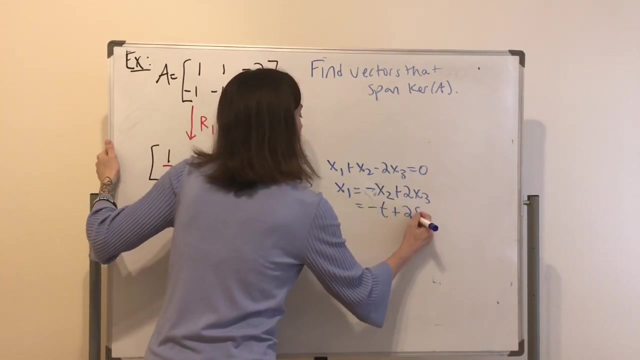 And then there's only one equation here. It says that X1 plus X2 minus 2X3 is 0.. Right, Okay. So then X1 minus X or equals- excuse me, negative X2 plus 2X3,, which is negative T plus 2S. 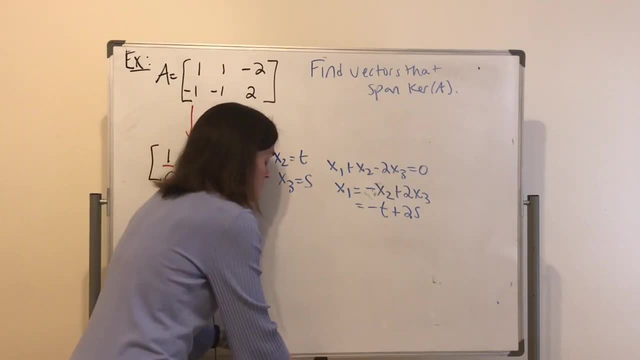 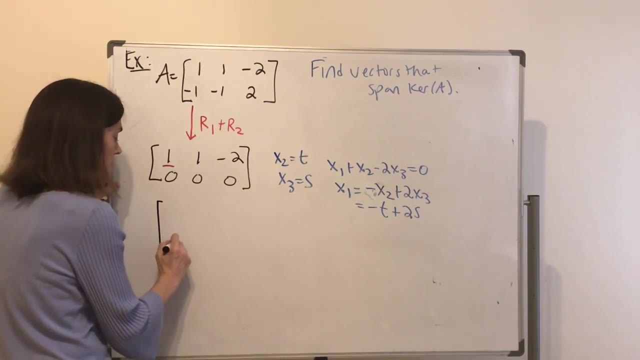 Now let's write the solution. It is okay: X2 is T, X3 is S, X1 is negative, T plus 2S. Well, I'm still not finished. I want to find vectors that span the kernel. We're almost there. 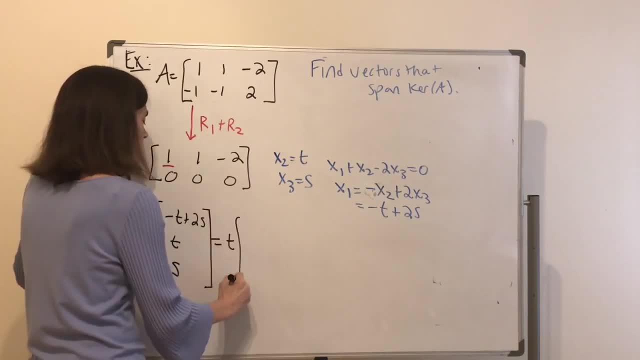 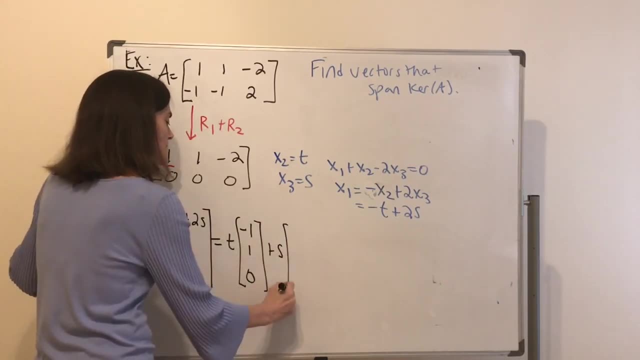 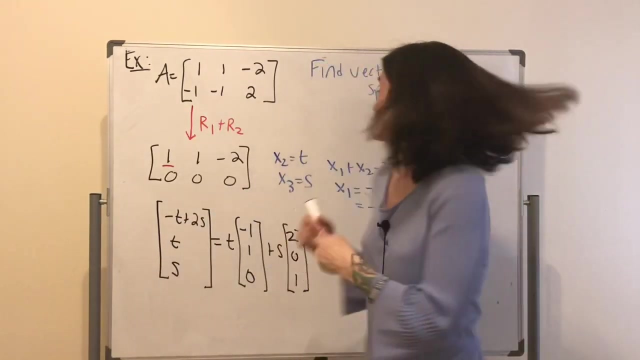 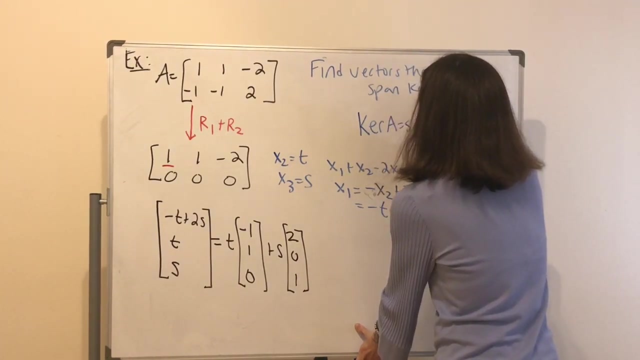 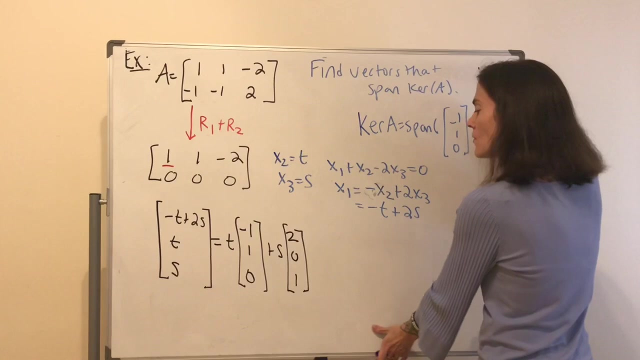 This is T times minus 1, 1, 0. And then S times 2, 0, 1.. These are the two vectors that span the kernel. Okay, Put it up here. The kernel of A is the span minus 1, 1, 0 and 2, 0, 1.. 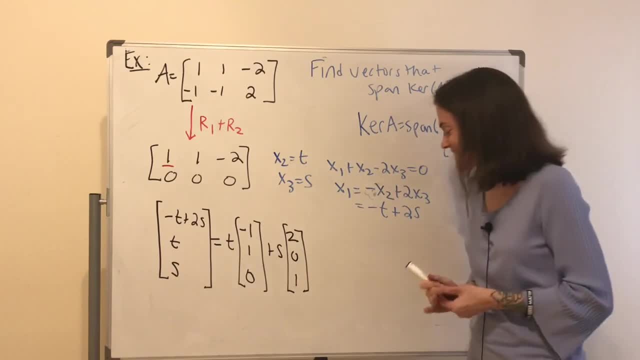 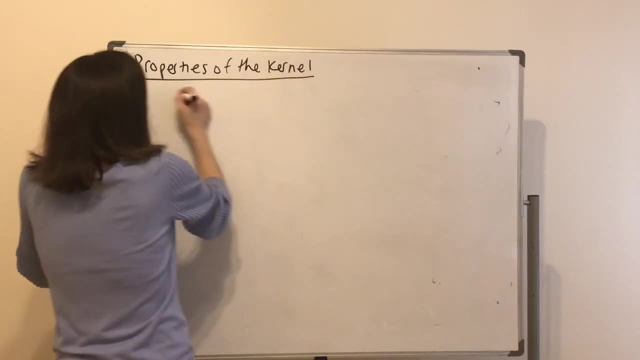 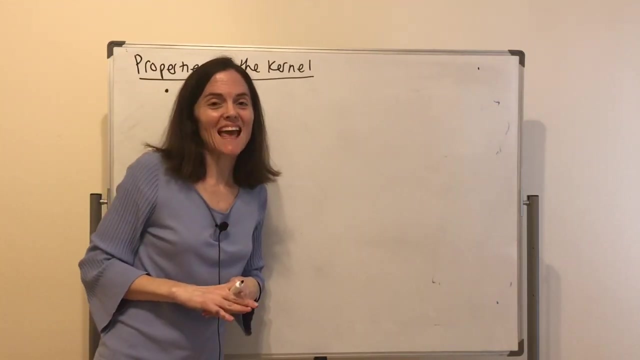 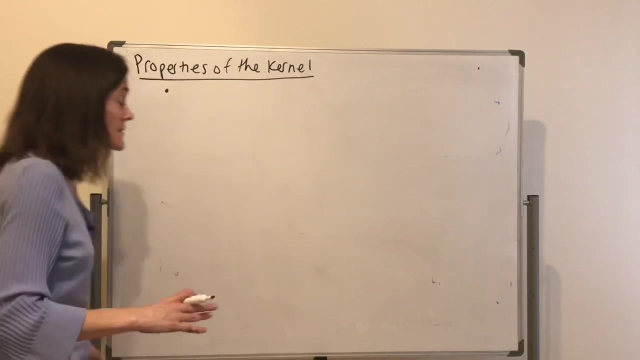 There you go. Okay, Very nice, The first one. Now, this is for any M by M matrix A or, equivalently, for any transformation from RM to RN. Okay, This all holds. The first is that 0 is in the kernel. 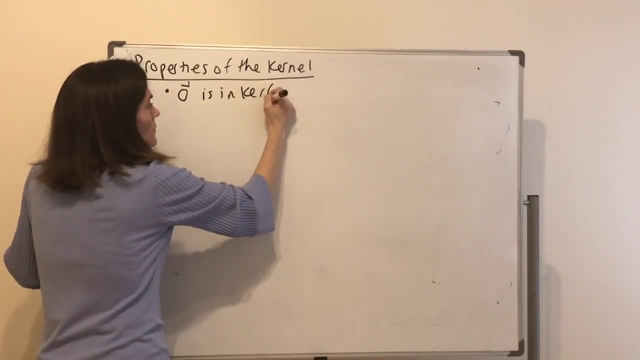 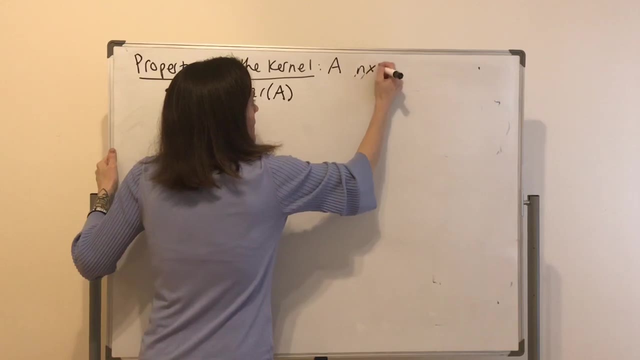 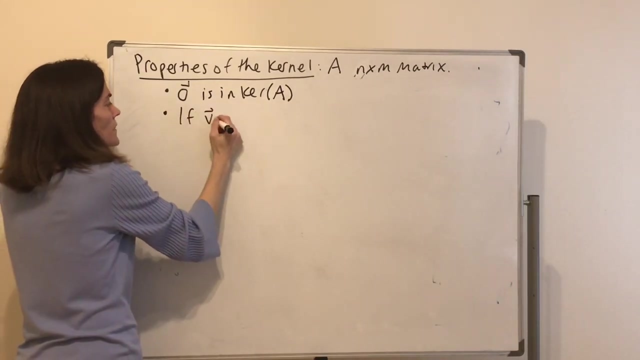 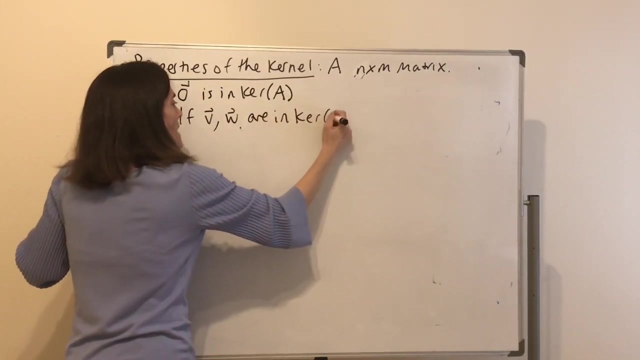 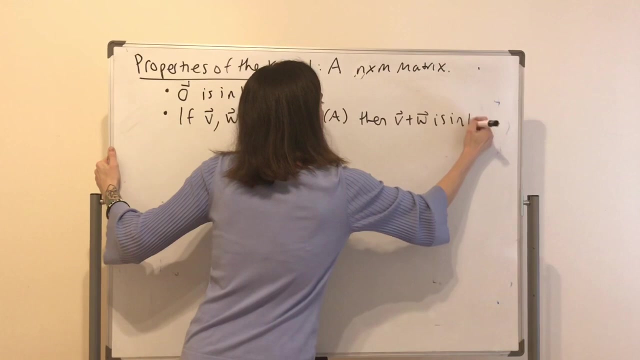 I'll just say for A M N by M matrix: Okay, 0 is in the kernel. If you have V and W are in the kernel, Then the sum is V plus W. V plus W is in the kernel. And finally, I'll give you a little bit of space. 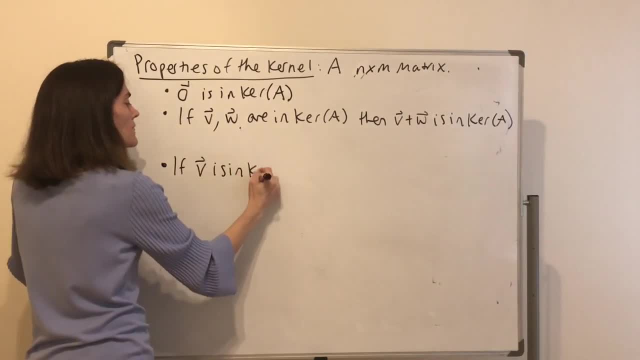 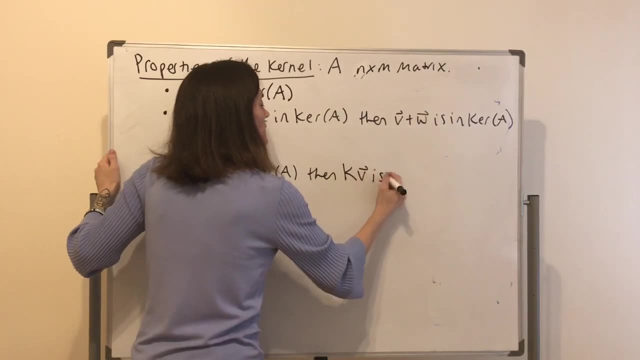 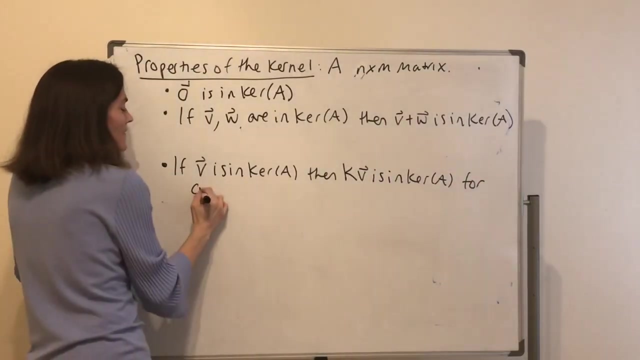 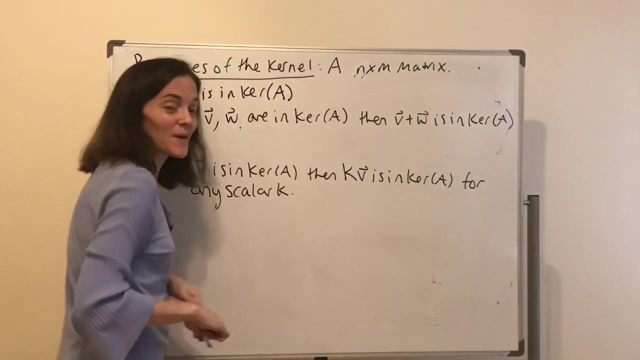 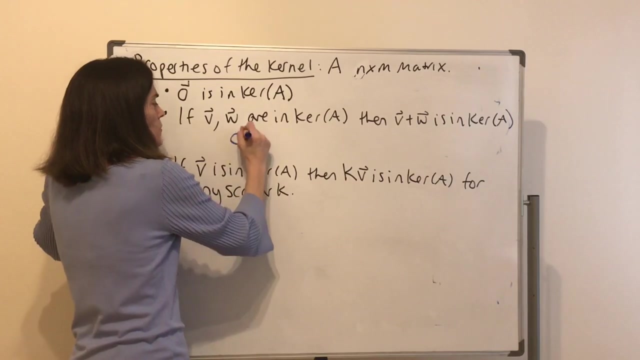 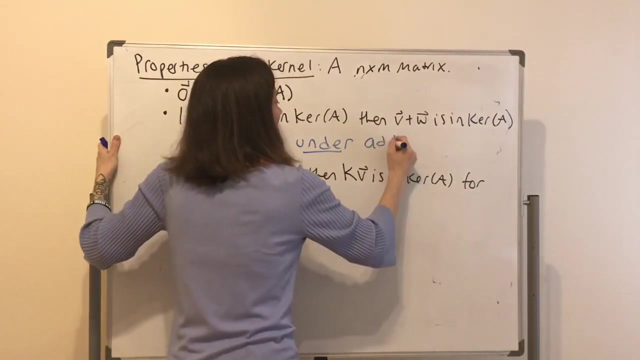 If V is in the kernel, then KV is in the kernel for any scalar. Okay, Okay, Okay. Well, these are very important. This has a name. The first one it says is what's called closed under addition. This is vector addition, of course. 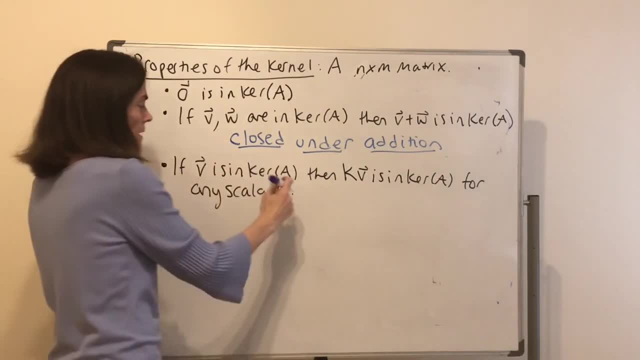 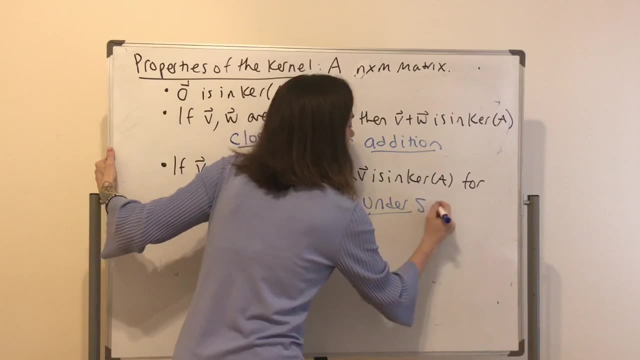 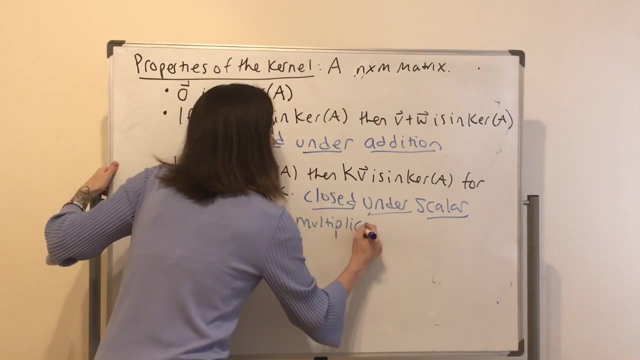 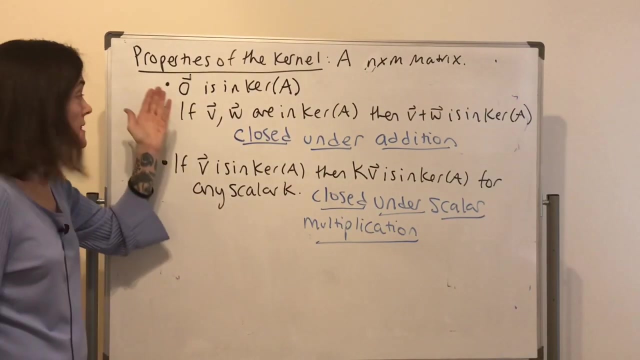 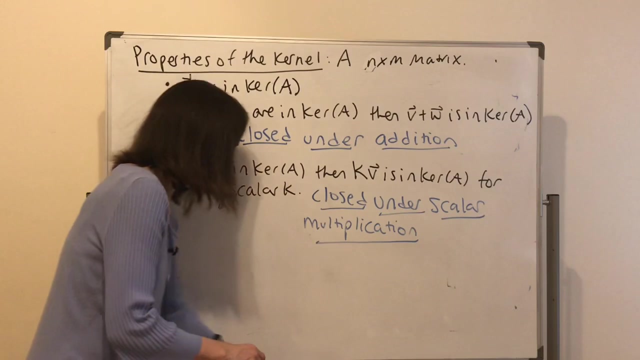 And this one is called closed And that one is closed under addition. Okay, this one is called closed under scalar multiplication. When you have these three properties, that zero is in, let's say. I'm going to talk about subset now, because we know, let's say it. 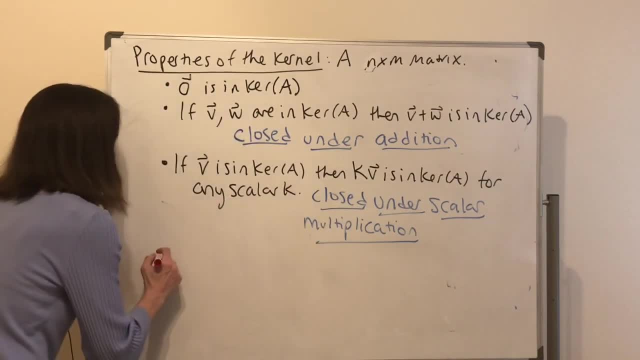 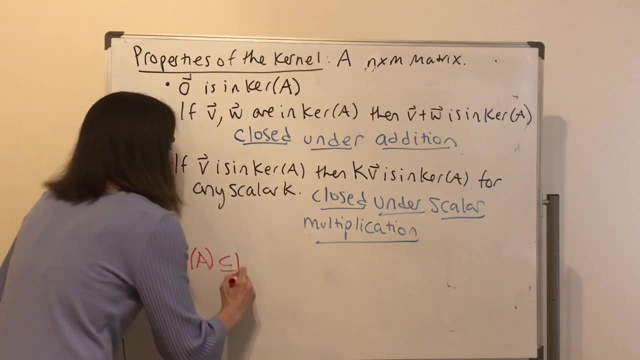 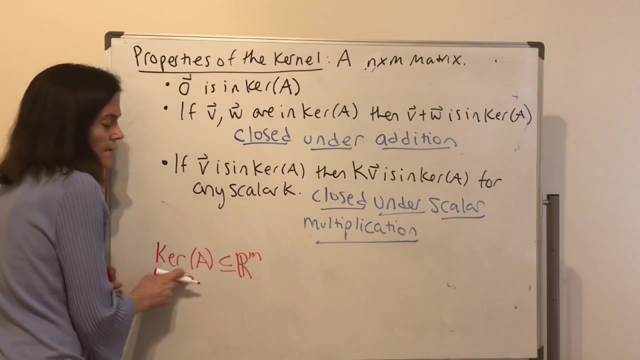 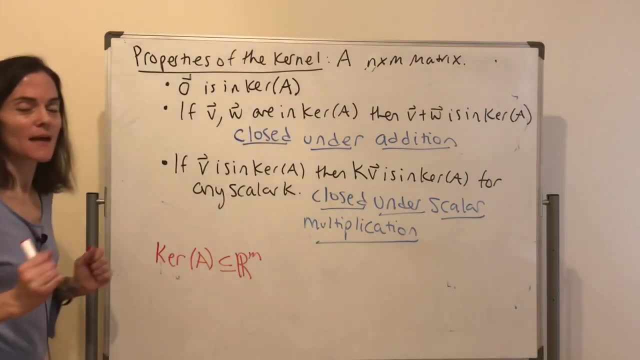 again, we know- what do we know so far- that the kernel of A is the subset of Rm, just meaning that this consists of some elements in Rm. there are vectors in Rm that are in here. okay, but any time you have a subset of some R to the m or R to the n, okay that. 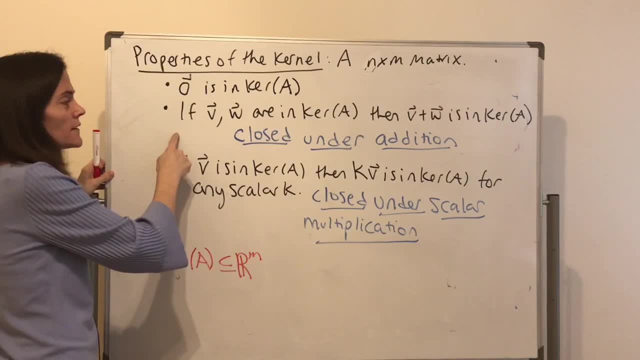 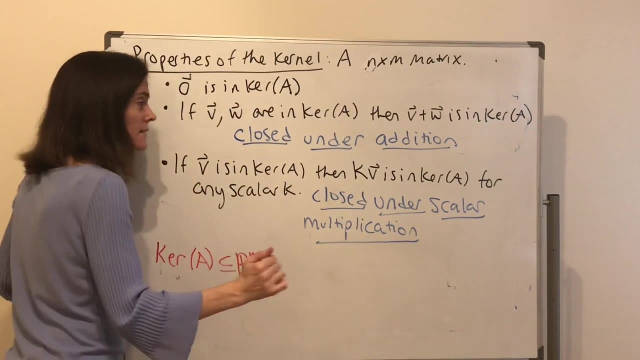 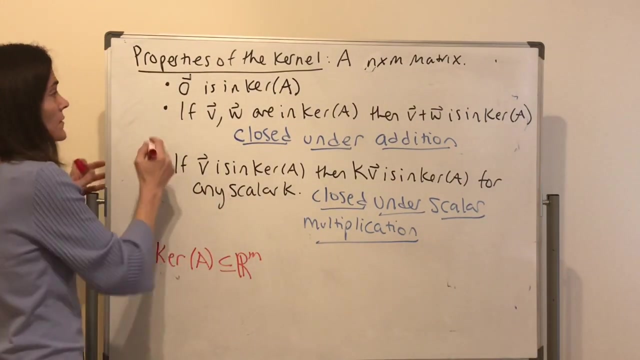 satisfies zero is in the set. if two vectors are in the set, then the sum is in the set, and if you have a vector in the set, then k times the vector is in the set for any scalar k. These three things together give you what's called a subspace. 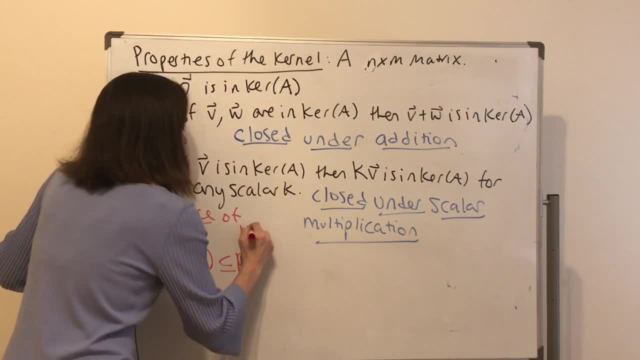 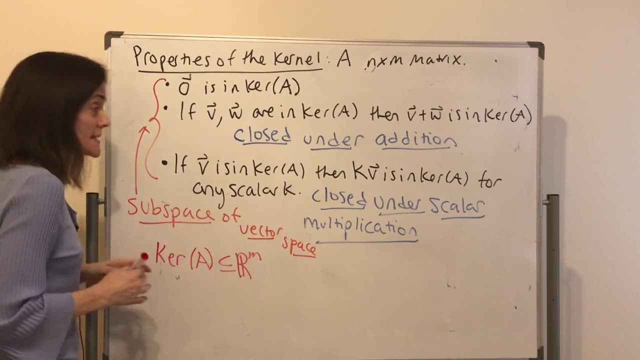 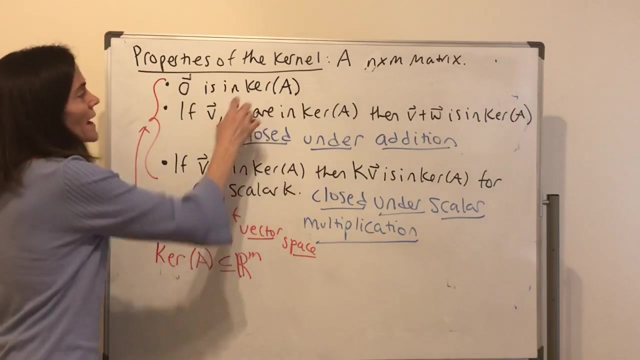 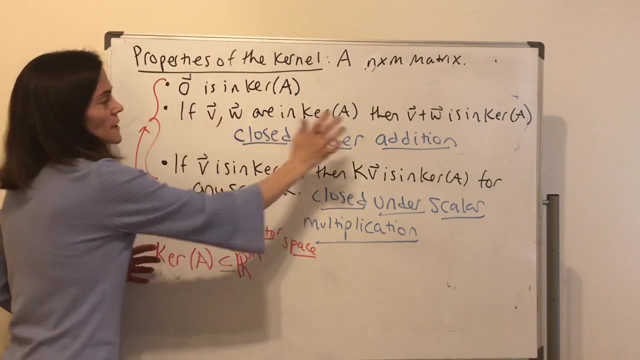 space? well, a vector space generally. and so what this says? these three properties which are not even hard to show. I was going to do it, but let's talk about it. Why is zero in the kernel? Well, because any matrix times zero is zero. Why, if you have two things? 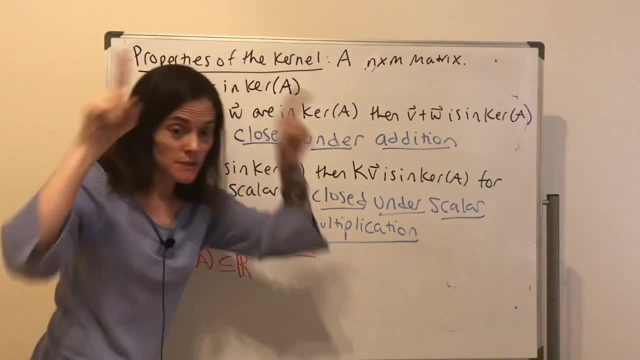 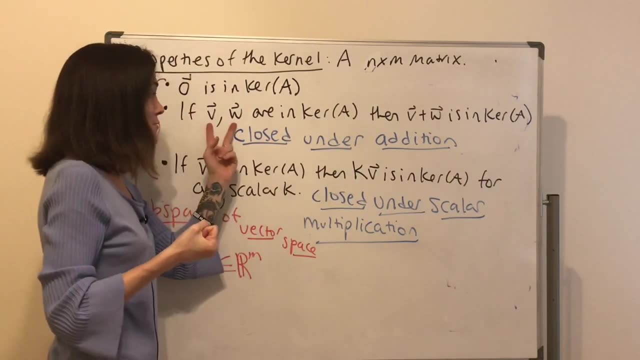 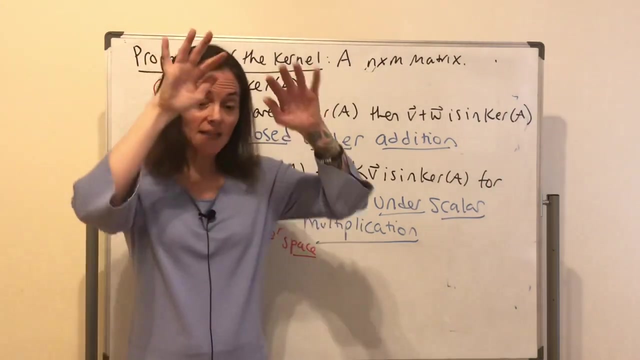 in the kernel. why is there some? Well, it's because A times V plus W Is A V plus A W, and this zero, this zero. so if these two are in the kernel, so is the sum. and then why is k? V in the kernel when V is well, A times k V is k A V, and 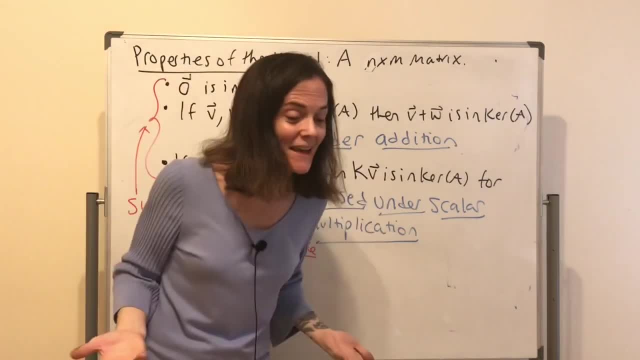 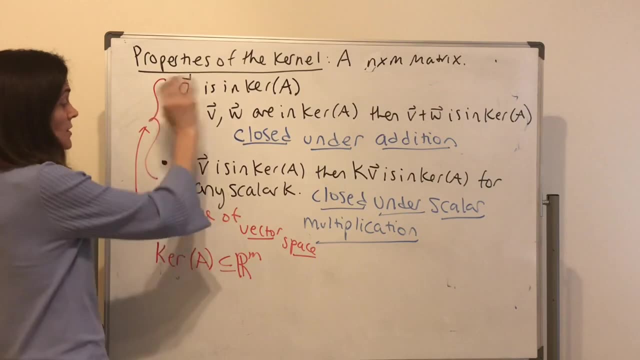 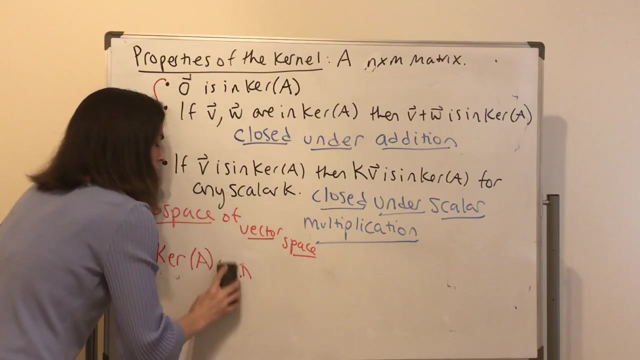 if this is zero, k times zero is zero, so it's very quick to write down the proof of these things. but what this is saying is that the kernel is a subspace Of Rm, so now let's change it. This is much stronger than just a subset. The kernel of 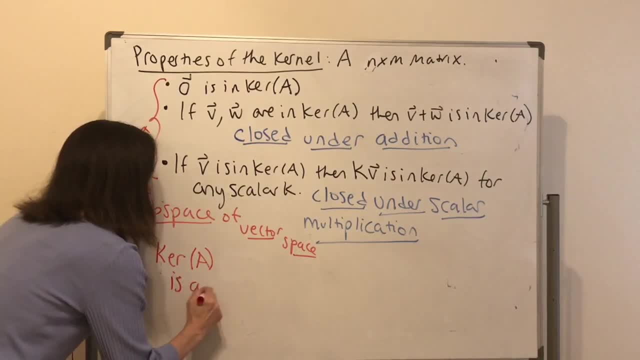 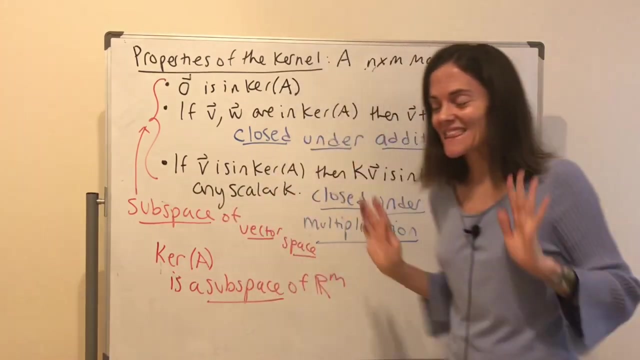 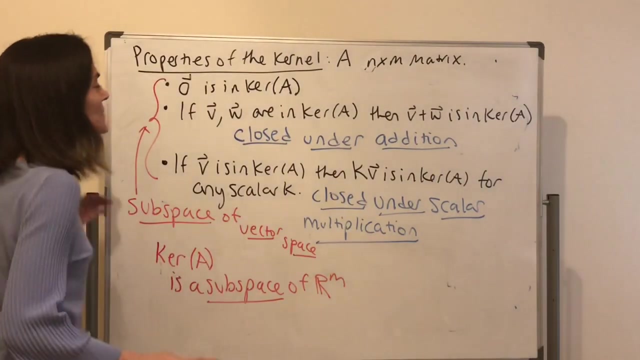 A is a subspace of Rm and we are going to get into subspaces, bases, things like this, in the very next section, but this is really the first subspace. Well, the first time I've mentioned this. what is a subspace? It's these three properties. 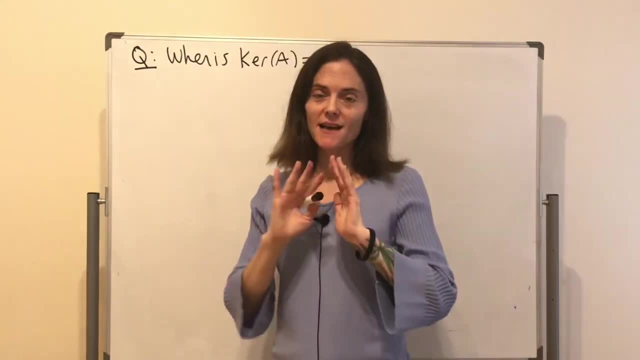 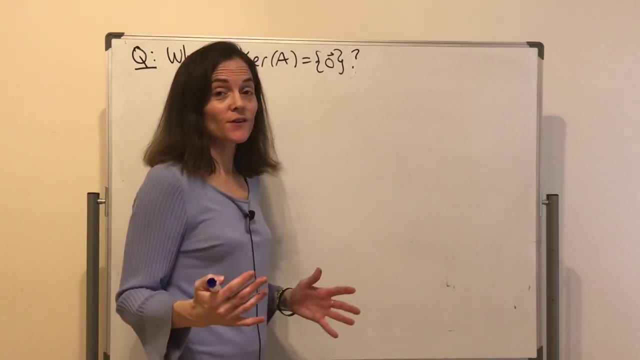 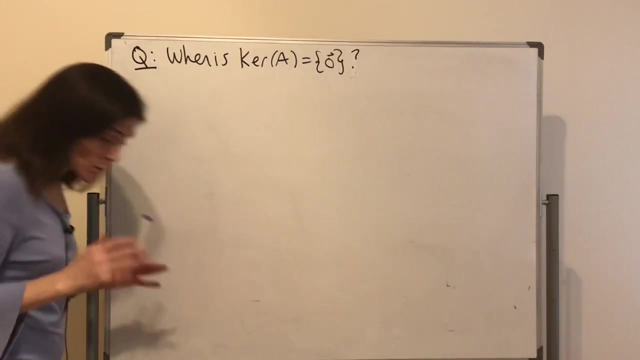 Now I'm going to discuss this question and then we will discuss the image. Okay, the question is the following: When is the kernel of A or the kernel of a transformation? when is this zero? So it's only zero, Okay, well, let's think about this. This occurs. 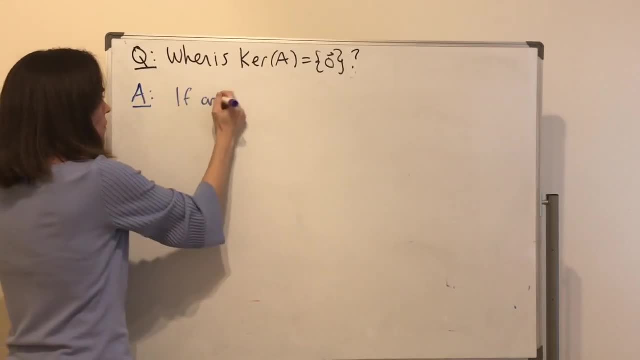 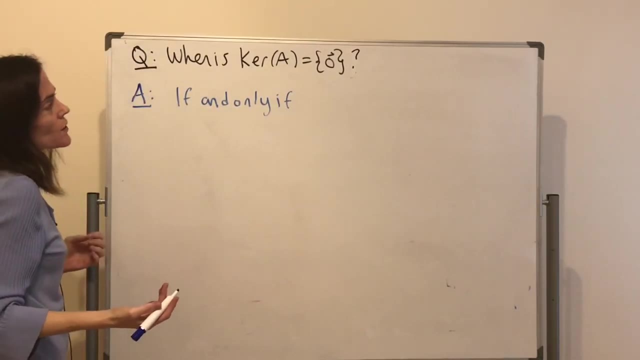 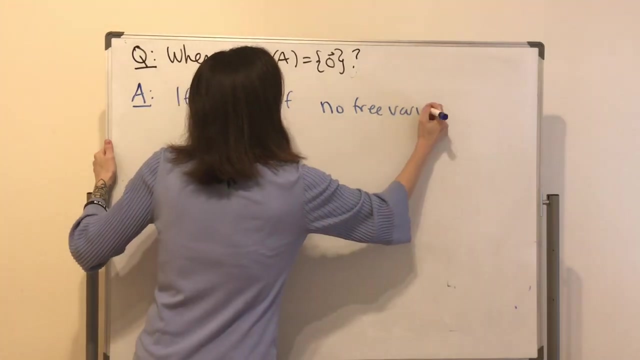 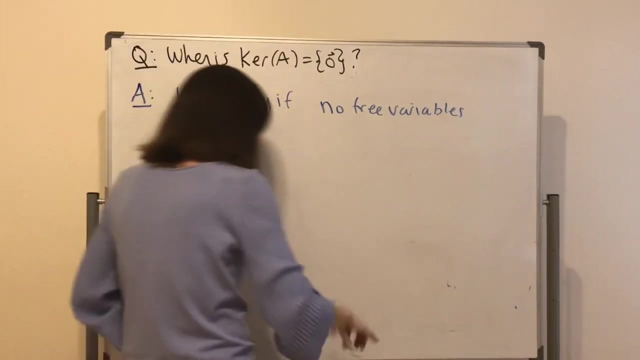 and the answer is if and only if. so let's just start unraveling some things that we observed. Well, the kernel of zero would be if, and only if, you have no free variables in your matrix. Okay, oh, I should say, let me add, let me add A. here is n by m. Okay, 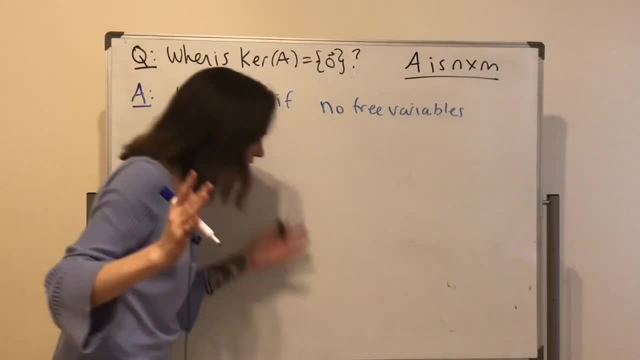 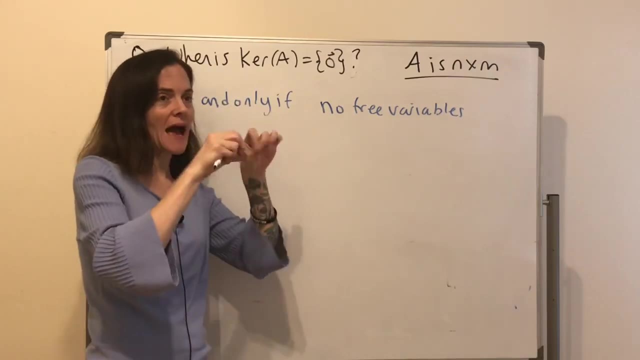 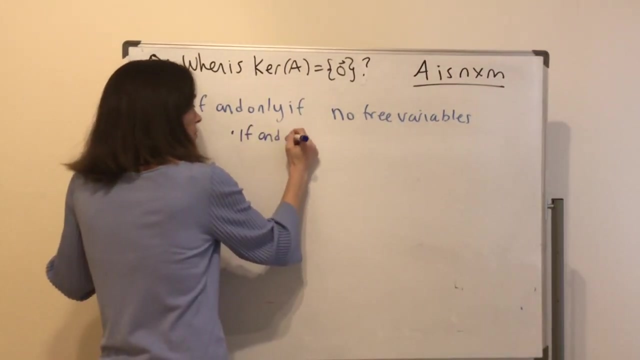 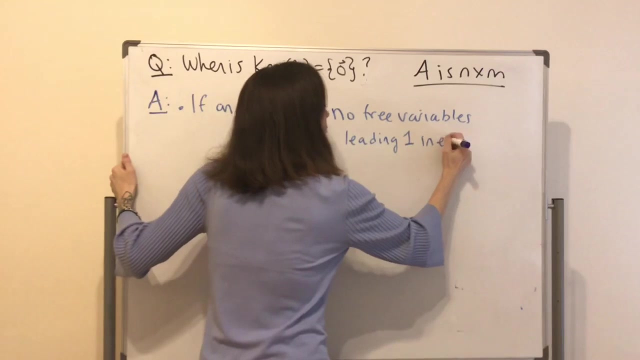 then I can think better. You have no free variables in your matrix because, well, as we saw on the examples, when you have the free variables is when you have, when you are able to find something in the kernel, if, and only if, there is a leading one in every column of the reduced 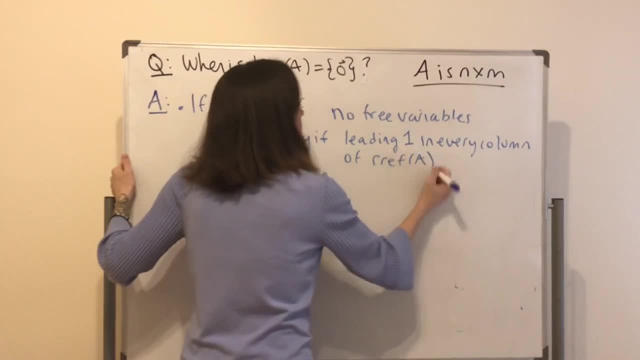 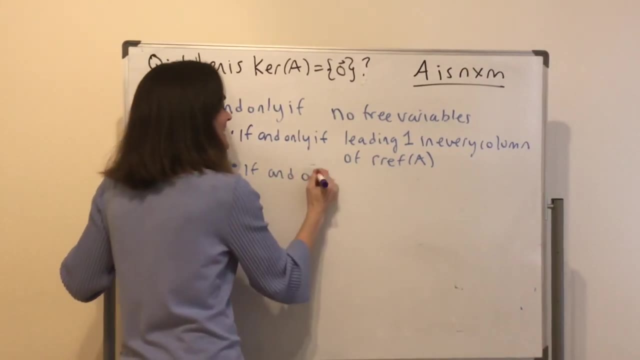 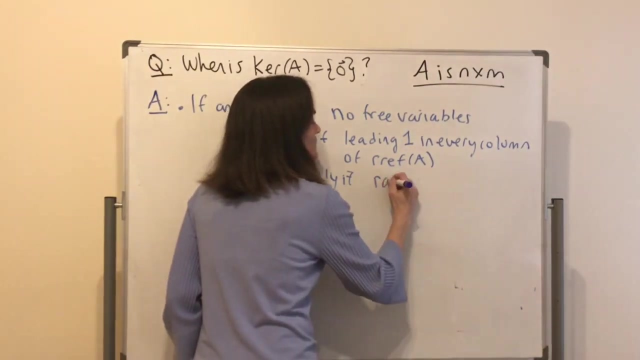 okay, row echelon. form of A. okay, this happens if, and only if, if and- ah, I left out my only only if. if you have a leading one in every column, this says that the rank of the matrix is going to be the number of columns M. 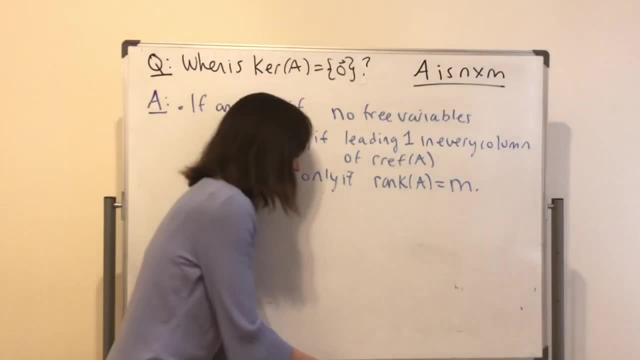 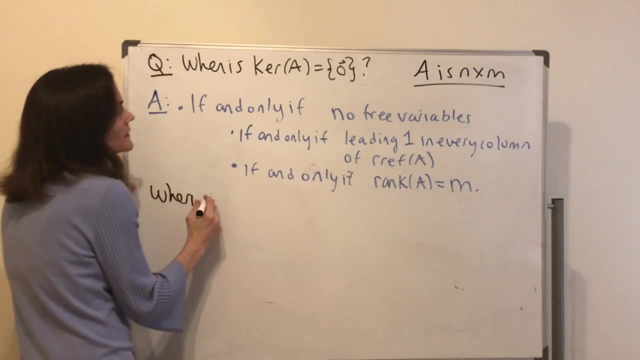 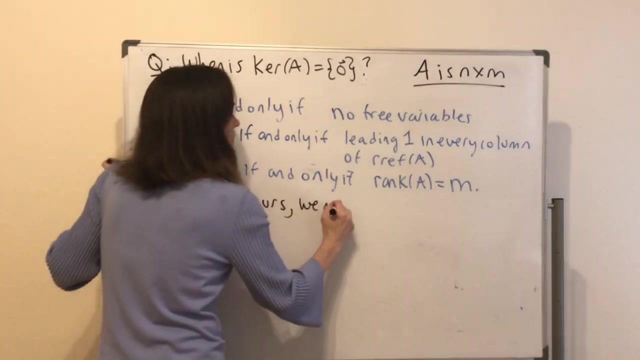 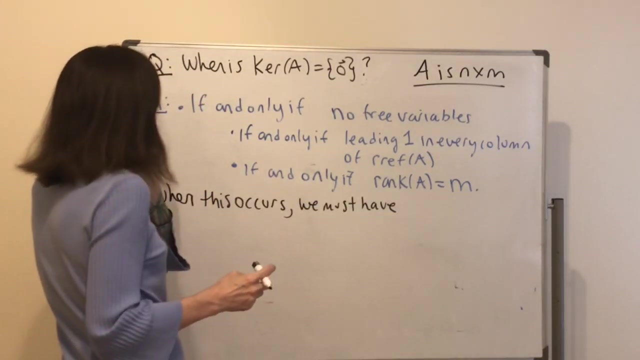 Um, now notice when this much so this is the end of my. I don't even have a string, but when this occurs, maybe I'll do this in black. when this occurs, we must have. well, let's see if you have um. 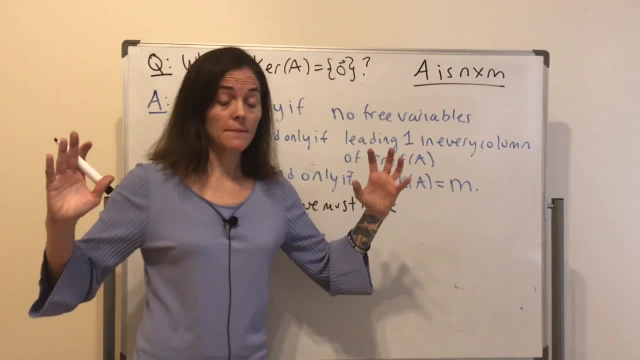 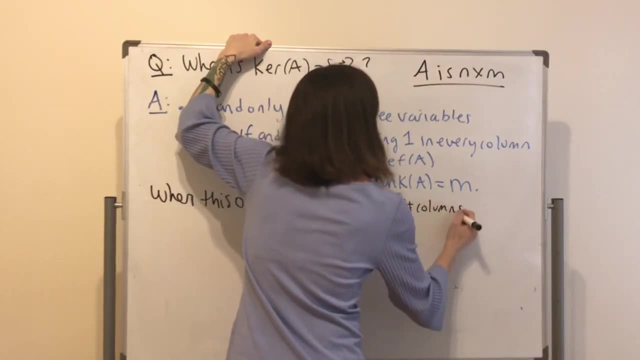 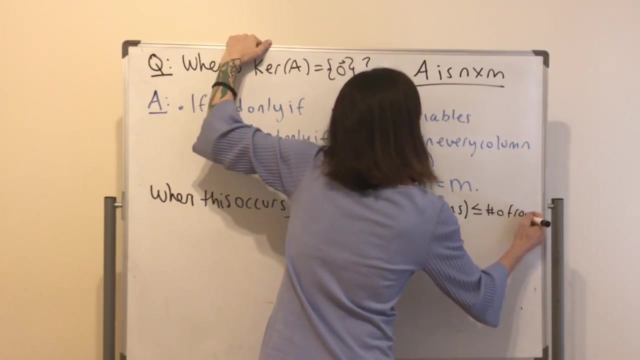 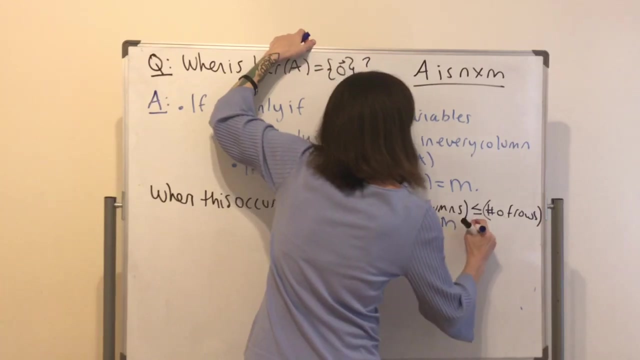 leading one in every column. If you have a leading one in every column, that means you have to have at least that many rows. so the number of columns must be less than or equal to the number of rows. Now if I translate that, this would say M less than or equal to N. but if I tried to remember it like that, it would mess me up, because I interchange M and N in my head. 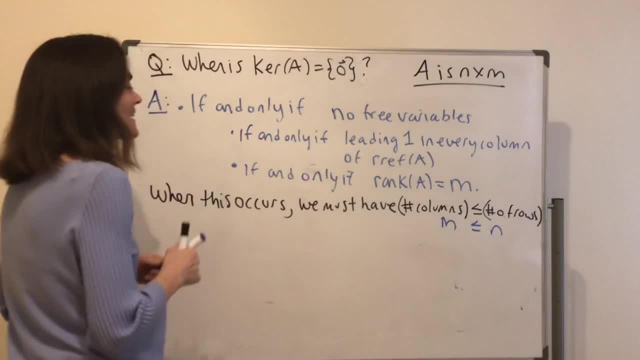 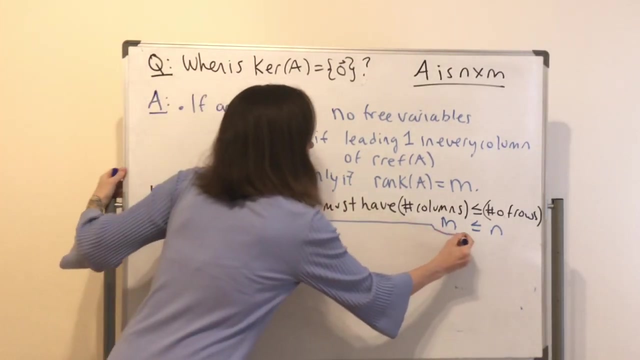 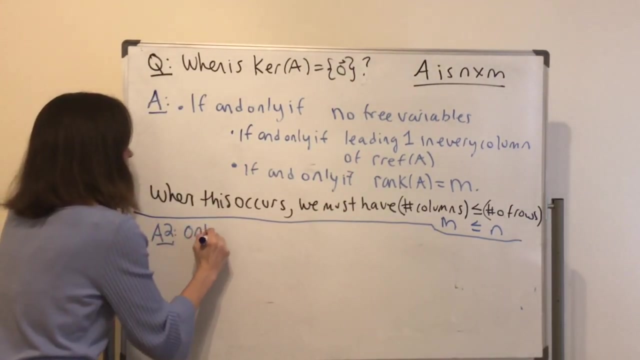 So I just thought about it as columns and rows. Okay, so this is all a very interesting answer to the question, but I'm going to have a second answer. Answer two: this is only for square Square, And I am. 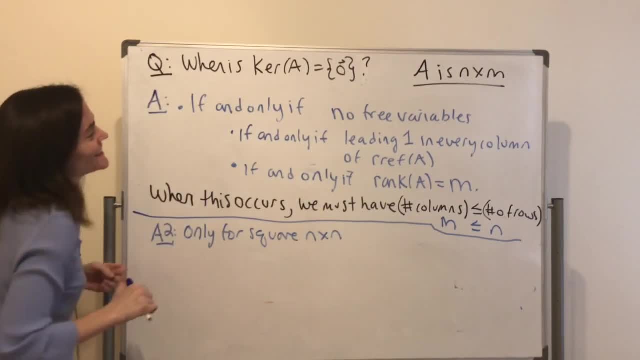 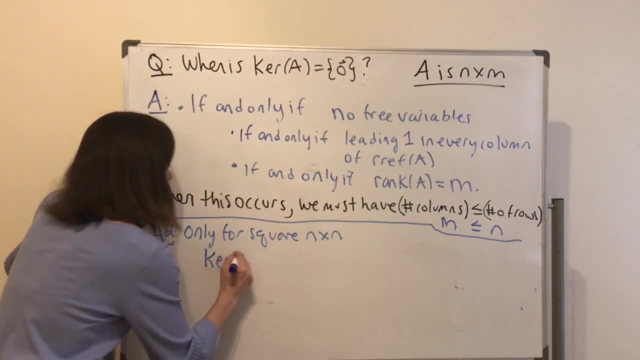 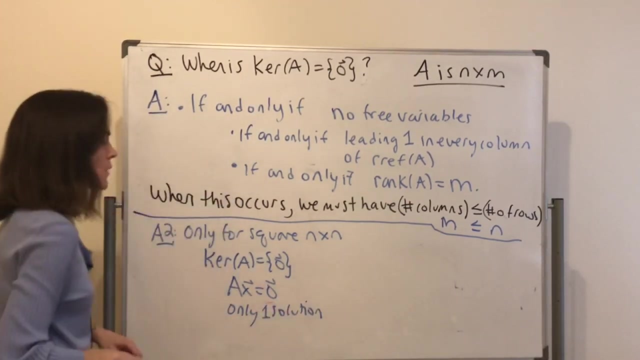 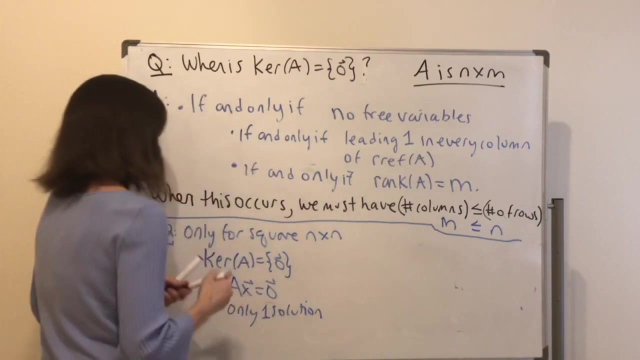 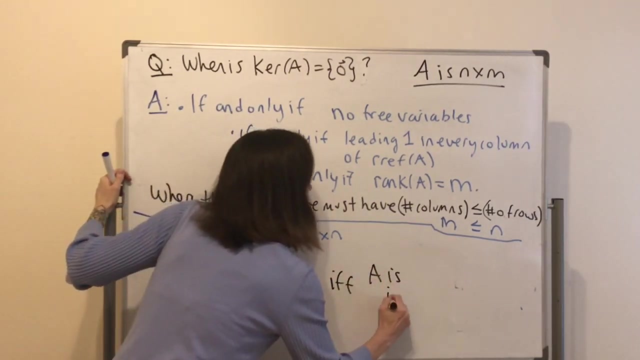 Okay, and then, well, we see the kernel of A equals zero. this is actually something we discussed. this was one of the things. well, right, that AX equals zero has only one solution, Which is the zero solution. and we can even look up here: if, and only if, the rank is all of well. N in this case is full rank, and this says this would be if, and only if, A is convertible. 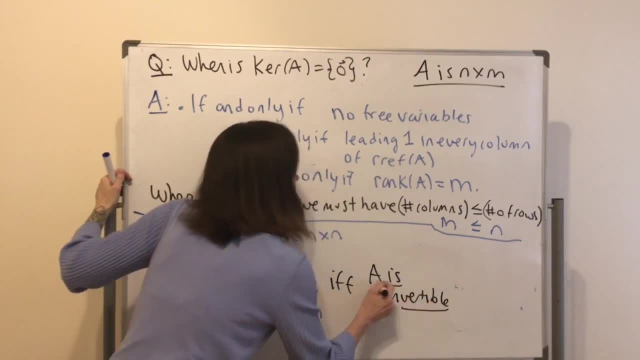 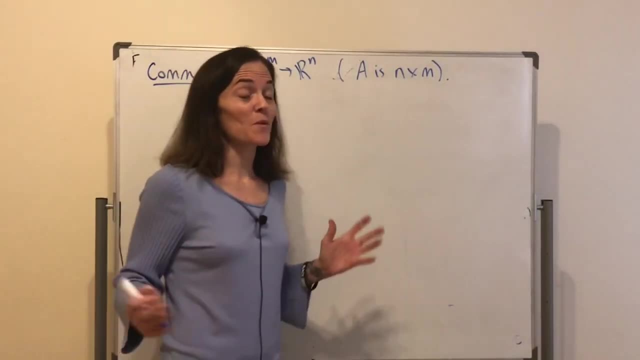 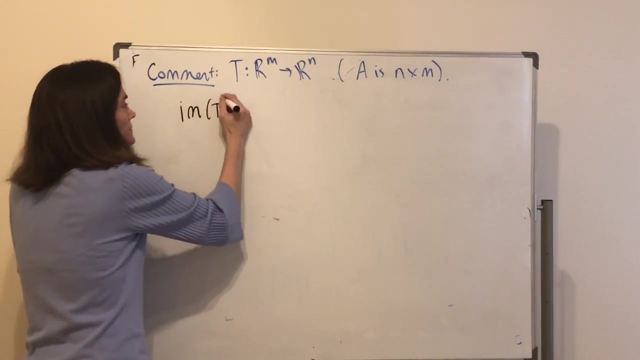 Okay, so this is a full rank. This is a full rank. Let's go here. Let's go here, make one comment before we do anything else, And this is something we're really going to spend more time on next time. But I wanted to just mention that the image of T is a subspace. 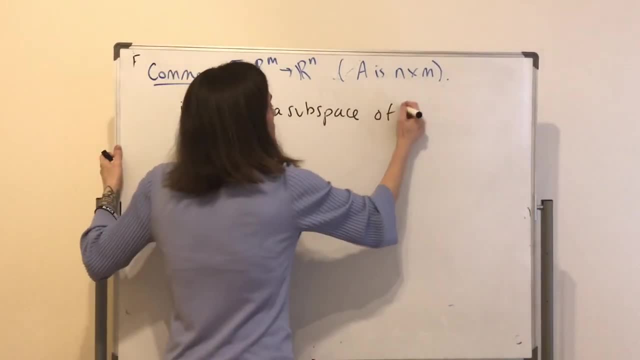 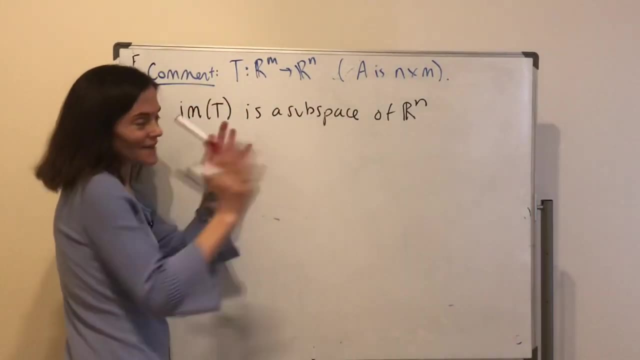 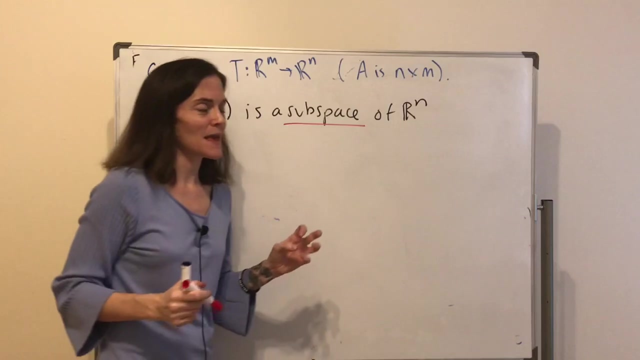 of Rn, So I spent a little bit of time discussing the kernel of T or of A being a subspace of this space, Rm, and this is a subspace of Rm, meaning 0 is in the image. The image is: 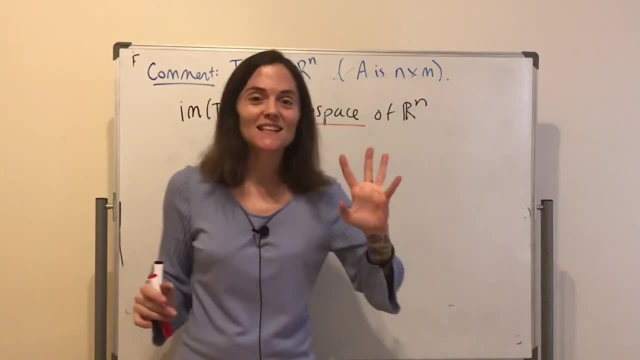 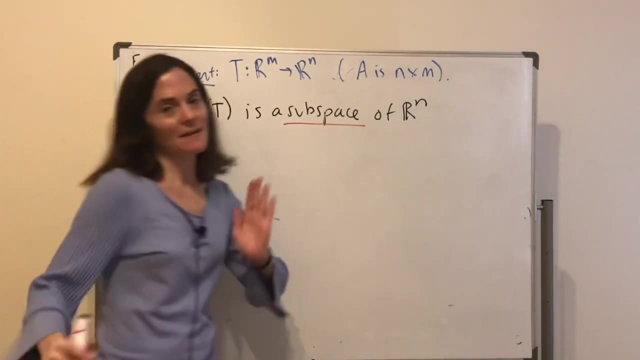 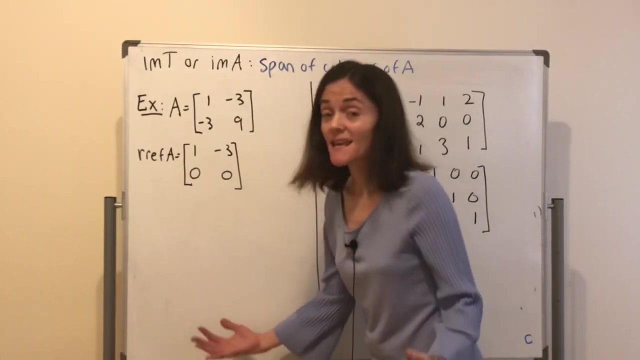 closed under scalar multiplication and it's closed under addition And this type of thing. we will see more next time, but I wanted to make this observation, or at least make the comment today, when we first talk about the image, Now let's do the image or discuss the. 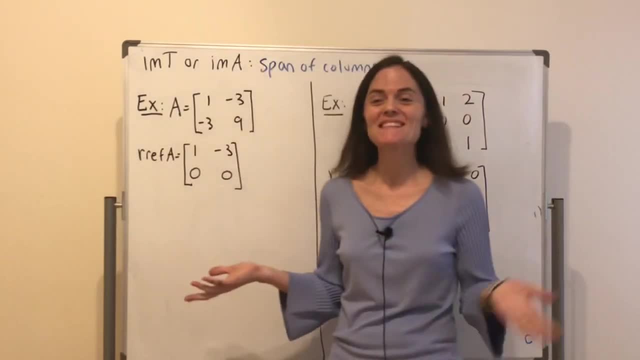 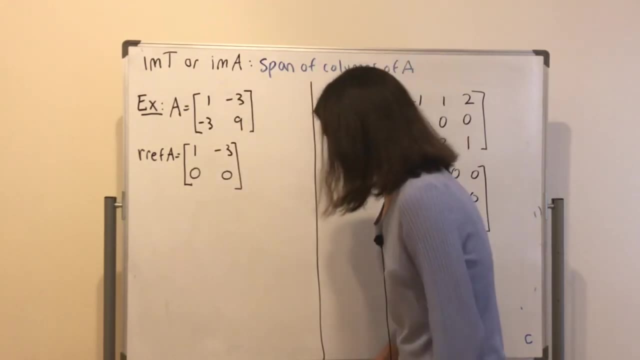 image. but I'm going back to both of these examples, where we found the kernel And we already have both the reduced row- echelon forms. Why do I have the reduced row echelon forms when I'm talking about the span of the columns? Well, I'll talk about that. 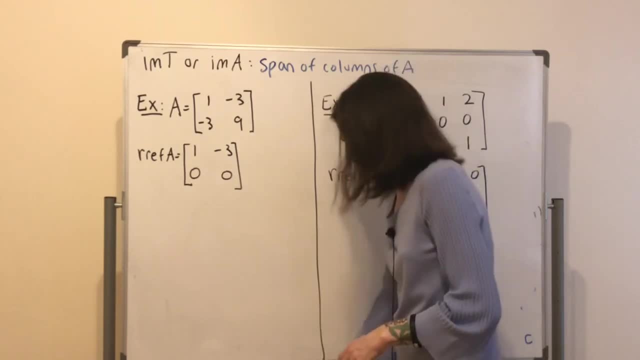 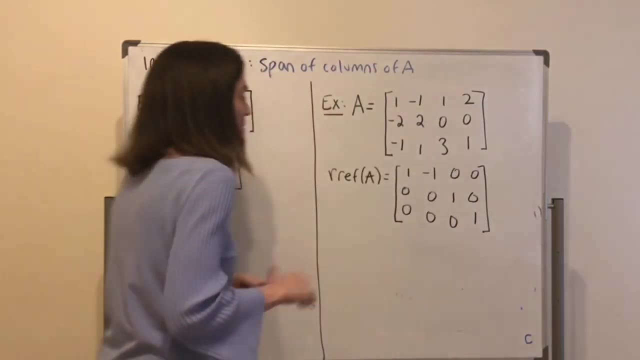 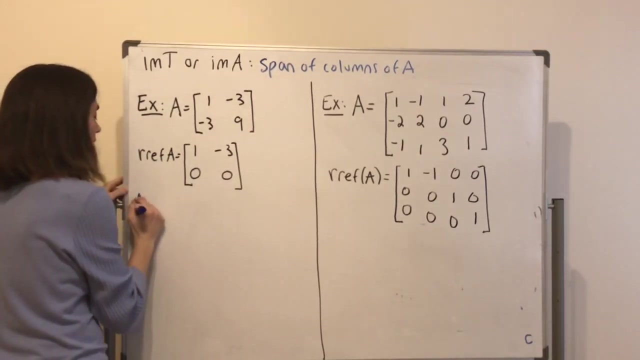 in a minute, Okay. Well, let's start with the easier. I guess it's easier. it's only 2x2, it's a warm-up example from before, If you take and multiply this by an xy. so here, if I take Axy, 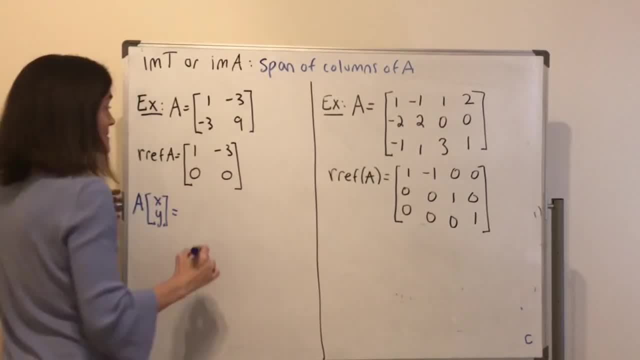 Linear combination of columns right, This is going to be x times 1 minus 3 plus y minus 3, 9.. And I can write this as the following: I can write this notice as x minus 3y all. 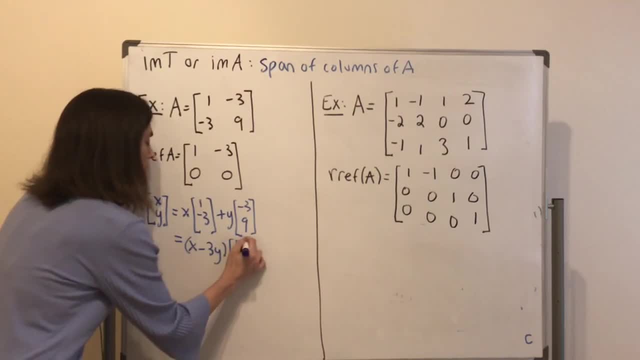 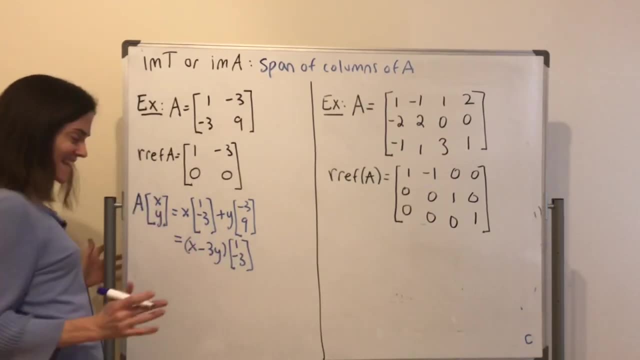 times 1 minus 3.. Right, because while this column is a multiple of this column, We see that, if you know, I don't need both of these vectors to represent the span of the columns, because any linear combination of these two vectors can be written as a multiple of just the first. Okay, So, 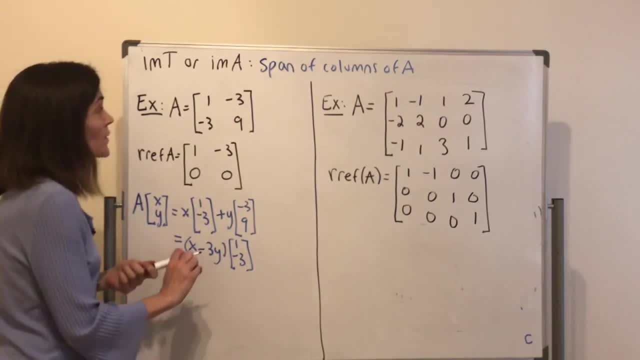 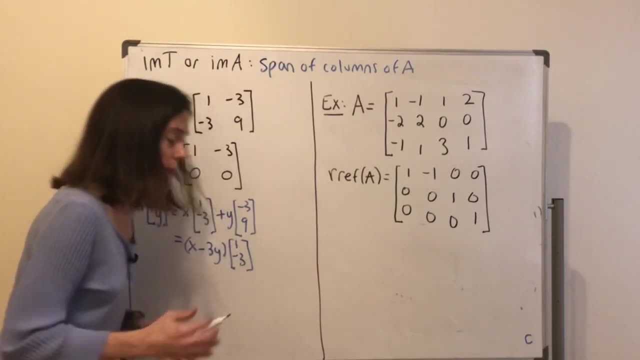 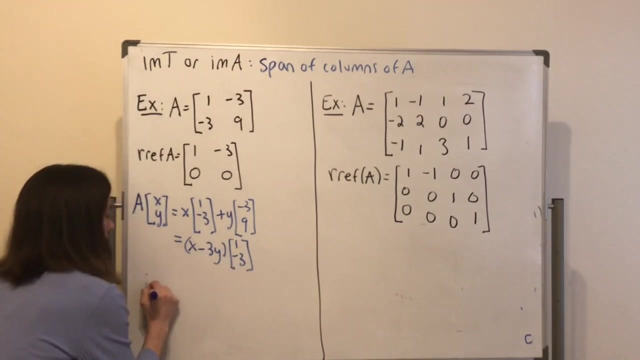 here the span. if we want to find sort of the smallest set- that's going to be the smallest set of vectors so that if we take the span we get the image of the matrix- All we would need is this one. so I will write that here. The image of A is the span of. we can represent it with just this. 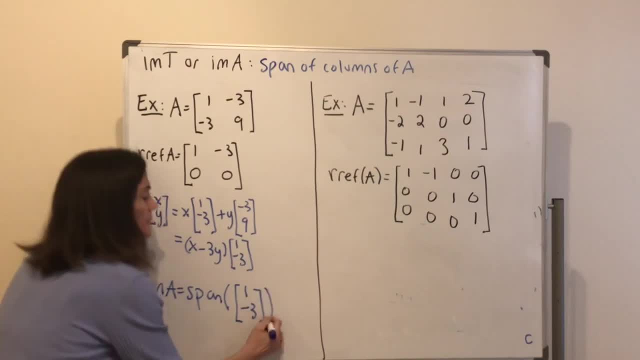 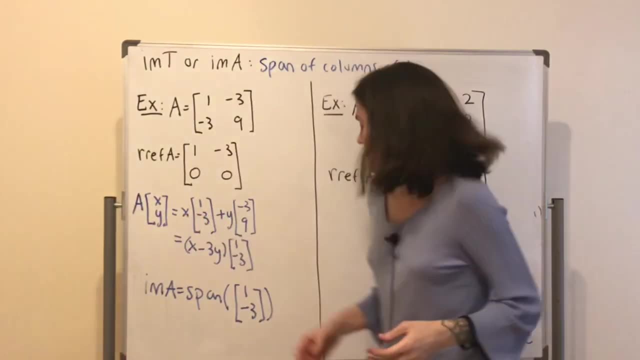 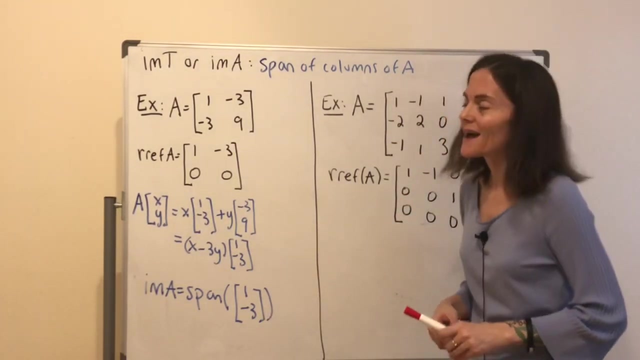 one vector, 1 minus 3.. Okay Now, how does the reduced row echelon form come in this? What you notice is the vector, at least the one that I chose to put here, and I could have equally have put 3,, 9,, but I'm about to go to one that's more complicated. is this vector or this column? 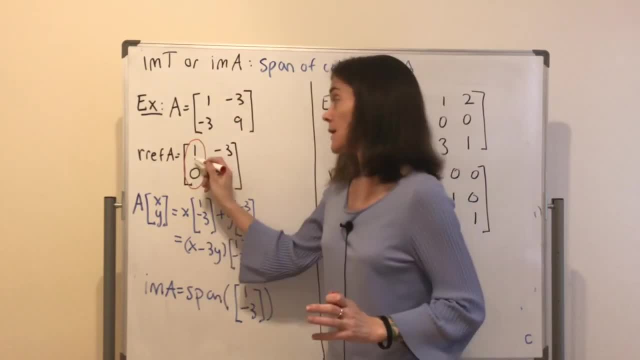 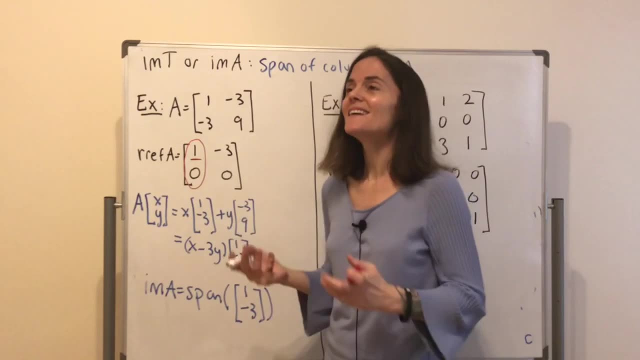 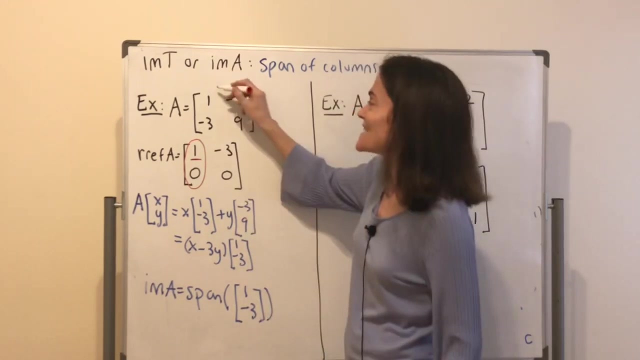 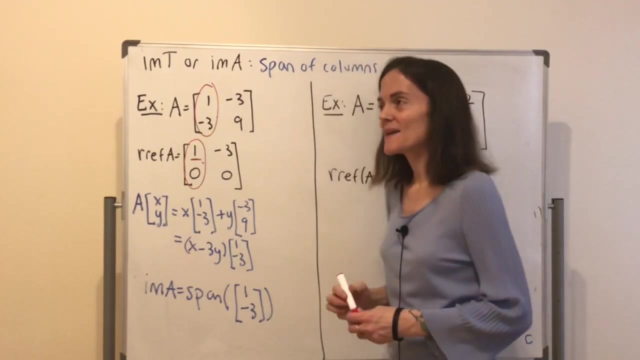 excuse me, is the column that has a leading 1.. And so when I write the image or the vector I chose to put as in in this set, to take the span of, I chose the one corresponding to the column that had a leading 1, and that was not by accident. 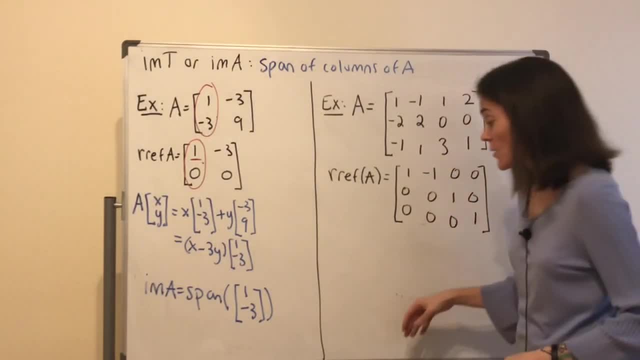 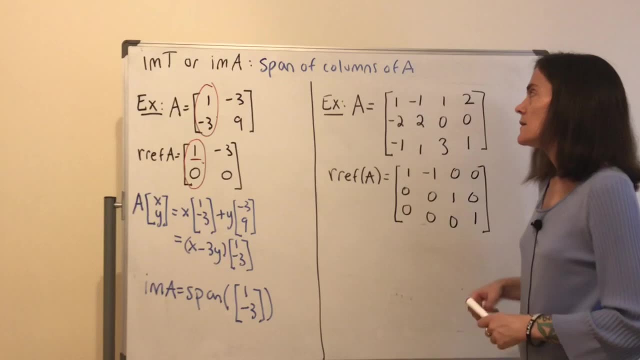 So how are we going to find, if we do the same thing here? we want to find, like the smallest we can, collection of vectors that span or that that that give the image right. So if you took their span, you would have the image of A. Well, you look here. this is how. we go about it. So if you took the image of A, you would have the image of A and you would have the image of A. So if you took the image of A, you would have the image of A. So if you took the 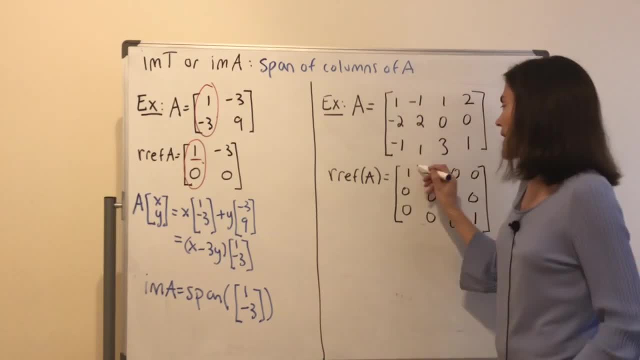 the image of A, you would have the image of A. So if you took the image of A, you would have the image of A. Look in the reduced real echelon form, such as this one here. This column has a pivot, or a leading 1.. This column leading 1, this column leading 1.. 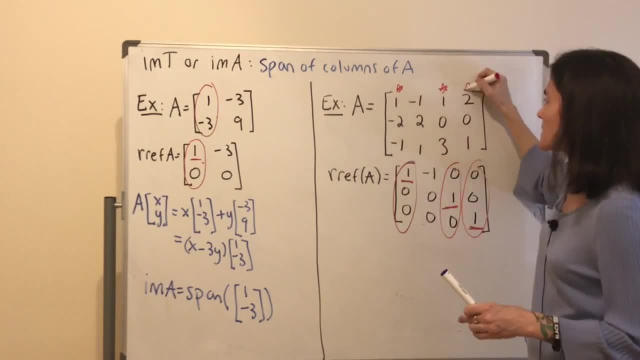 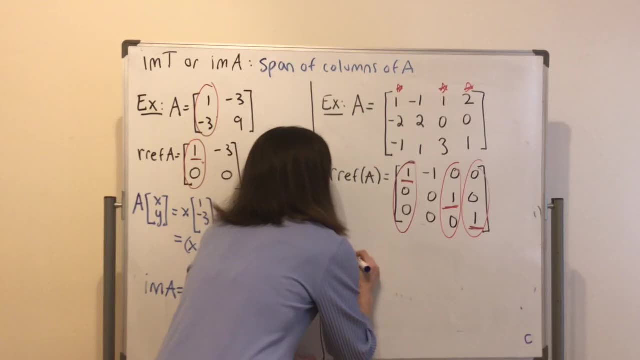 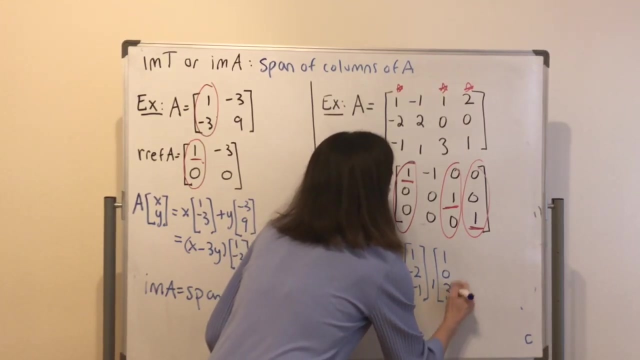 So I would take this one, this one and this one. Okay, The image of A. here is the span 1 of: okay, 1 minus 2 minus 1.. Then I have this vector: 1, 0, 3.. 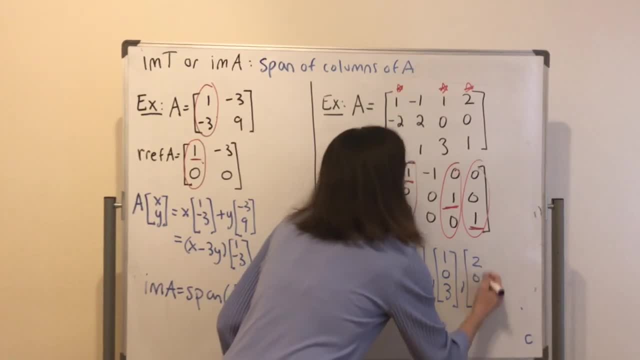 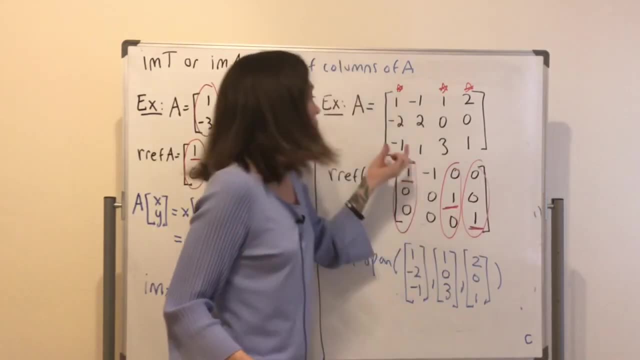 Then I have this vector 2,, 0, 1.. It's also true that the image of A is the span of all four of these vectors, But this one is well. it's redundant to add it to the list, okay. 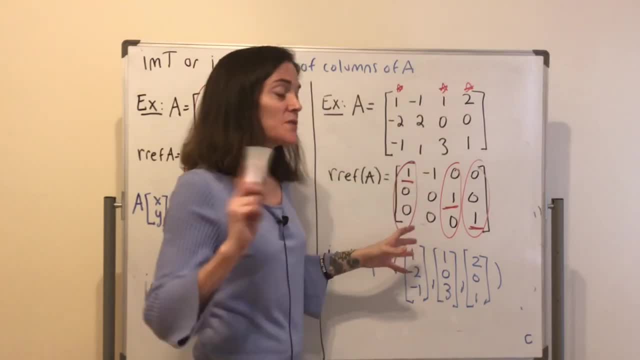 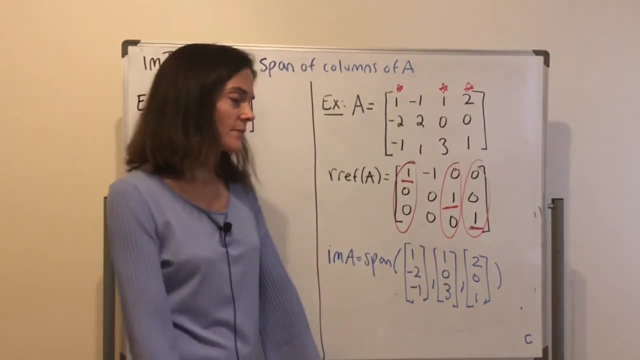 because we don't see, we don't have a pivot here, And this is something that we're going to get a lot more into in the next video. In fact, it's really the this idea, I should say, is really the focus of the next lesson. 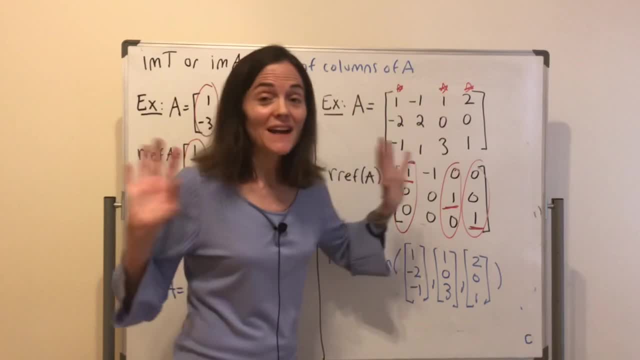 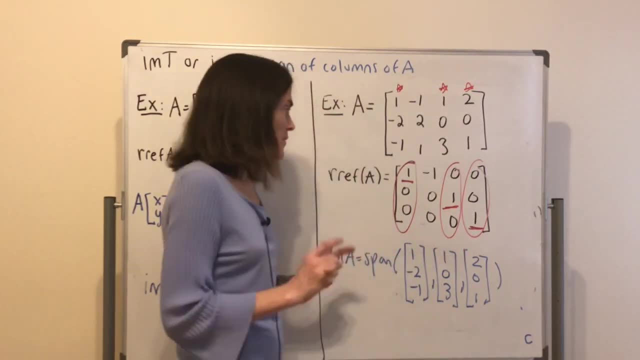 But for now this is. you know, we want to find the reducible echelon form of the matrix, Whether you're looking at kernel or you're looking at image, and then, when you're trying to find the image, you pull off the columns of your original matrix. 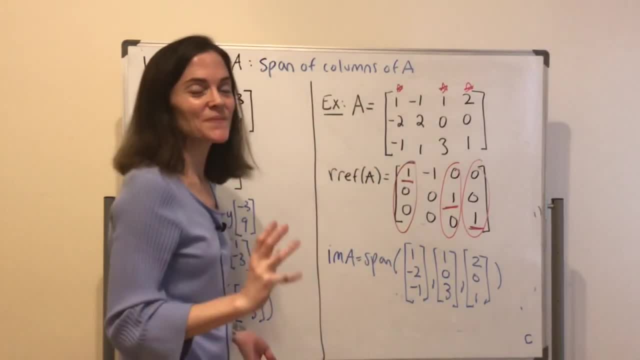 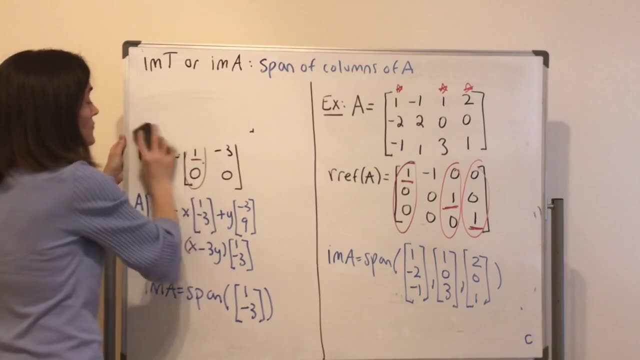 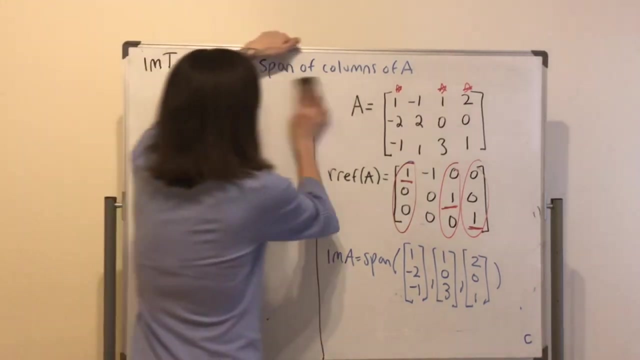 that correspond to the column, So the leading ones in the reduced row, echelon form. But let me show you how. before I do anything else, it's very important that you do just as I said, okay, So let's do the careful type of example. 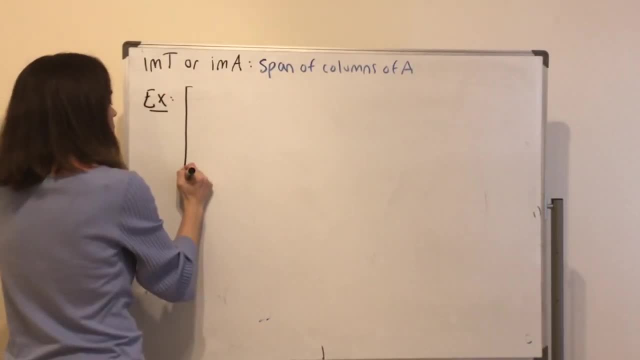 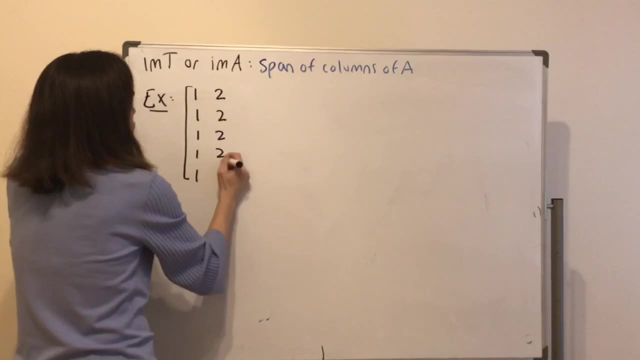 Let's look at this example: 1, 1, 1, 1, 1.. Okay, 2, 2,, 2, 2.. I don't know: 7, 7,, 7,, 7, 7.. 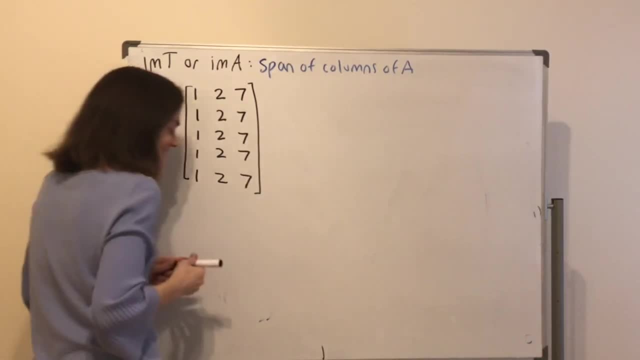 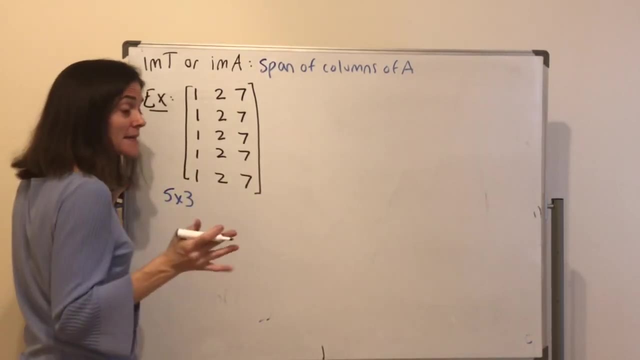 Okay, that's enough. This matrix is: we have 5 rows, 3 columns. Our image will be inside of our 5, right, You take a linear combination of the columns. Very nice. Well, let's start performing. 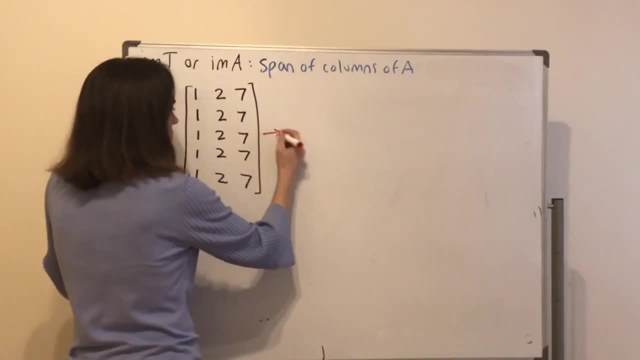 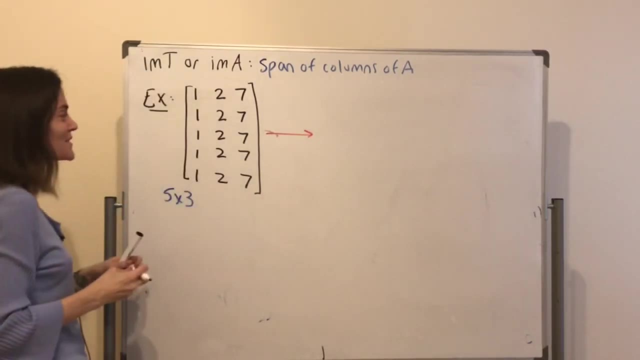 Okay, This is also going to be Wednesday. It's going to be super quick to get this matrix in reduced row echelon form. All I'm going to do. do I even need to write it? Oh goodness, This is what I get for putting so many rows. 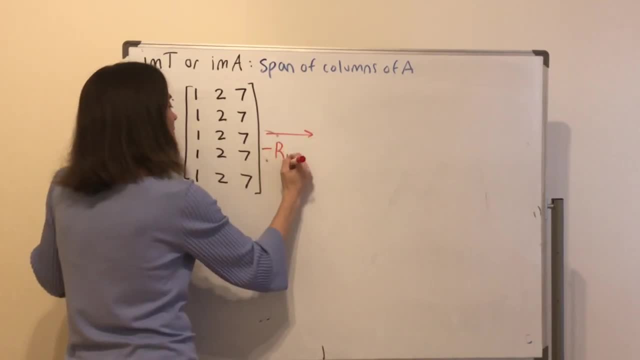 I'm going to take minus row 1 and add it to. I'm just going to put row I where I goes from. let's see 2, 3,, 4, 5.. Okay, And because it's the exact same thing. 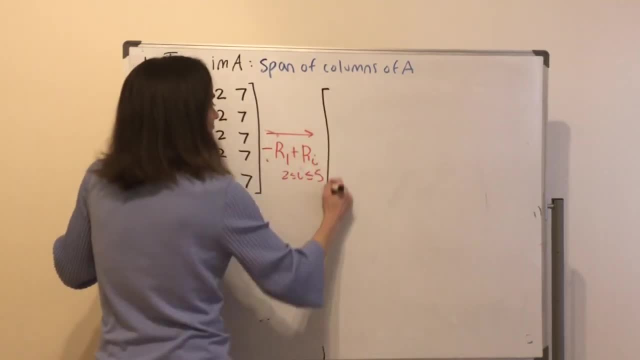 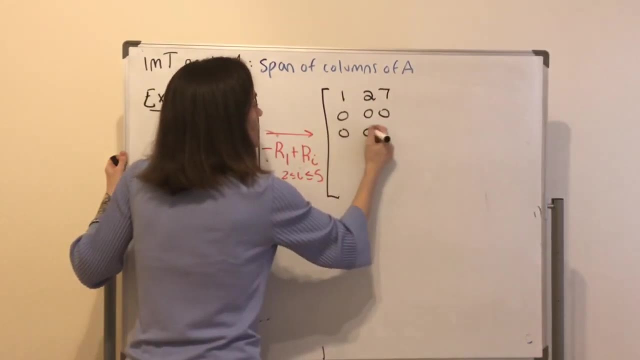 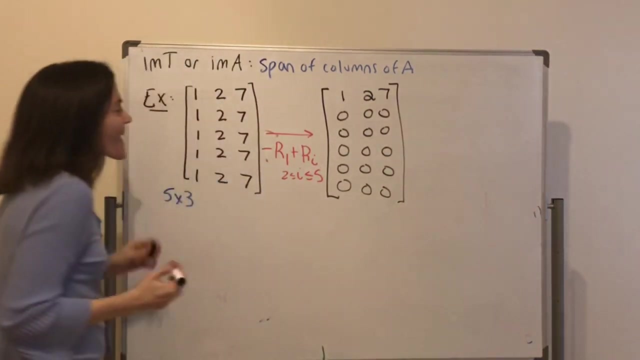 I'm going to do every single row And we get the following: 1,, 2,, 7, then we get 1,, 2,, 3,, 4 rows of 0s. Okay, Well, okay, very nice. 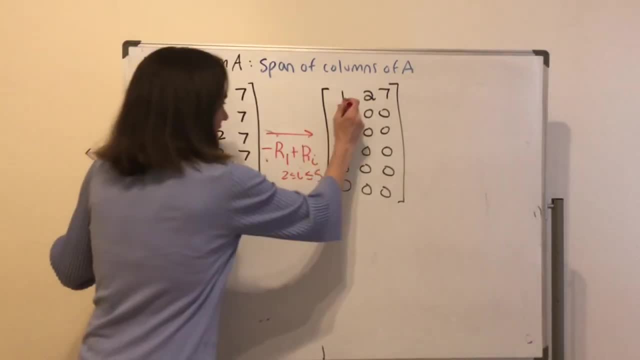 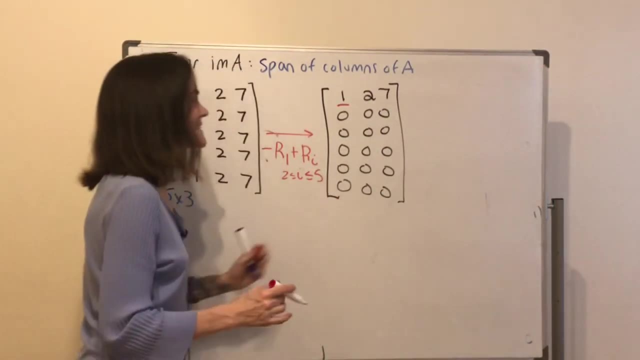 Before we go, as we did in the last two examples, we look here. This is my only leading one. In fact, well, before I say anything, we're going to reduce row echelon form here. Right, I have one leading one that corresponds to the first column. 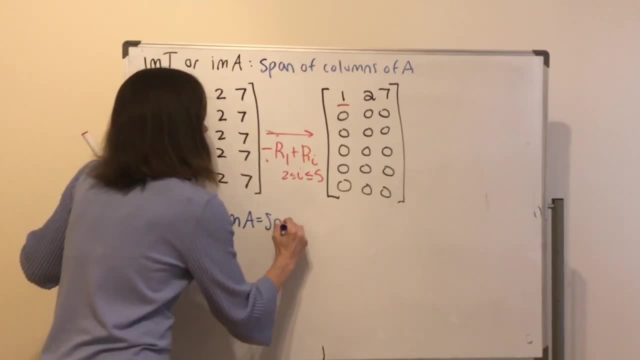 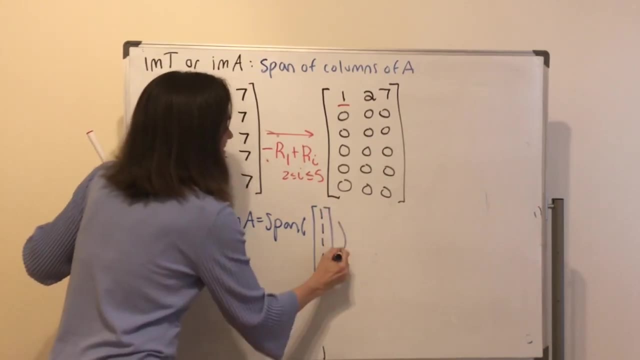 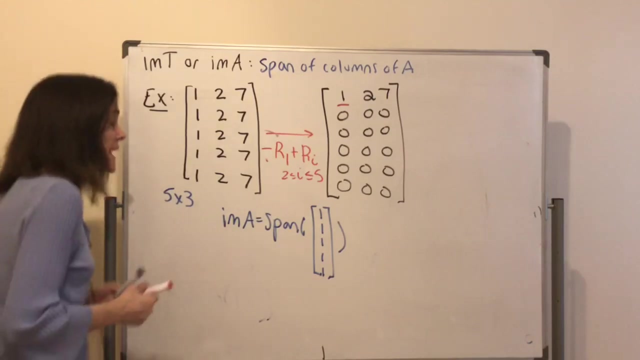 And so the image of A is the span of 1,, 2,, 3,, 4, 5, with 1s like this: Okay, perfect, Great. However, be careful. This is my caution. And when I said, do just like, I say, be careful. 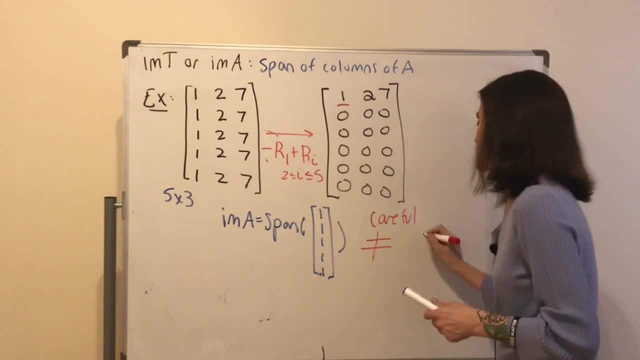 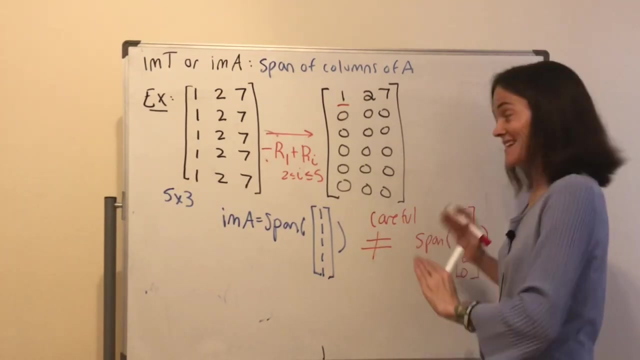 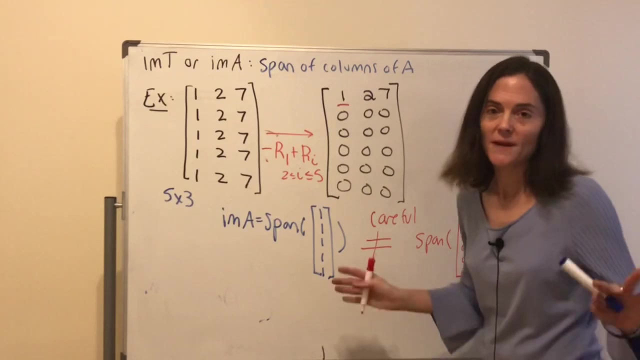 Because this is definitely not equal to the span where we just take the first column in the reduced row echelon form. These are, without a doubt, different, Right, They're not the same: The span of this one vector, every single vector in the span, has the same entry all the way down the diagonal. 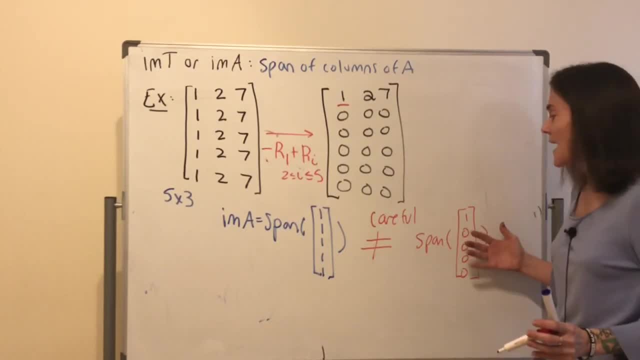 Every single vector in this span. well, if you think about it in R5, it lives in the just along the line x-axis, where x is something, everything else is zero. Okay, these are not the same. So you do not want to find the reduced row echelon form and then pull off the columns of the reduced row echelon form where they have leading ones. 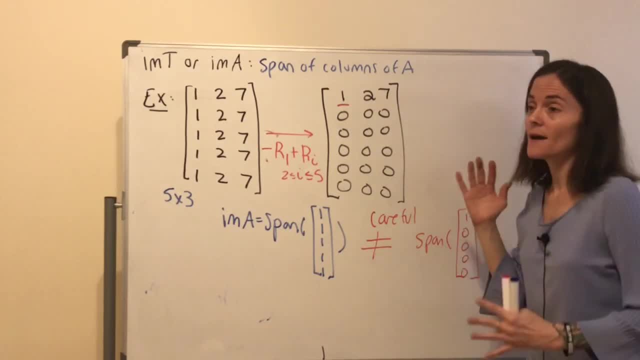 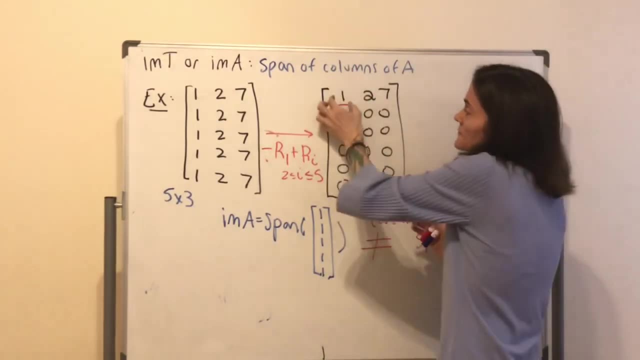 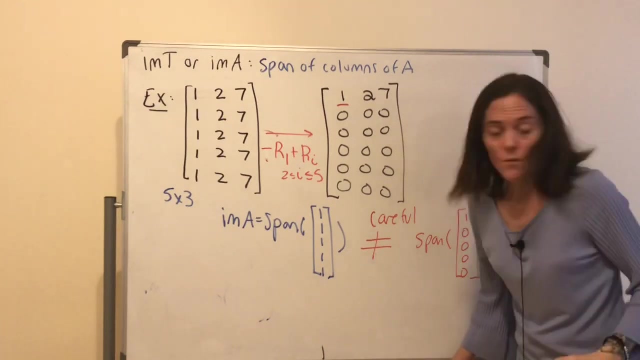 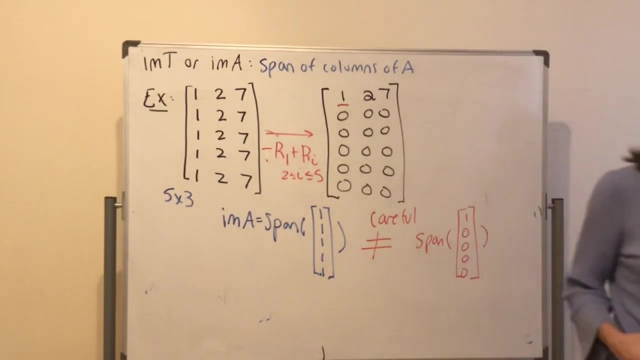 This would not give you the right, the right image. We see it here. So that was my word of caution. If you reduce to find where the leading ones are, then you pull those columns out of the original matrix. Okay, I think what would be nice is, let's do one more example where we find both the image and the kernel. 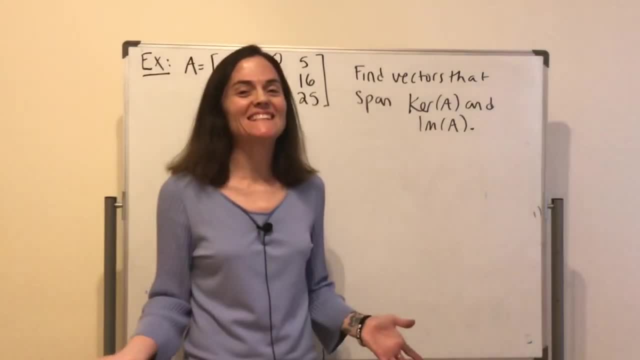 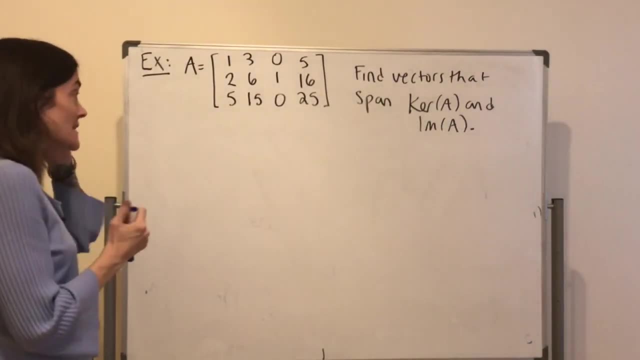 Here's my last example. Then I'm going to make one or two comments And then we will be about done for the day. So here is a. We have a three by four Matrix And we're going to do both things. 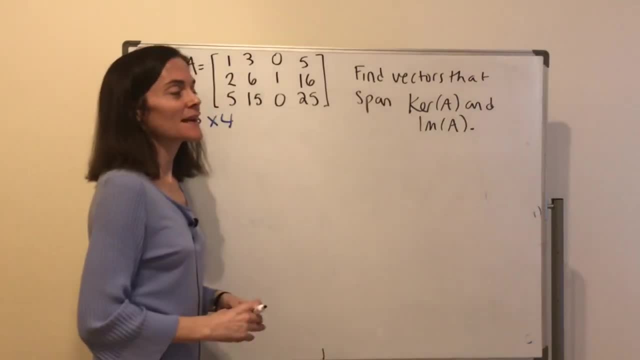 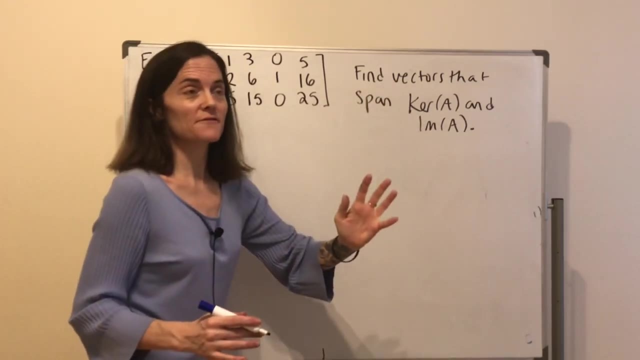 So we discussed kernel, We discussed image, And we will find vectors that span them both. In both of these, I need to find the reduced row echelon form of A in order to solve the problem. So this is what I will do. first, 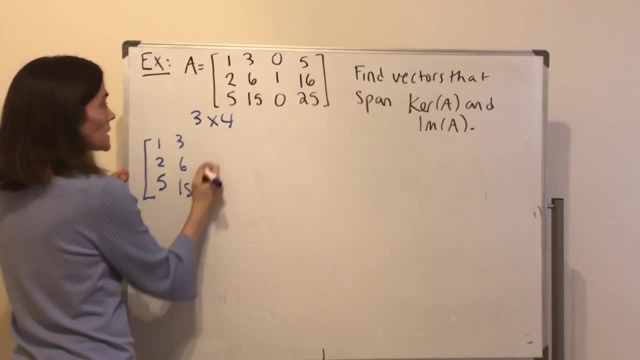 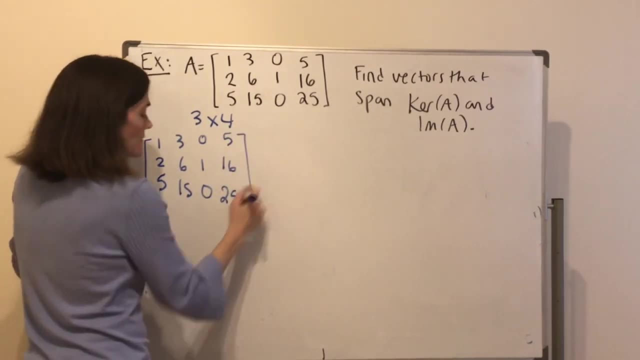 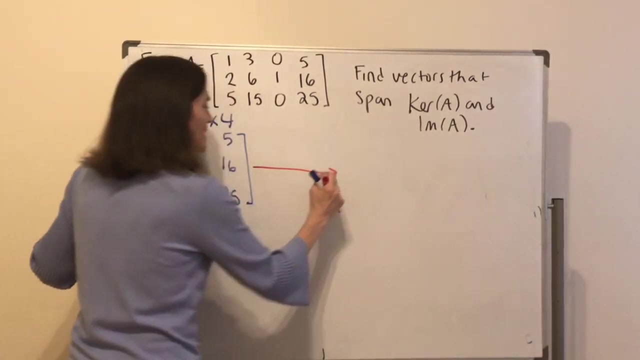 One, two, five, three, six, fifteen, And then This one is fortunately a Fast example in terms of the elementary row operations. I think we don't have too many to do to get it in reduced row echelon form. 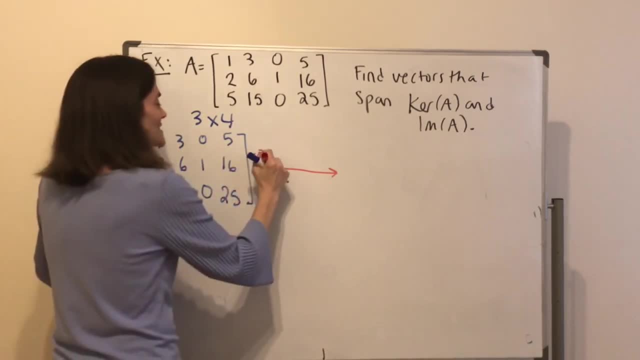 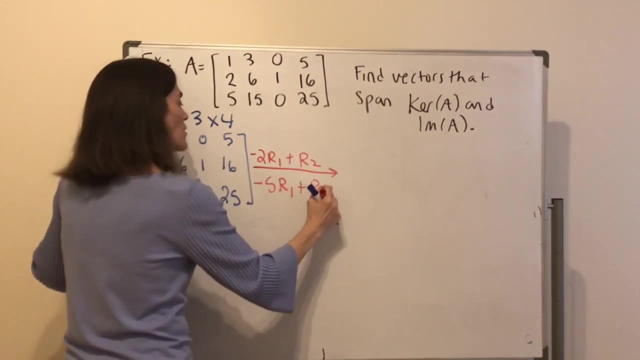 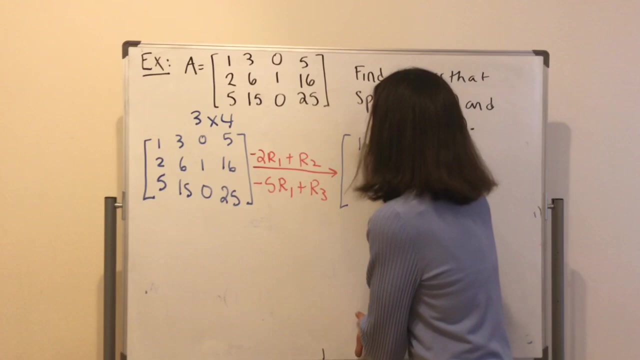 Well, okay, We're going to take minus two. row one, Add it to row two. I'm going to take minus five, row one, Add it to row three, And then let's see what we get. Row one: I have not changed. 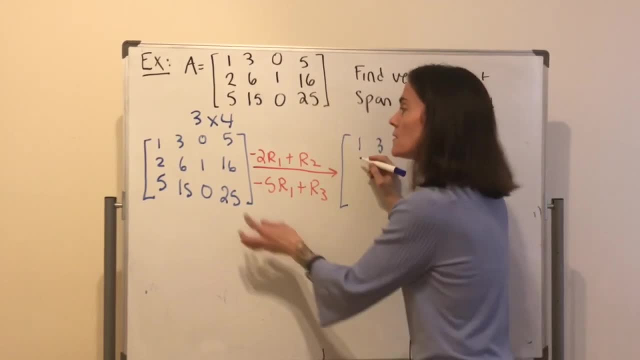 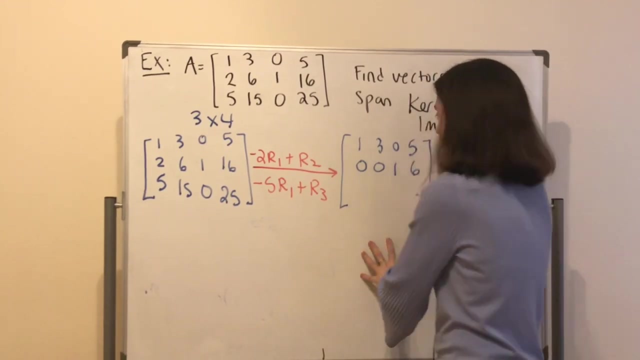 Row two: okay, good, Here this is zero, zero one. And then here this is going to be minus ten, And here is six. Okay, And then the last row: we take minus five times this. Add it here. 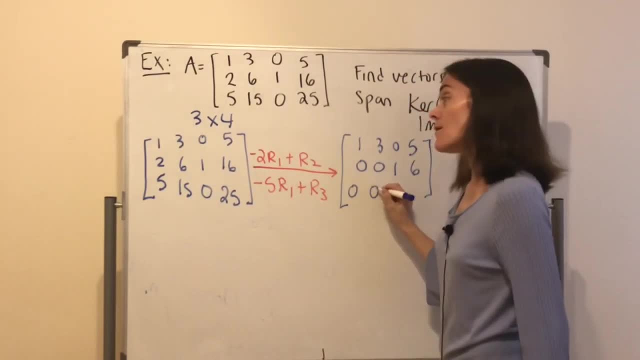 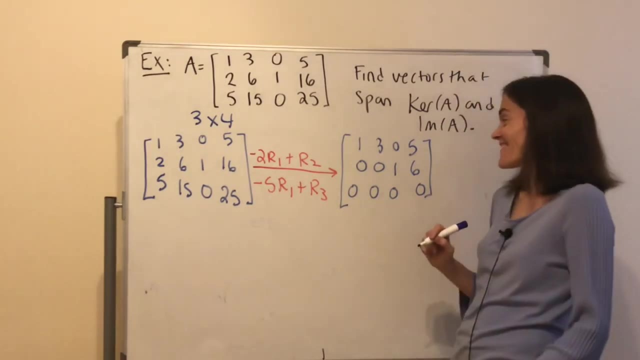 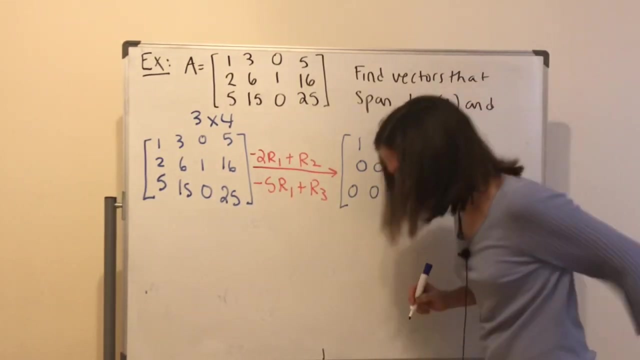 We're going to get zero, zero, zero And then minus five. Oh no, Okay, zero. See what I was saying. It's a very nice example, because it was just one step. Well, we did two things, but in one shot. look, we are in reduced row. echelon form. 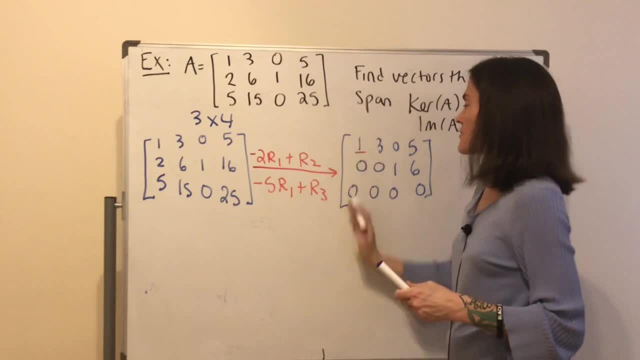 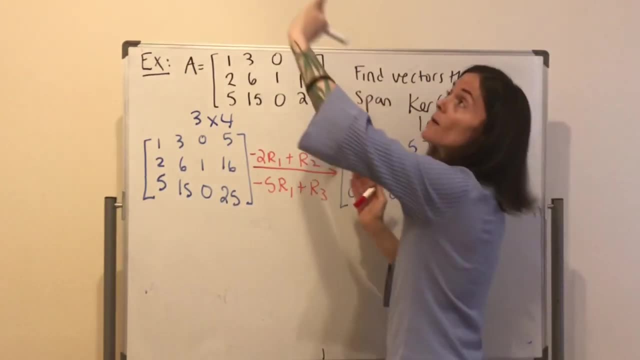 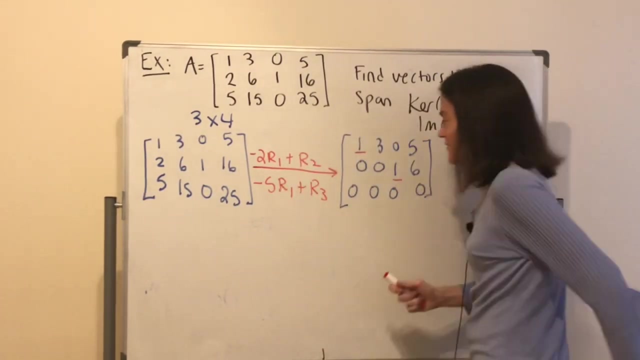 because here's a leading one. zeros above and below. here's a leading one. look up, look down, all you see is zeros. and then, for this leading one, every row above, you see there's a leading one, and it occurs to the left. Wonderful, Okay, we're in reduced row. echelon form. 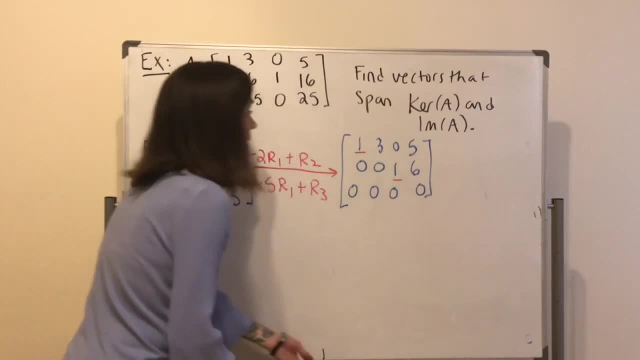 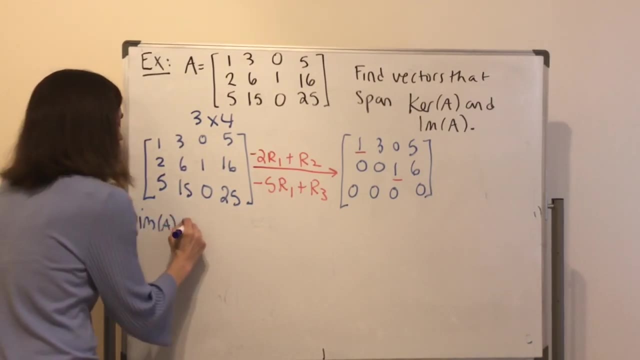 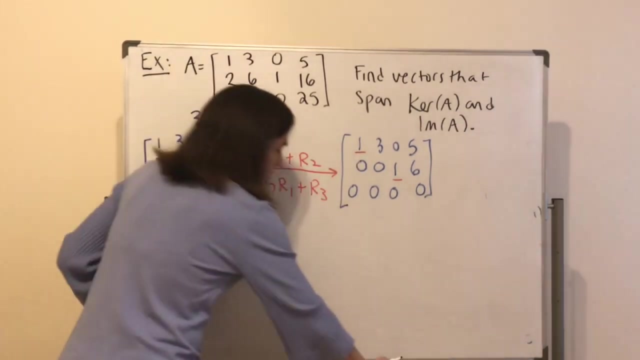 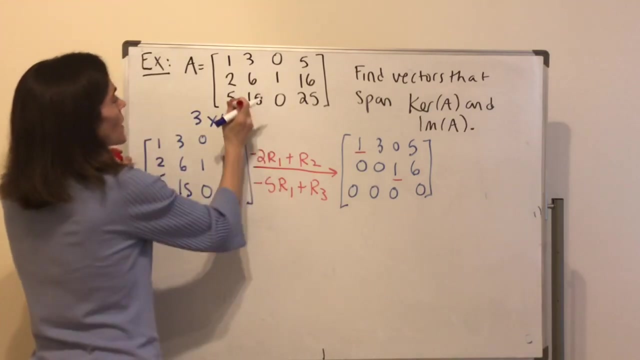 Which one do we want to do first? Well, maybe the fastest one is for the image. The image of A is the span. I look, okay, careful, don't pull it. uh, the columns out of here, but it's column one and column three. 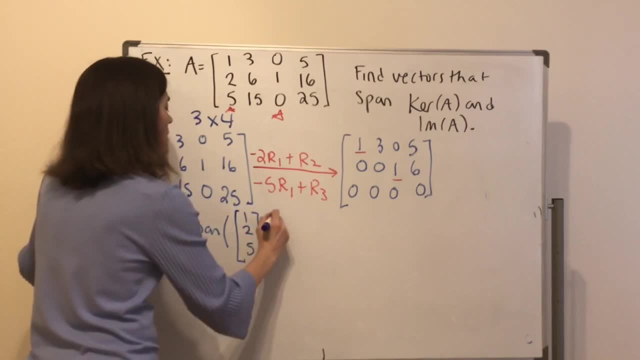 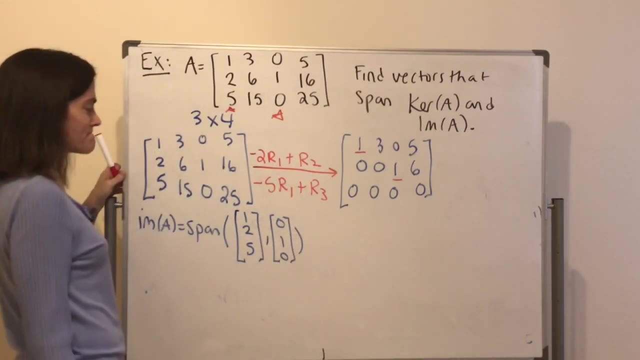 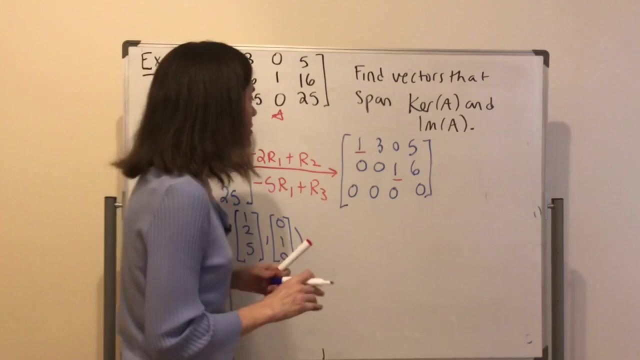 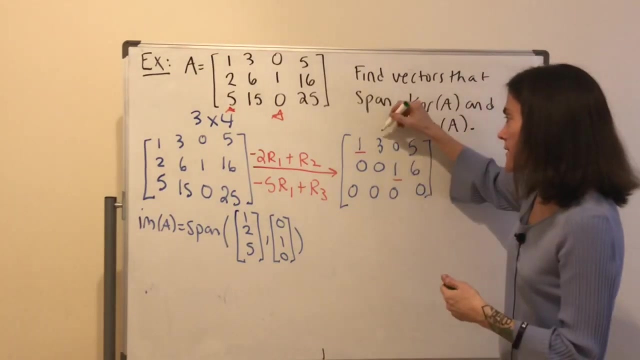 One, two, five and column three: Zero, one, zero. Okay, we have the image, or two vectors that span the image. Now for the kernel. well, now I have to think free variables. So my free variables are here and here. So let's start writing some things. 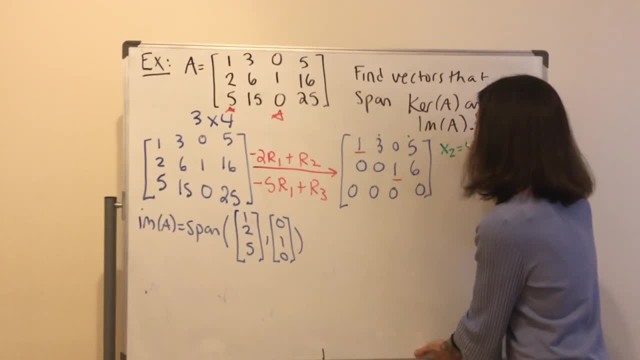 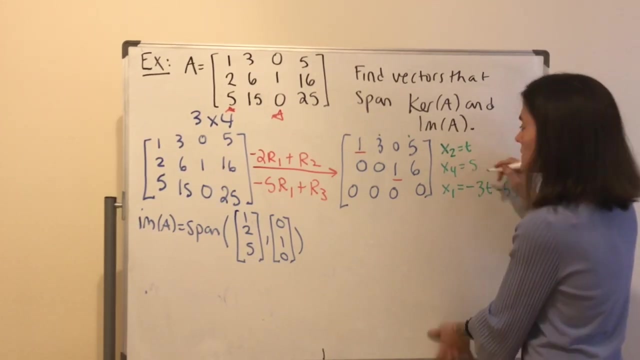 Let's say X2 is T and X4 is S, and then I have that X1 equals. well, if I write this, it's going to be minus three T and S minus 5s. this is an s from this first line. and then this is: x3 equals minus 6s. okay, 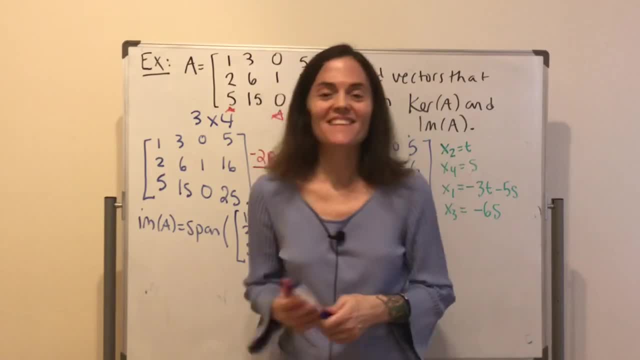 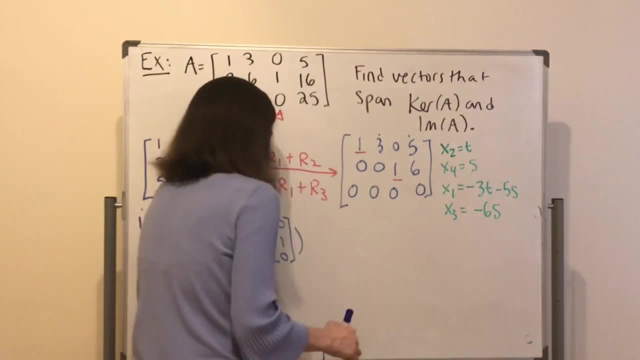 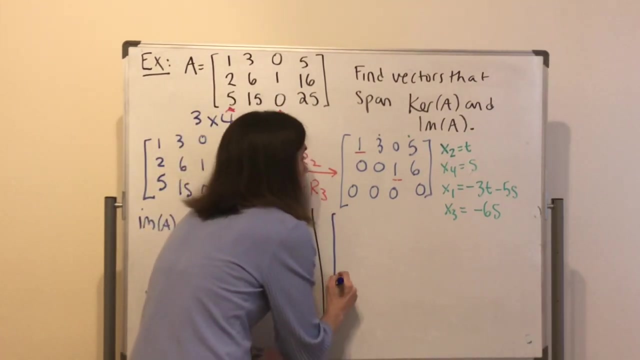 So now let's write the vector, then we will figure out the vectors. well, we'll finish the problem. vectors that will span the kernel. so now maybe I'm going to do a vertical like this: we get x2 is t, x4 is s, then we have minus 6s and we have minus 3t minus 5s. okay, 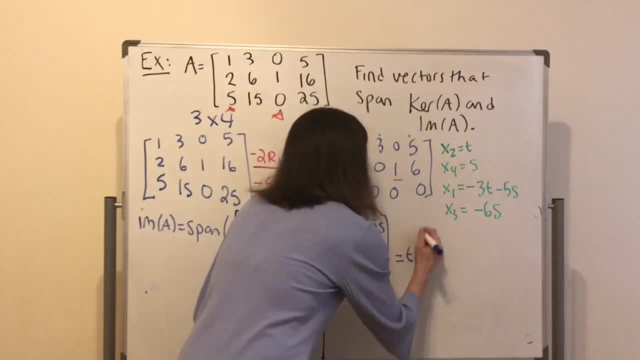 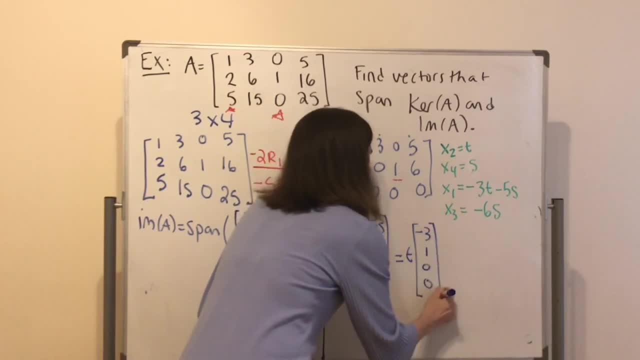 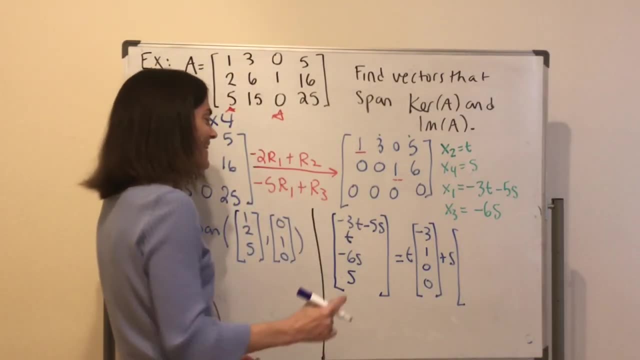 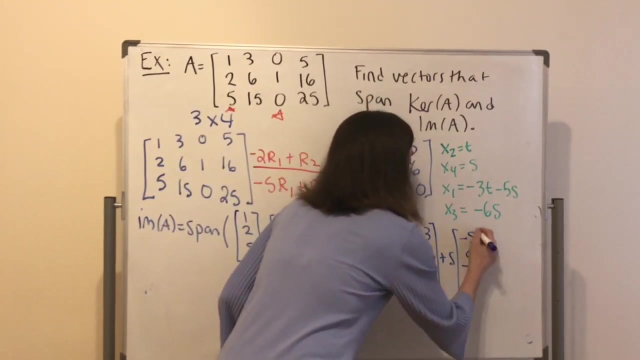 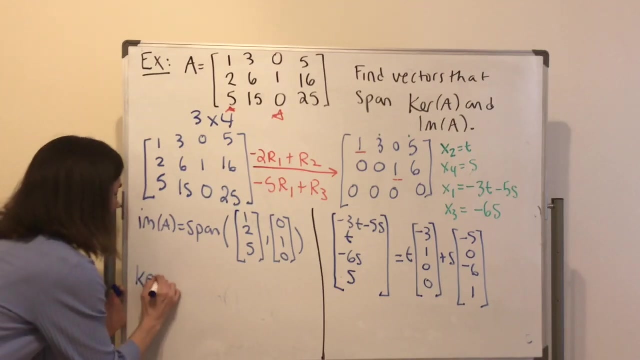 Minus 3, 1, 0, 0,. plus s times minus 5, 0, minus 6, 1,. minus 5, 0, minus 6, 1.. Okay now, ah, maybe I'll write it over here. the kernel of A is the span. 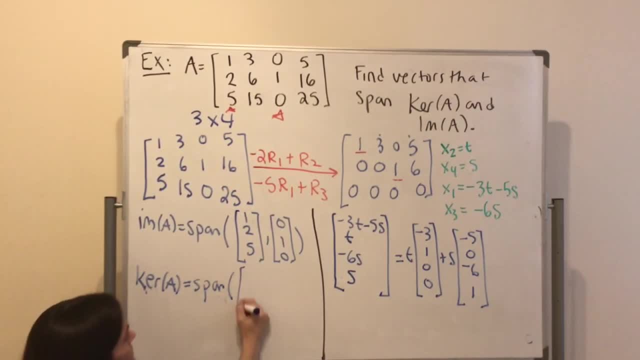 of. I have two vectors here, two minus 3, 1, 0, 0, and minus 5, 0, minus 6, 1,. okay, So here is. maybe now I'll put this in a black box. this is the two answers to our problem. 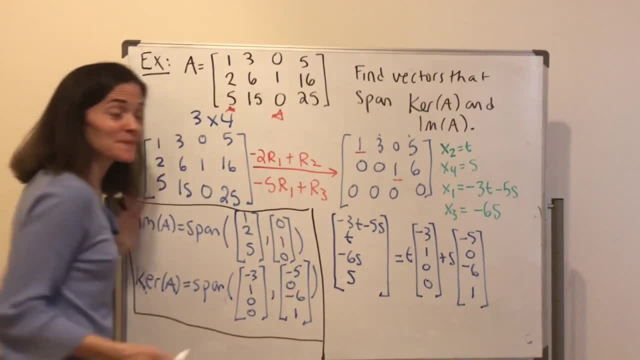 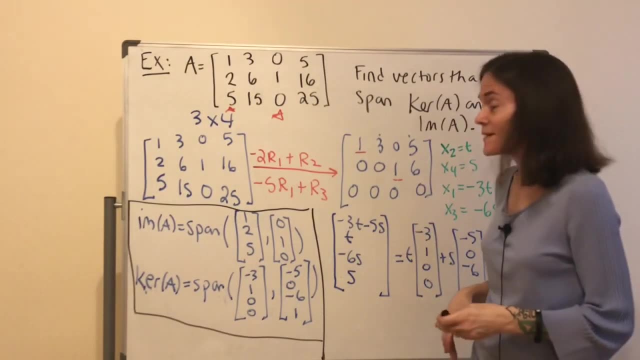 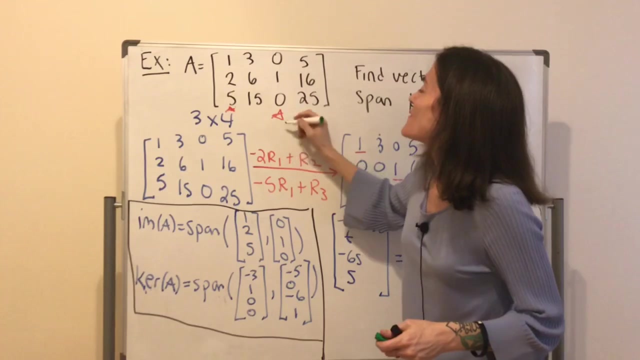 and let's make a couple of observations. Um, you notice, okay, I want to focus on numbers here. after all, this is a math class. Okay, well, you notice, we have four columns. you have four columns I'm going to erase. 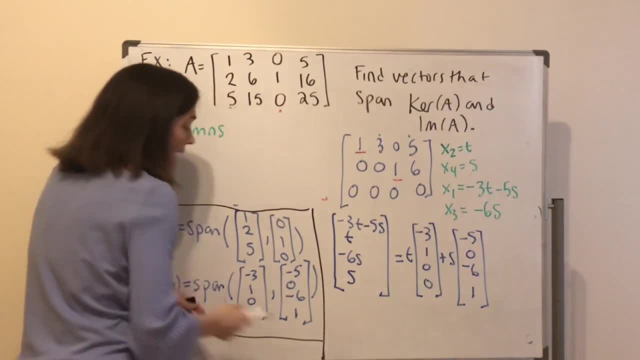 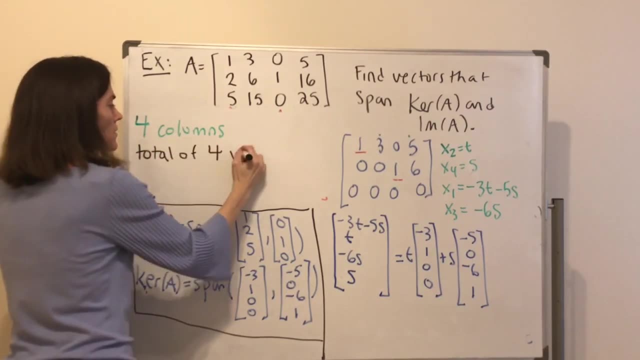 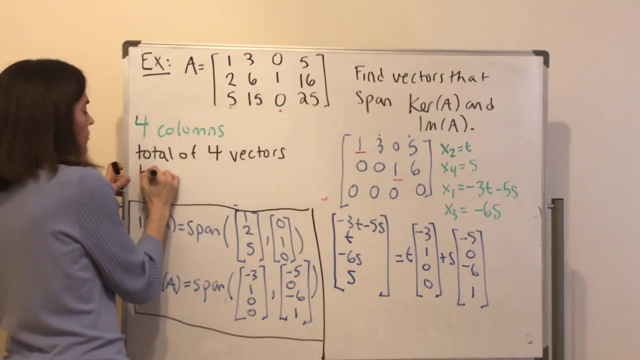 of my matrix. And if you add up all of them, all of these, we have a total of four vectors that in our answers I'll say below. And this is not by chance, because in the image two of them- the ones coming from the image- 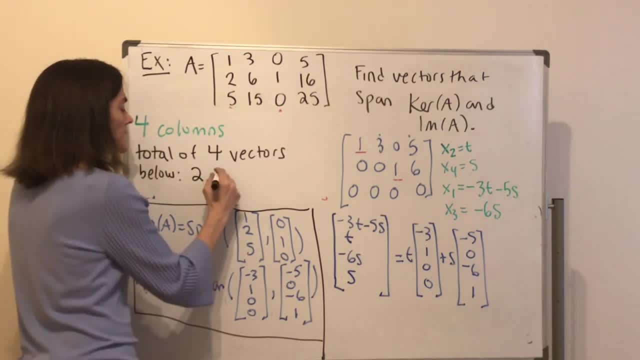 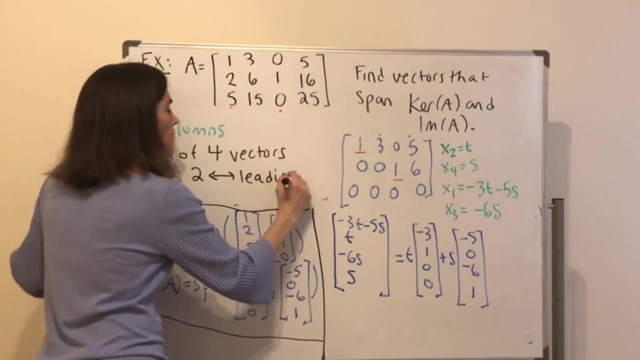 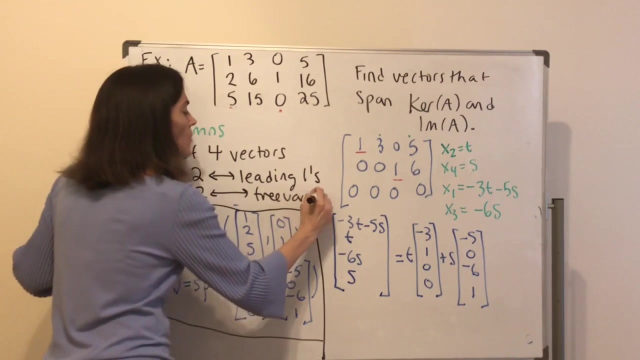 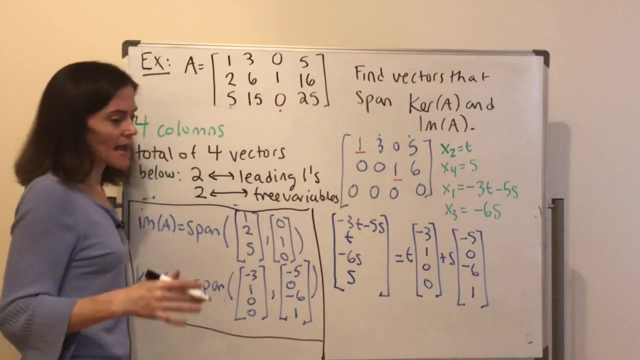 these corresponded to the leading ones And these the rest of them corresponded to the free variables, And so, of course, every single column, once you reduce to reduce row echelon form, is either going to have a leading one. 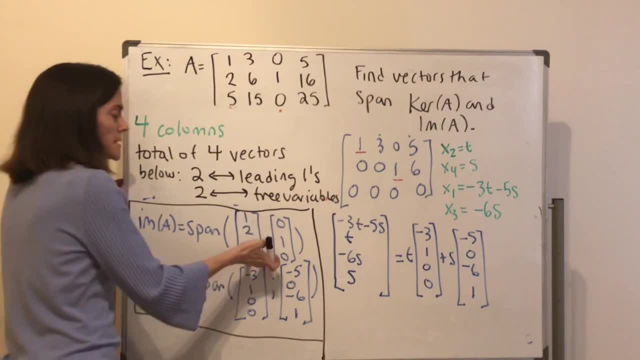 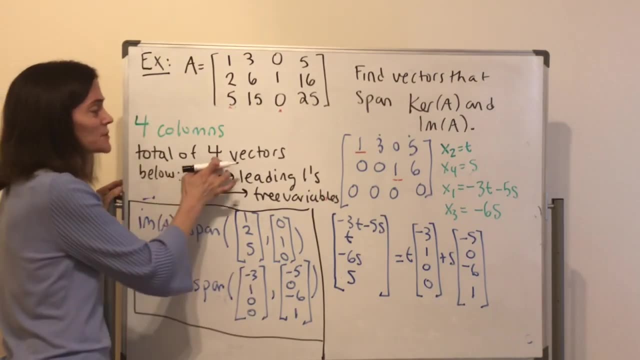 or be a free variable. So if we take this number which gives us the span of the image, this number which gives us the span of the kernel adds up to the number of columns of the matrix. Okay, this is like I said, this is not by chance. 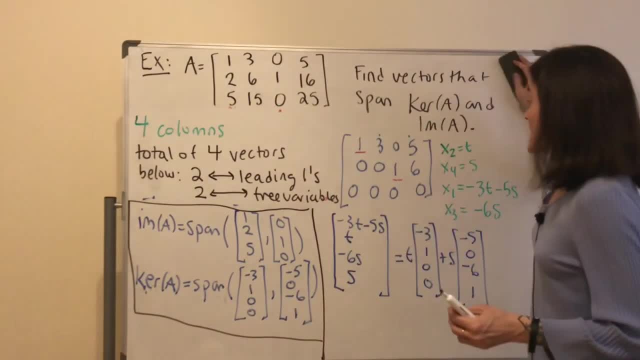 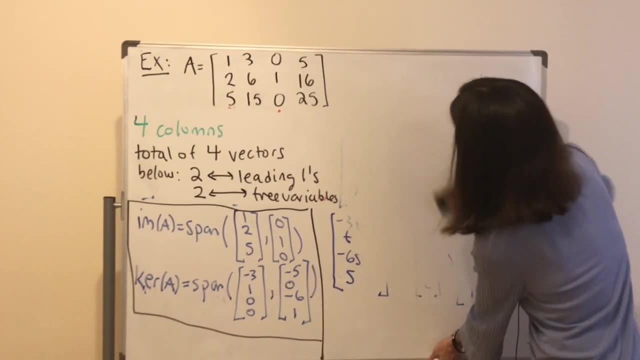 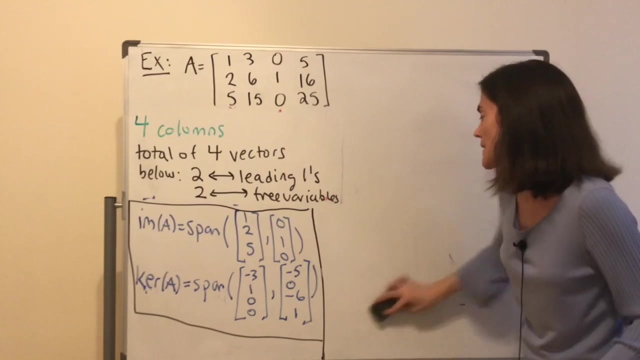 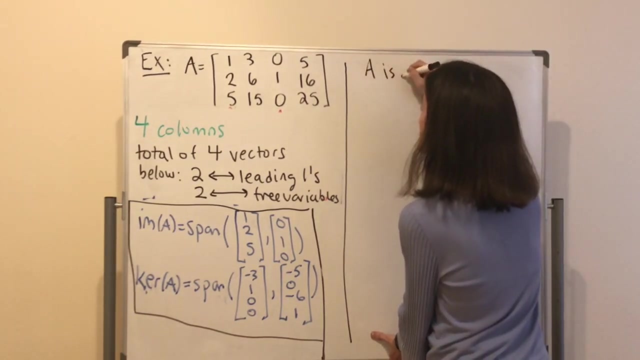 This always happens. One thing that comes out of this- and this will really be more natural once we get into the next section where we're discussing bases and linear independence and things like this- but one thing that comes out of this observation is suppose, now that we have A is n by n. okay, so then we know one characterization: A is 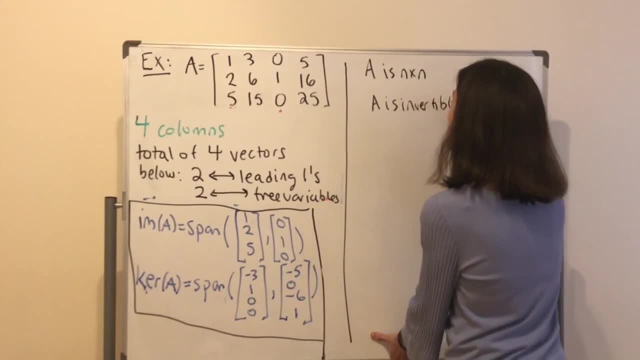 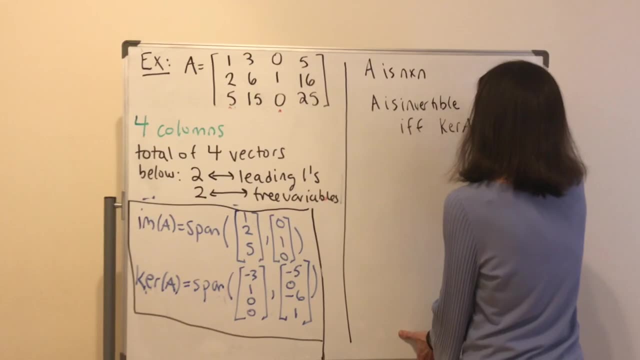 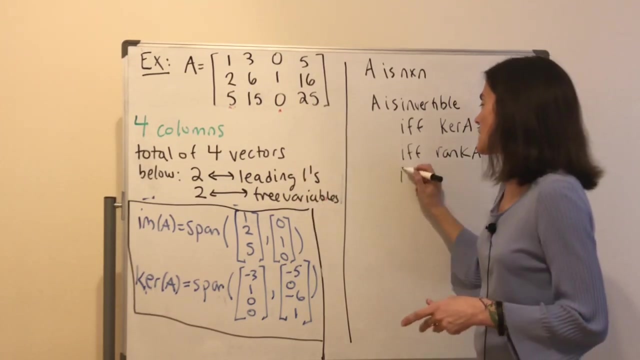 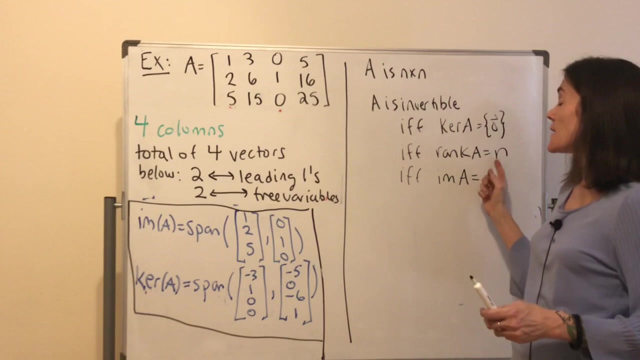 invertible if and only if. well, the kernel is zero. okay, this is the case if, and only if, the rank of a is n. well, if you think about this kind of thing, this would say if and only if. what about the image? well, here, the image, you would have the number of vectors in here that you have leading ones. 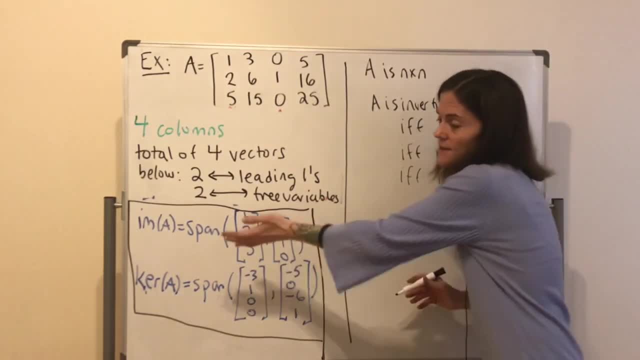 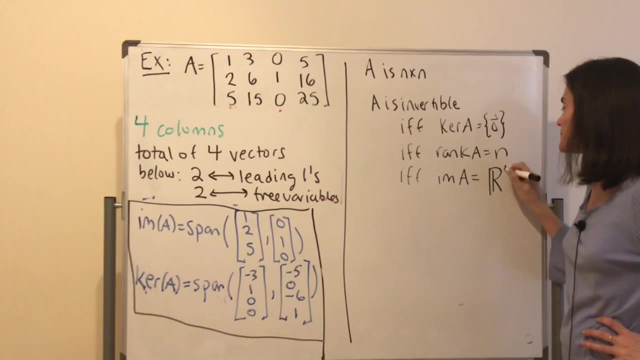 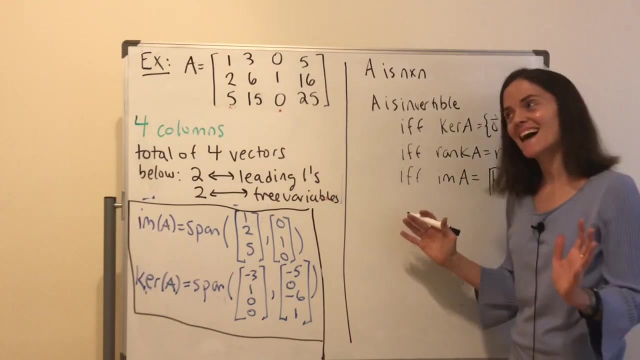 which is the rank. so you have n different vectors that all were sort of coming from leading ones. okay, so you will get this, and this goes back to my comment. well, this is two videos in a row. we're ending on the same comment. i kind of like that. my comment at the end of the last.